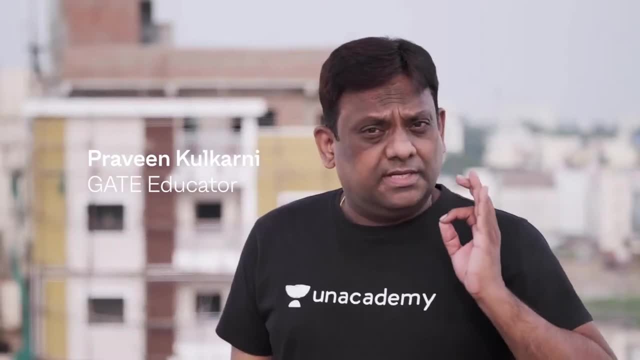 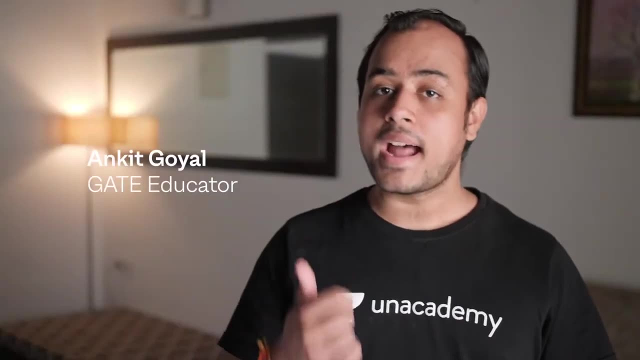 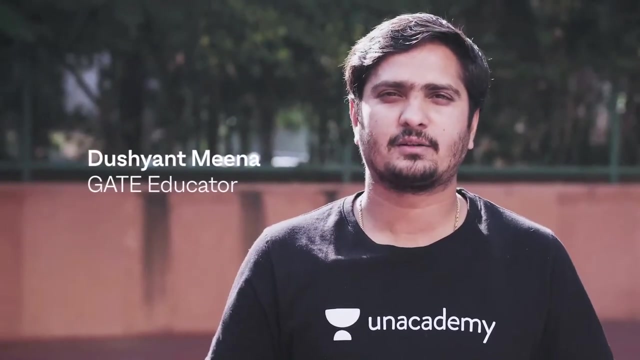 With the best of the questions by best educators, With detailed video solutions from top educators right after each contest. Combat live with peers to get real-time rankings and win big. Participate in every contest to improve your ratings, Challenging contests every fortnight or alternate Sunday. 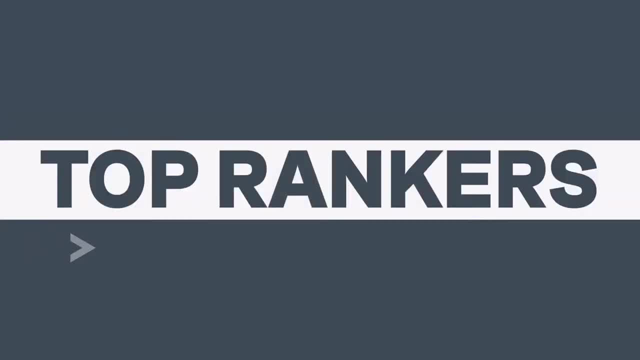 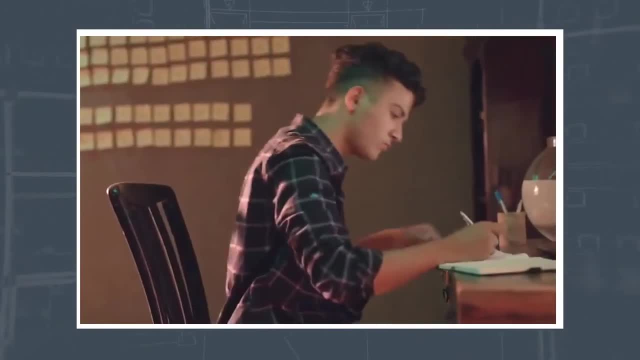 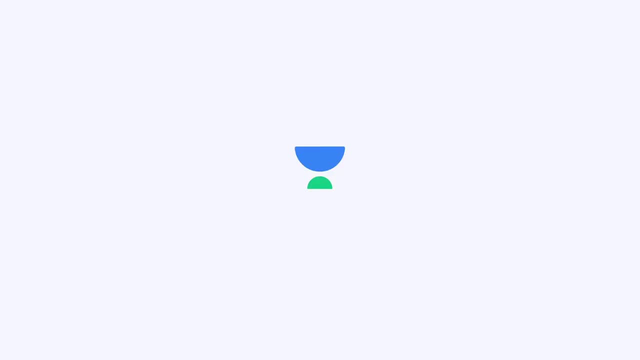 Live ranking after every question. Big rewards for top rankers. Your passion to crack GATE deserves this. Your hard work towards your dream deserves this. Fuel your inner fire for the ultimate GATE challenge. Unacademy Combat Register now wwwunacademycompetitioncom. 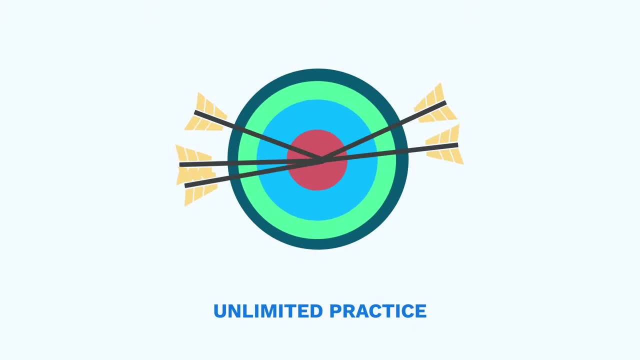 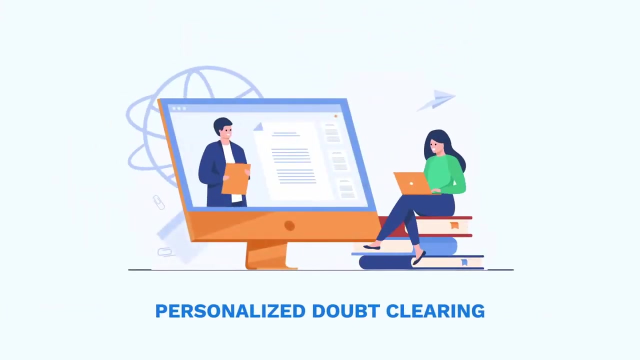 Seems like it's time to realize in the while zone. In fact, it was my dream And again, But still, Unless your GATE is a choice, The course is open up. ada respel k decompzza Unacademy Combat. 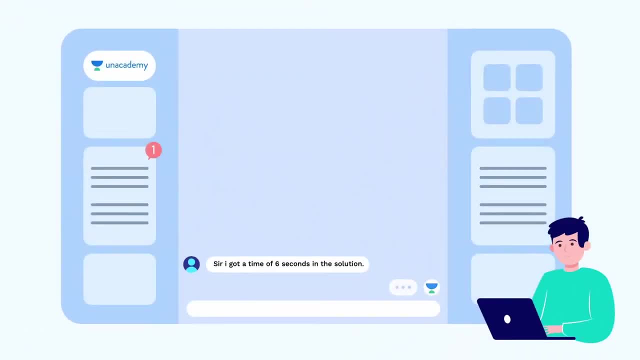 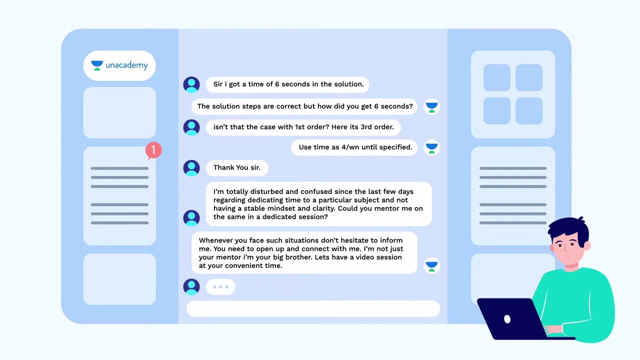 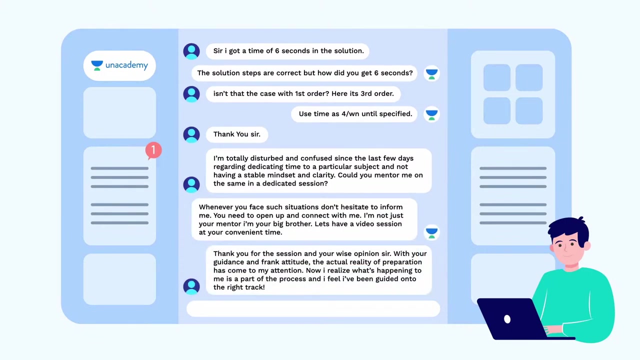 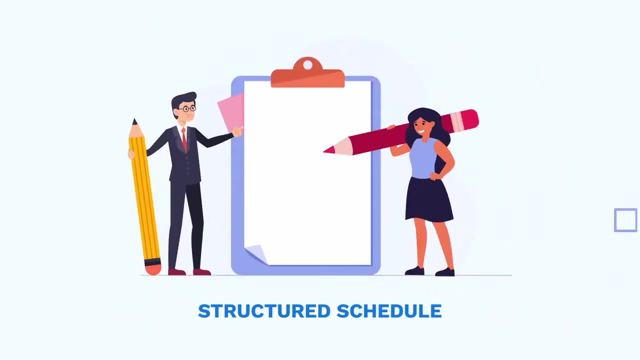 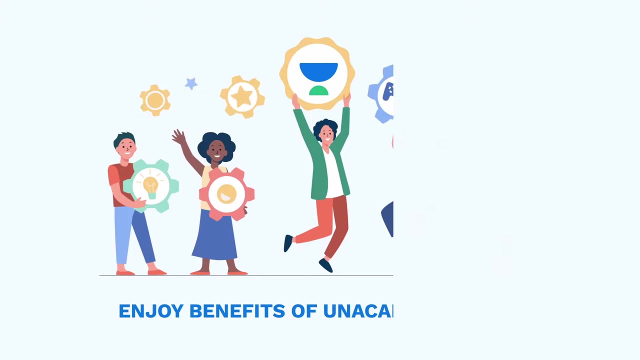 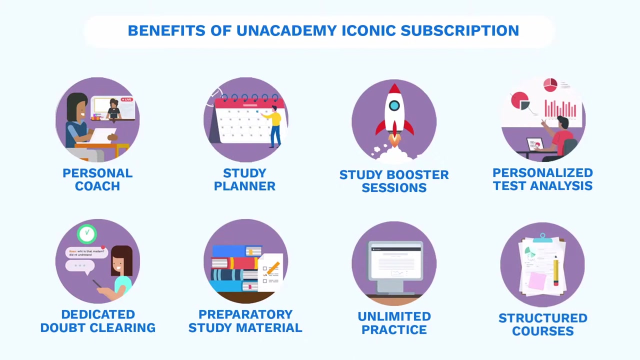 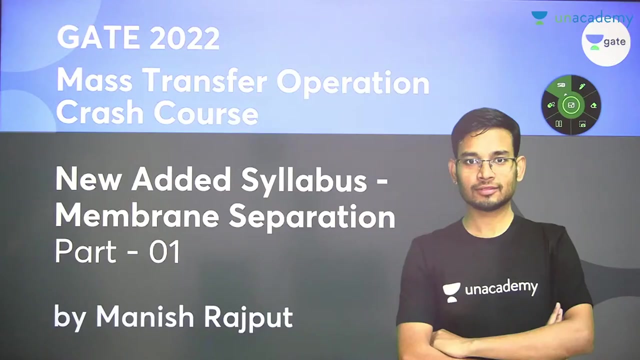 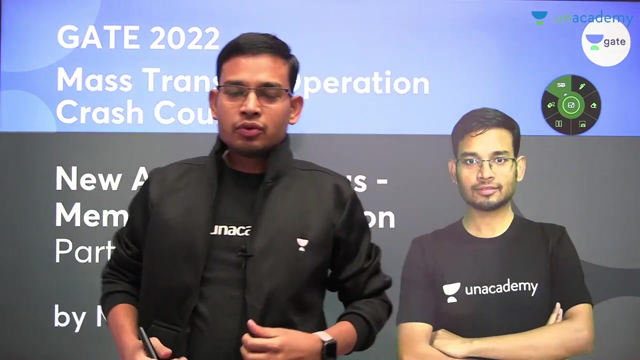 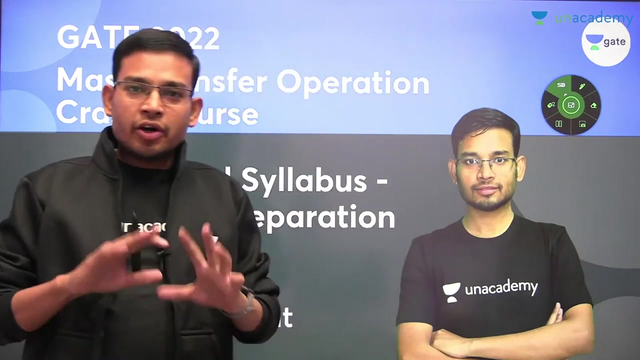 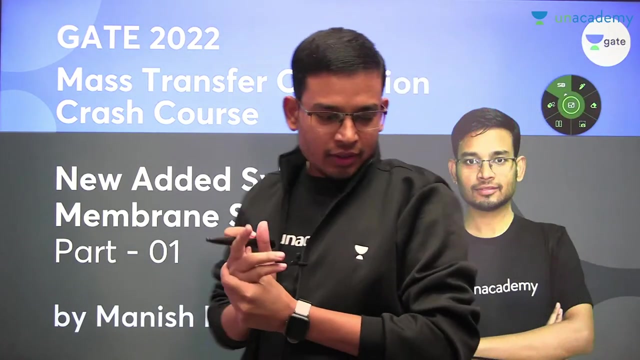 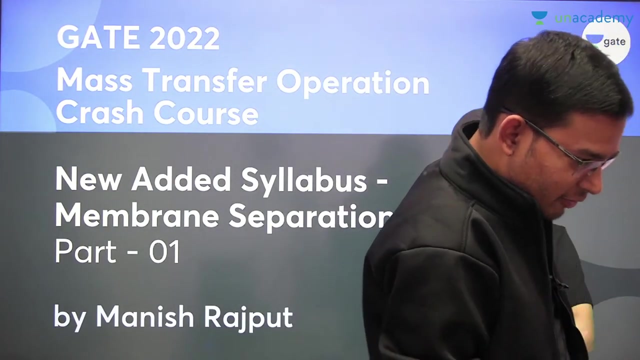 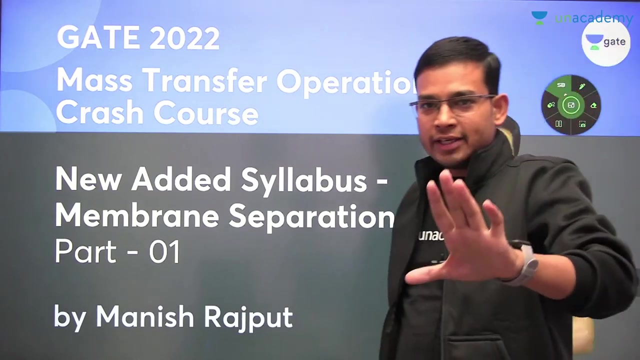 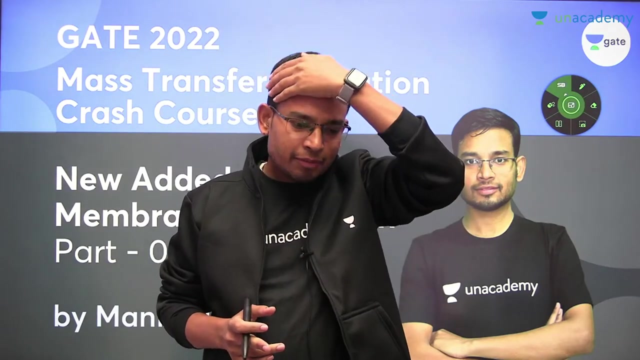 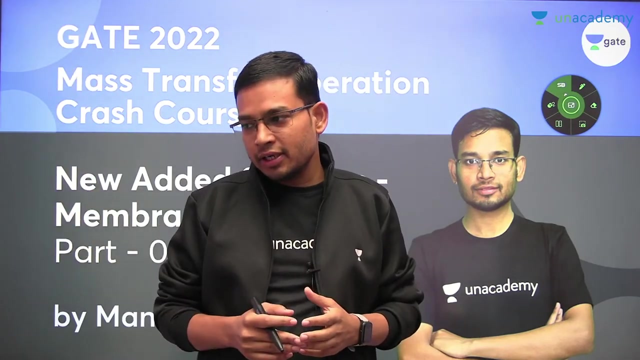 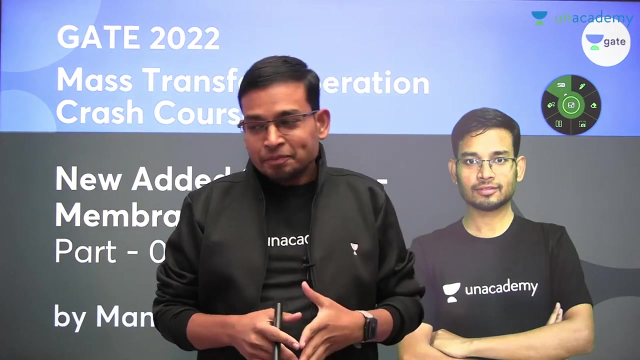 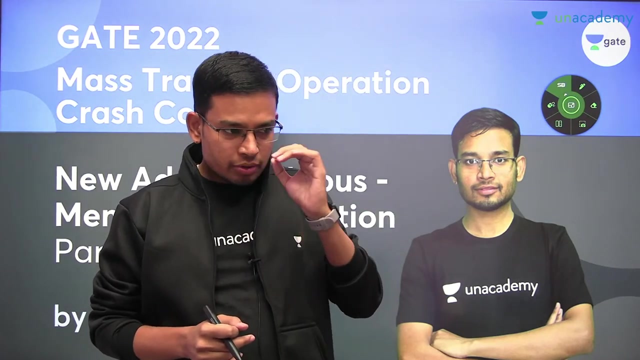 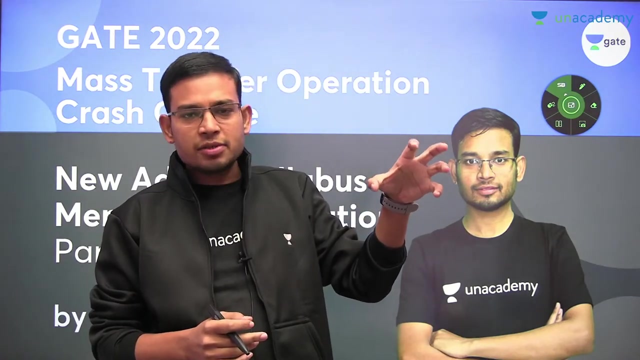 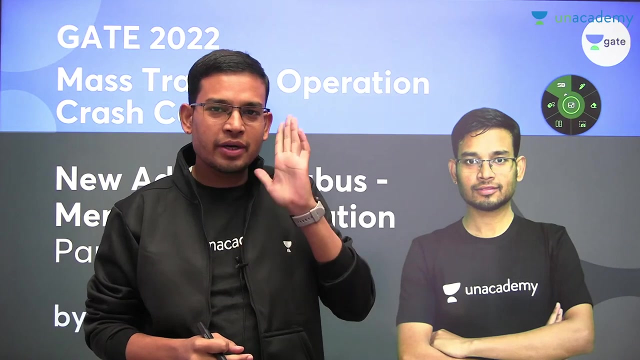 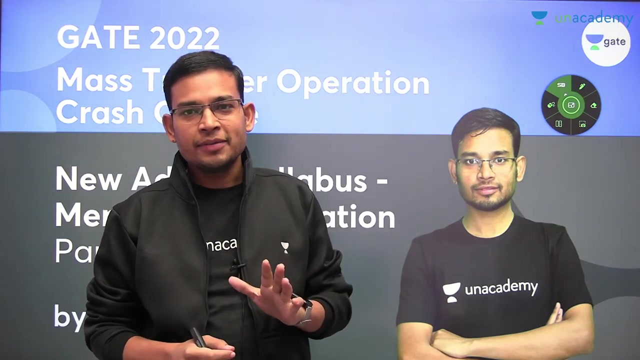 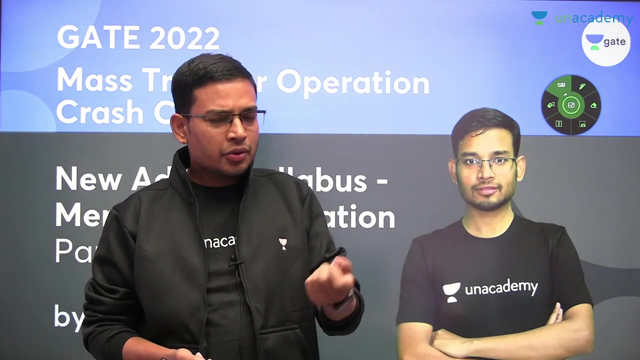 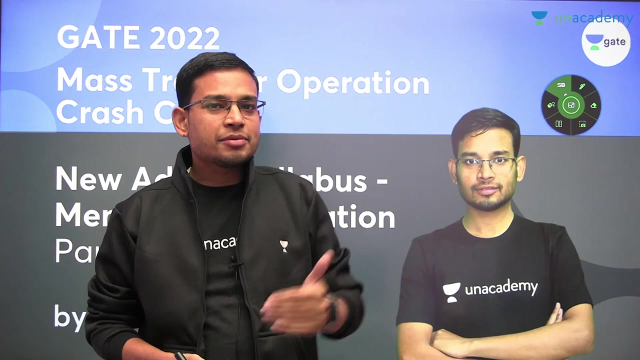 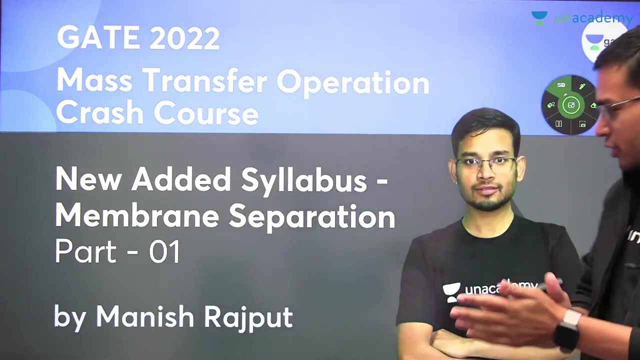 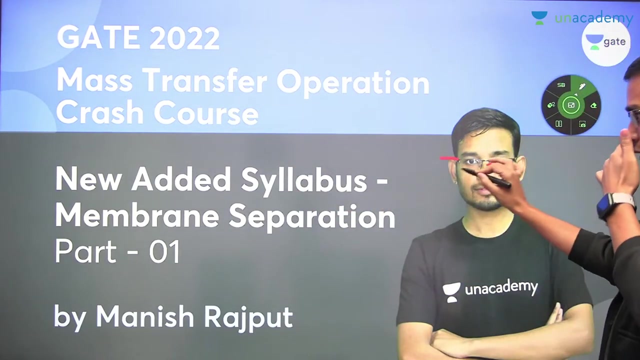 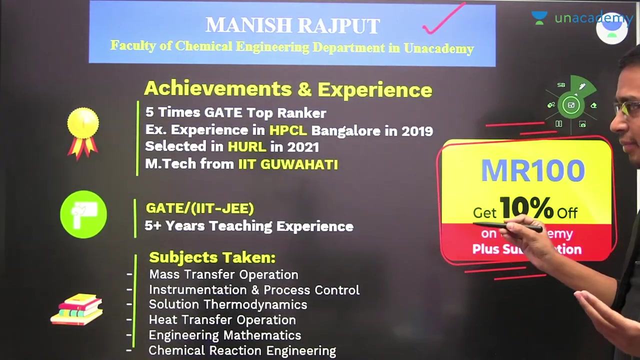 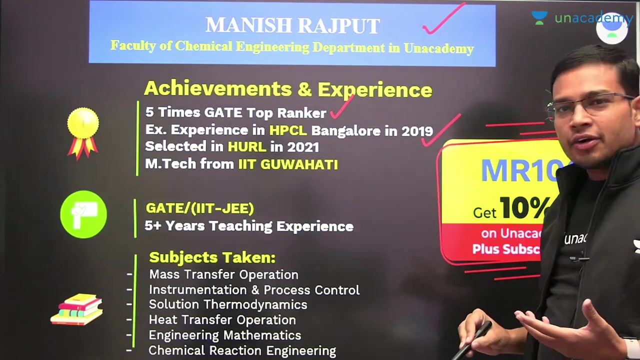 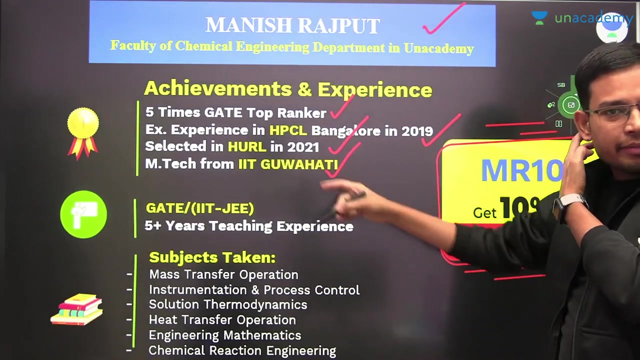 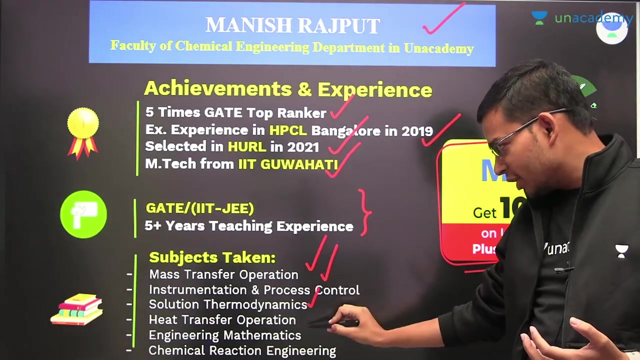 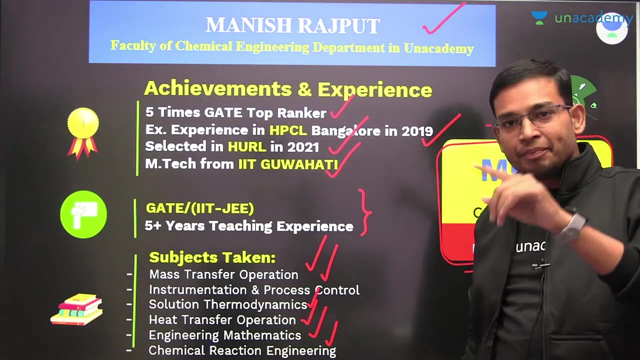 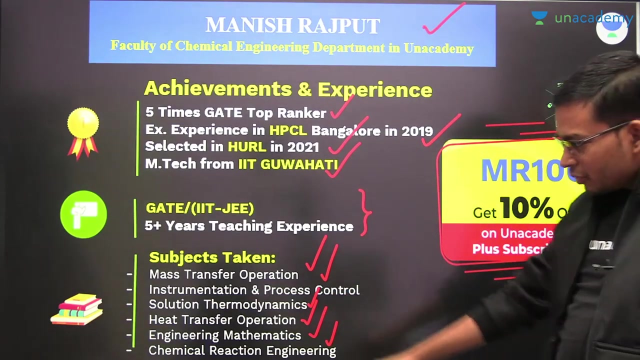 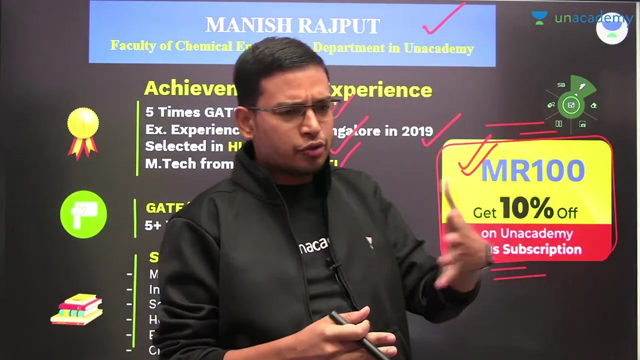 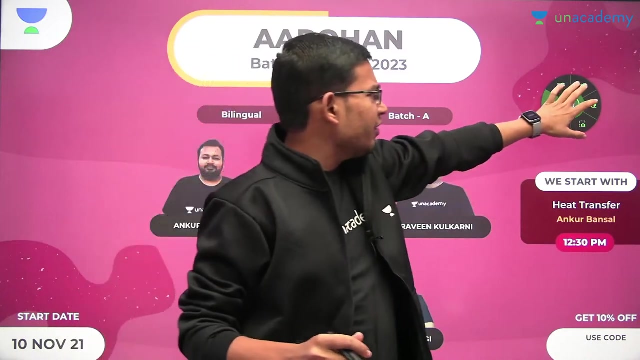 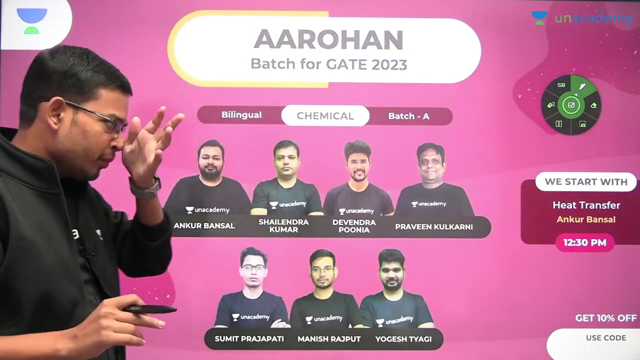 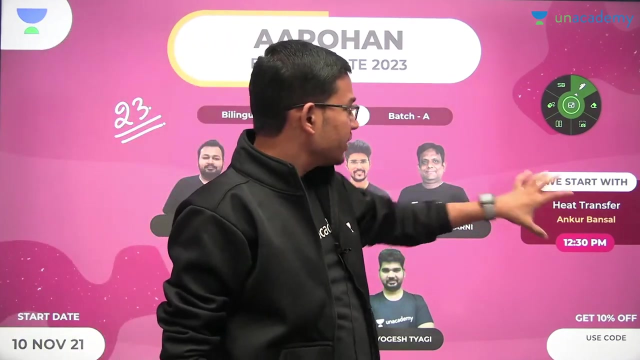 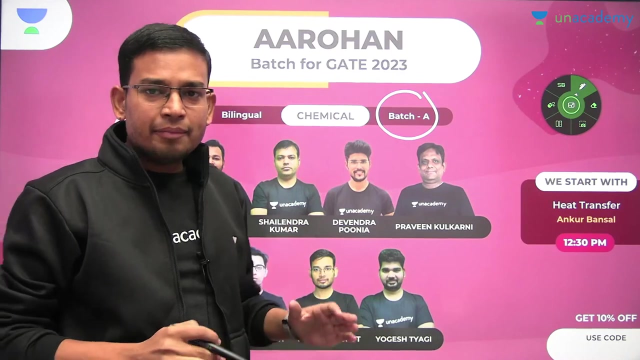 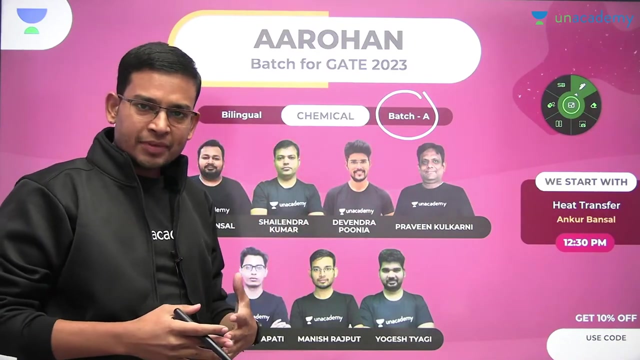 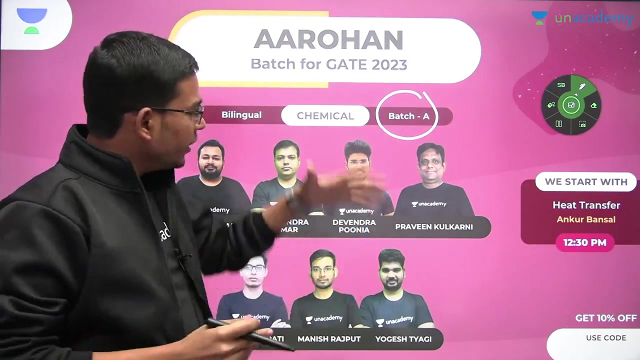 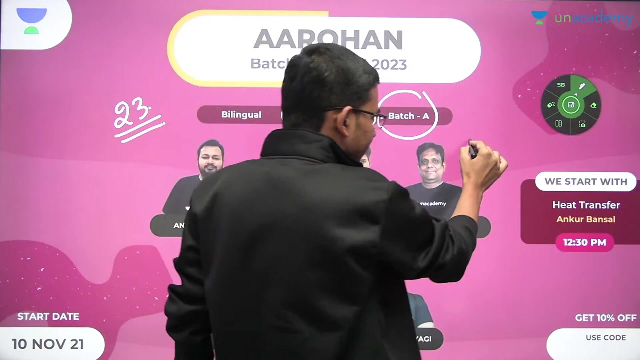 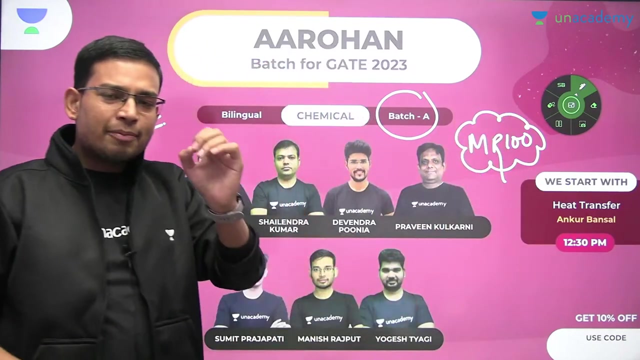 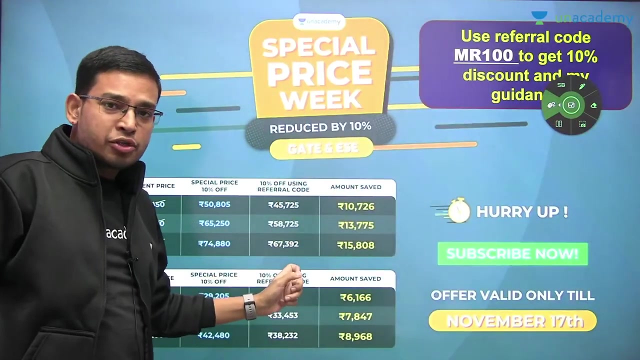 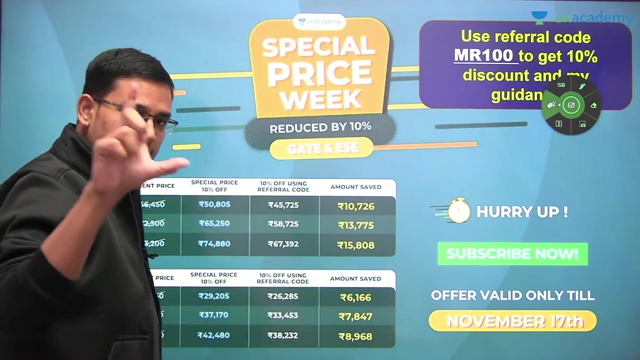 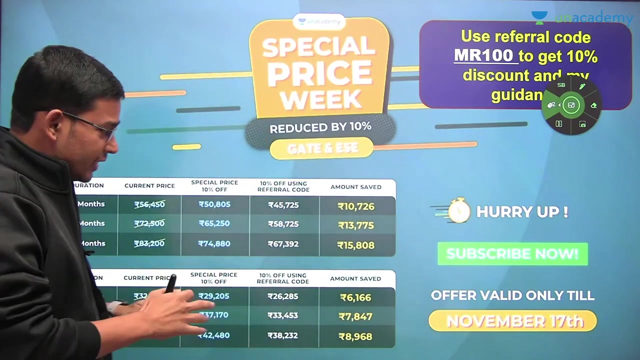 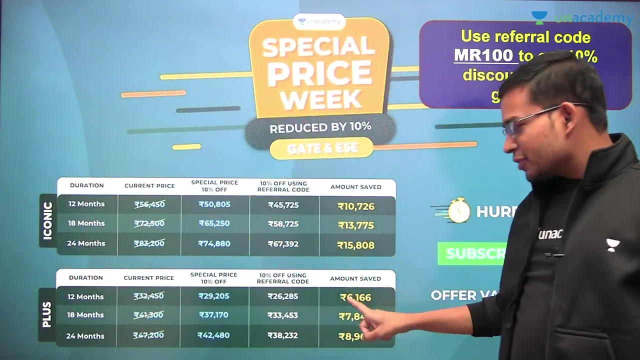 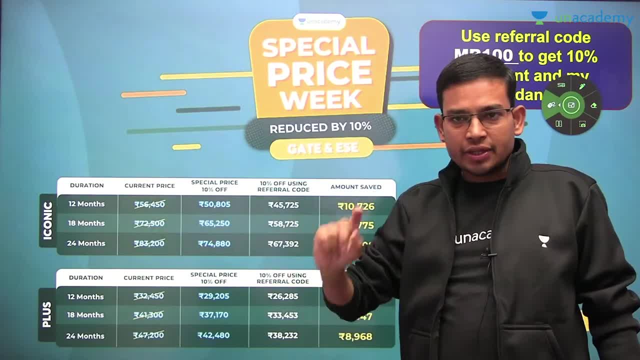 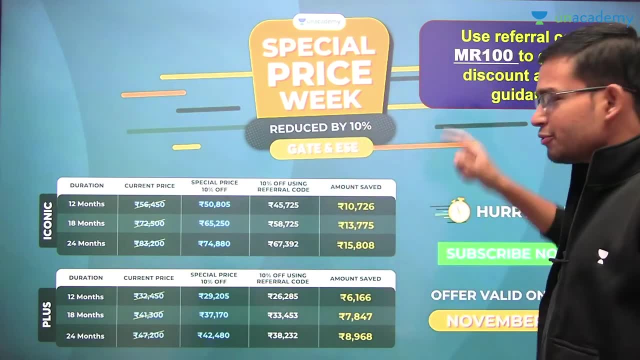 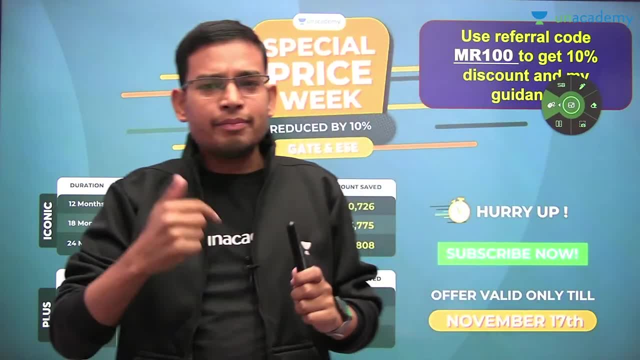 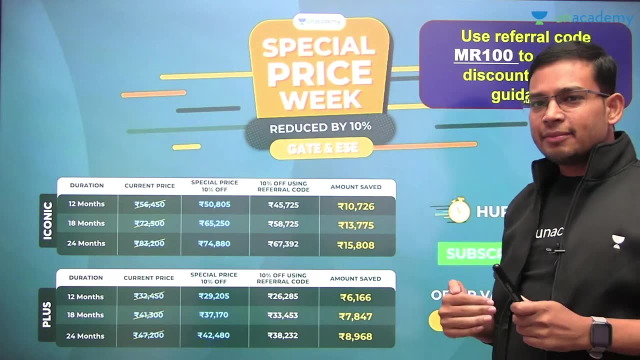 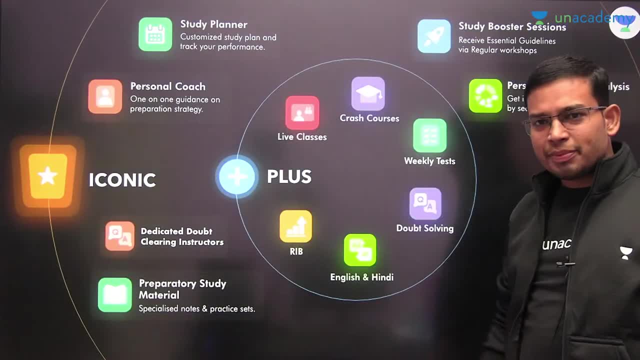 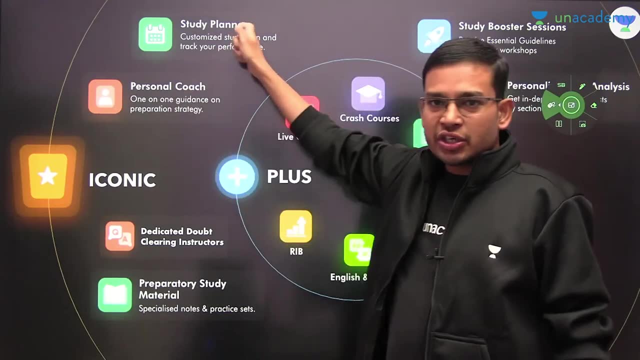 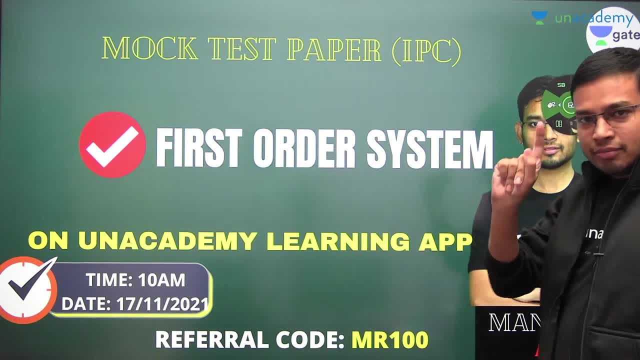 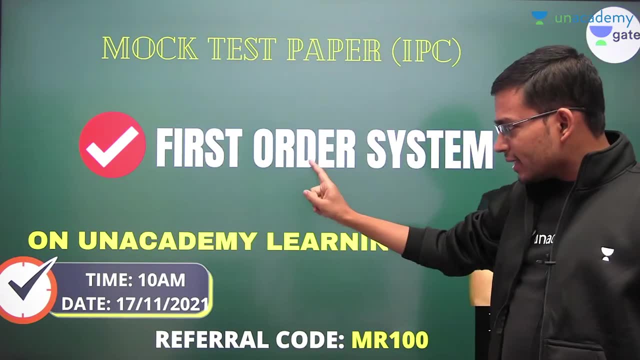 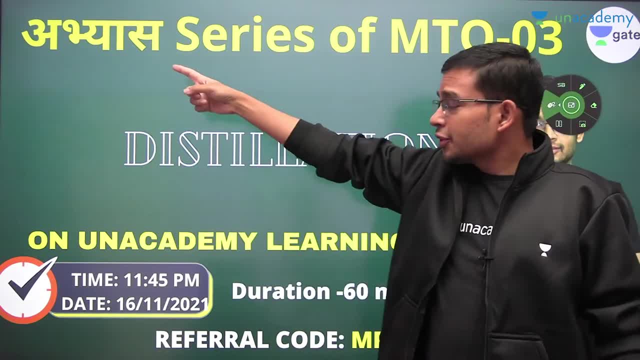 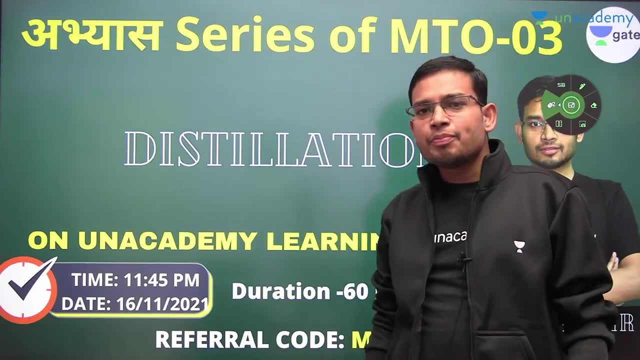 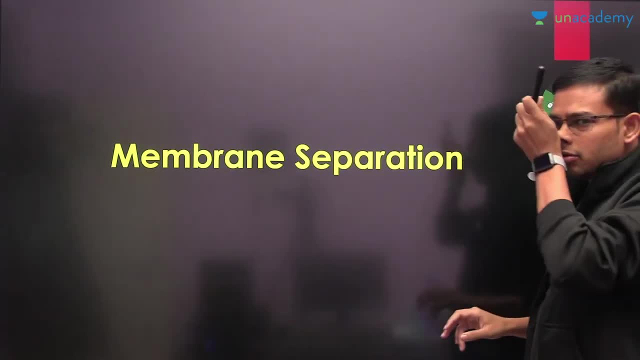 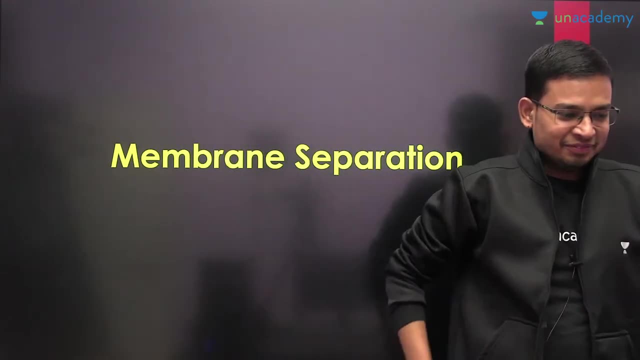 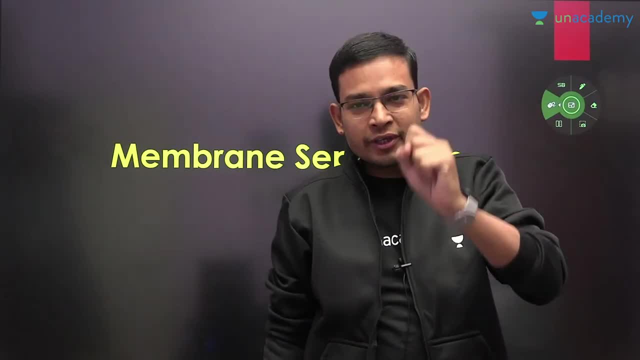 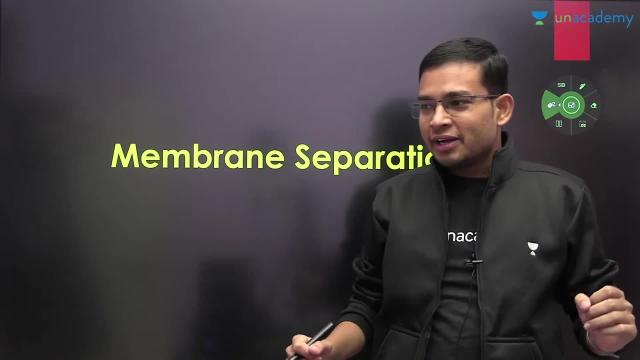 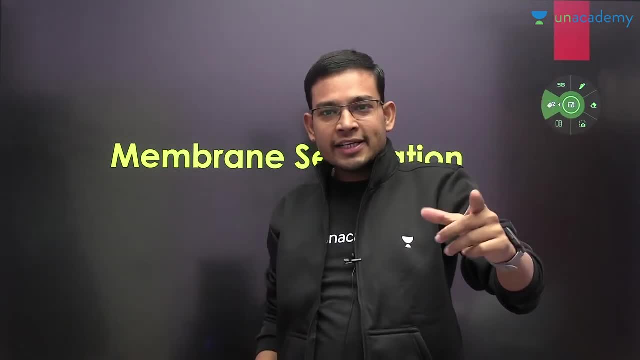 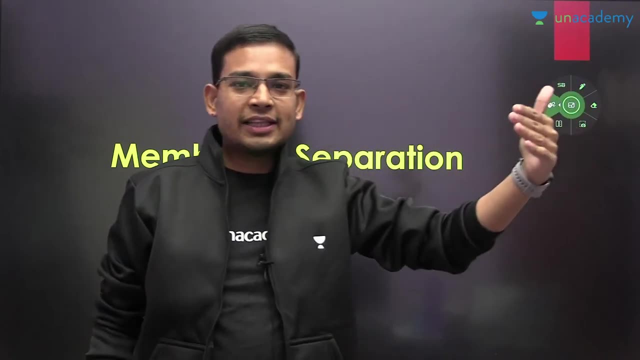 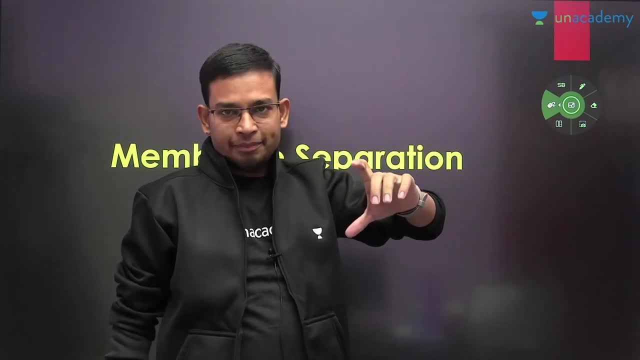 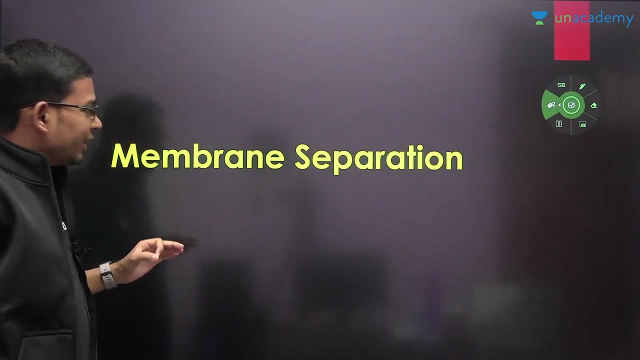 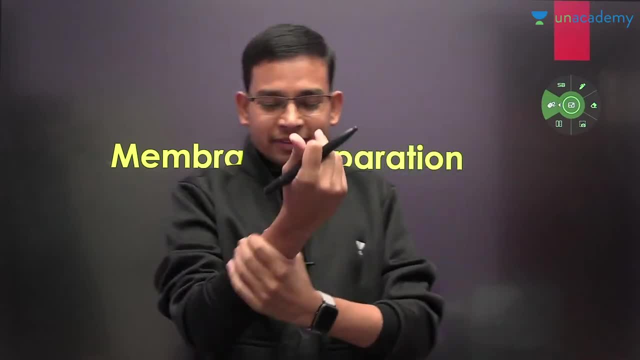 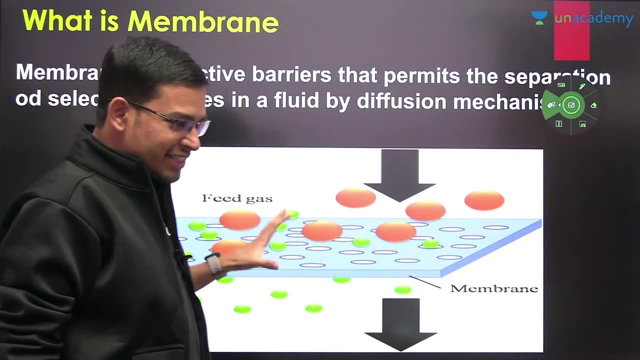 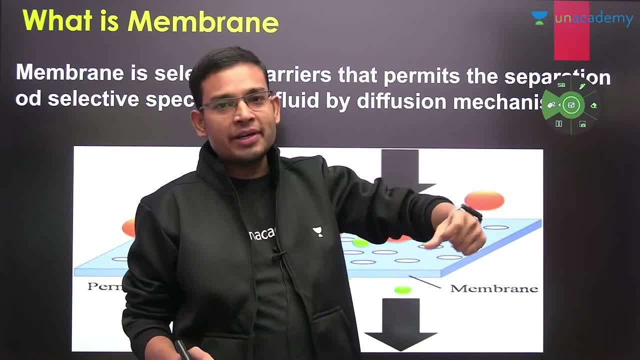 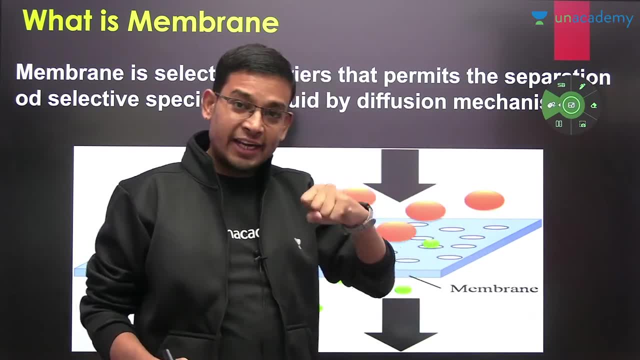 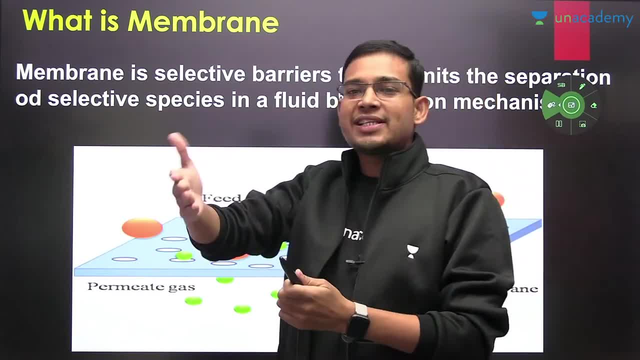 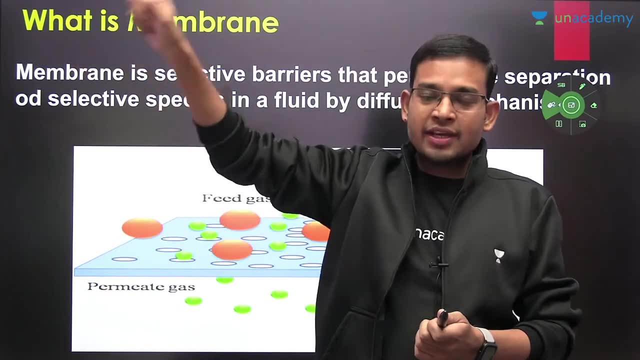 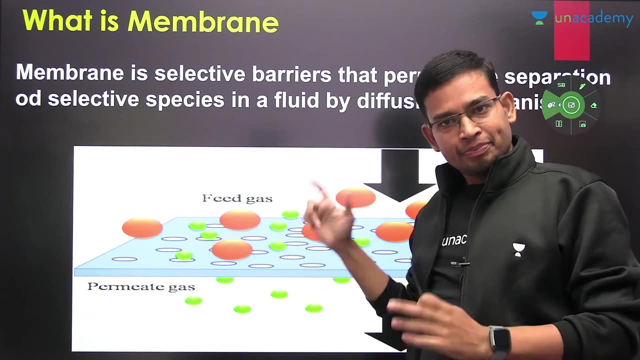 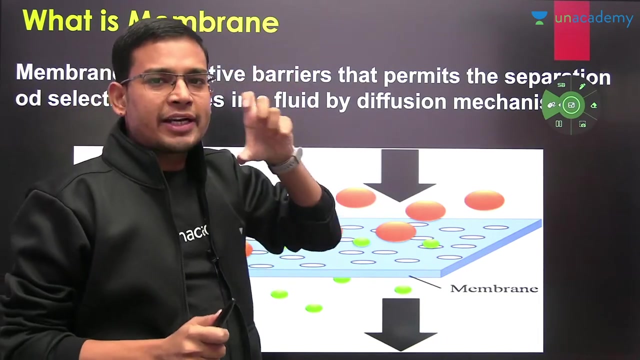 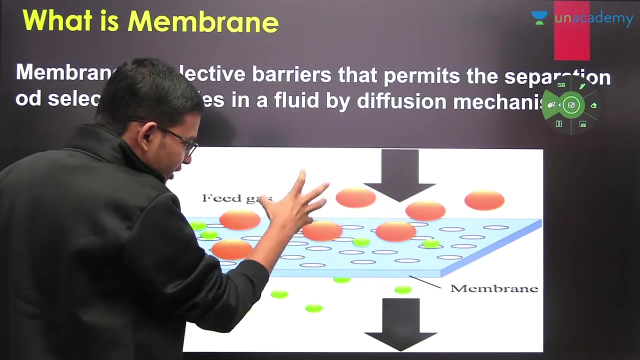 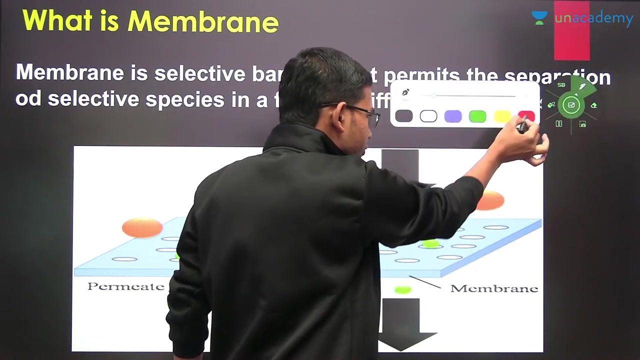 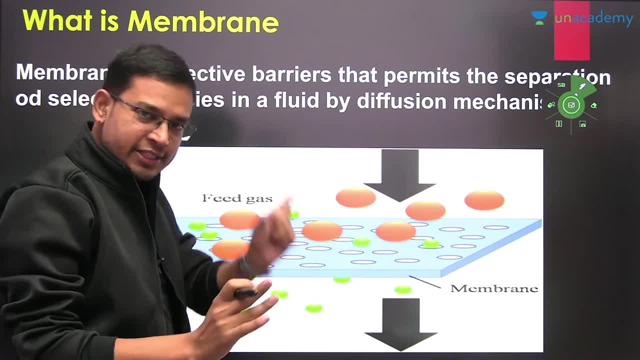 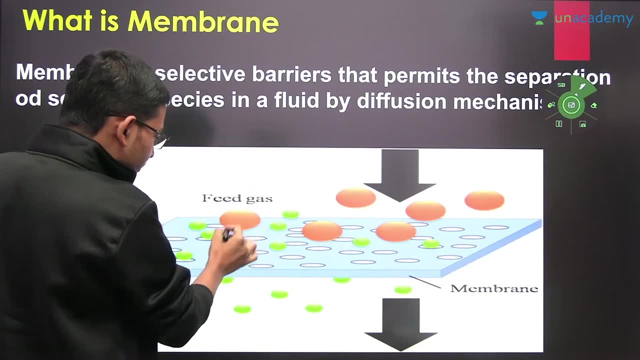 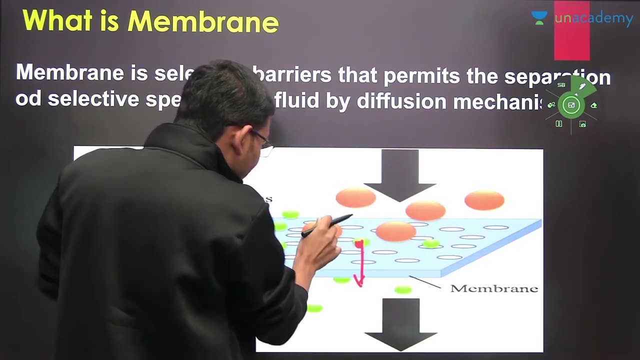 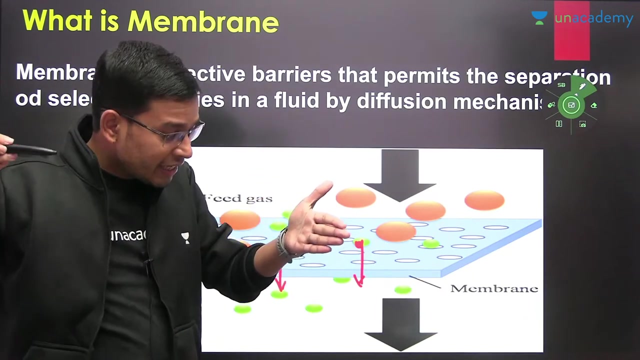 what is this Membrane doing? it is a selective barrier. selective barrier it is not a barrier that you are not able to go out. this type of barrier is not there. this is selective barrier. selective barrier means that it is passing particular molecules. it is passing particular molecules but not passing some molecules. this is called Membrane. okay, Membrane will not happen. that there is no Membrane, then nothing is passing right. so this is not called Membrane. 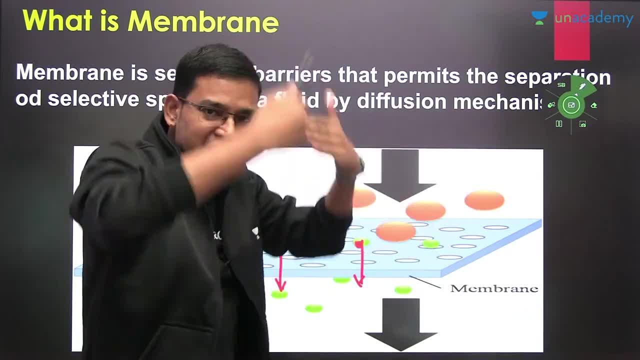 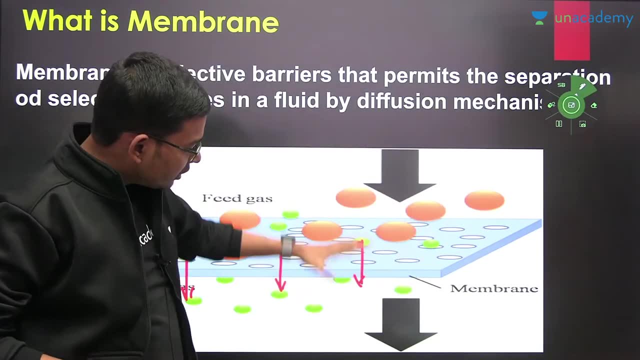 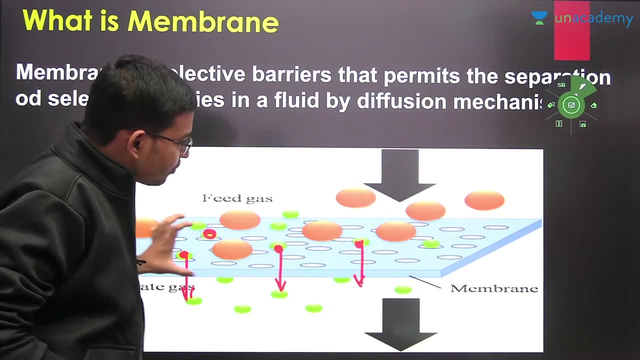 It will pass out some selective particles and will retain some of them. It will permeate some of them. So the side which is removed from the particle is called permeate. This is our product, pure form. This is called permeate And the thing which is retained is called retentant. 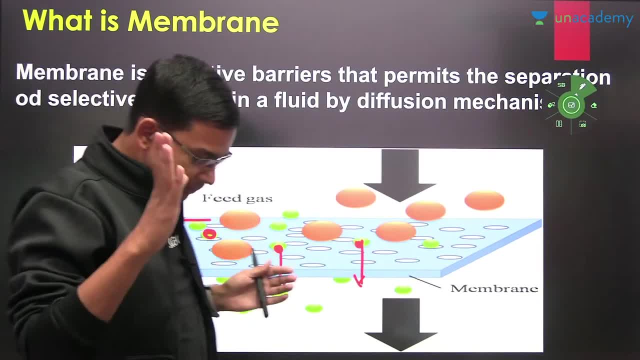 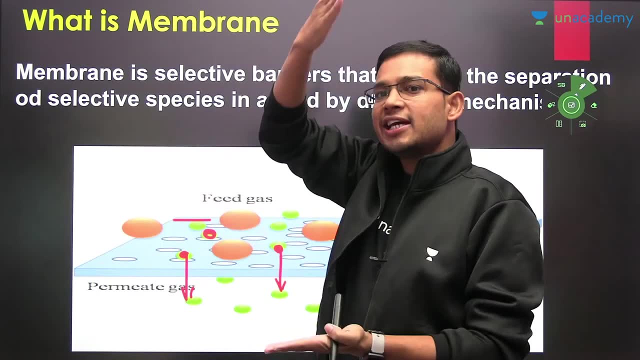 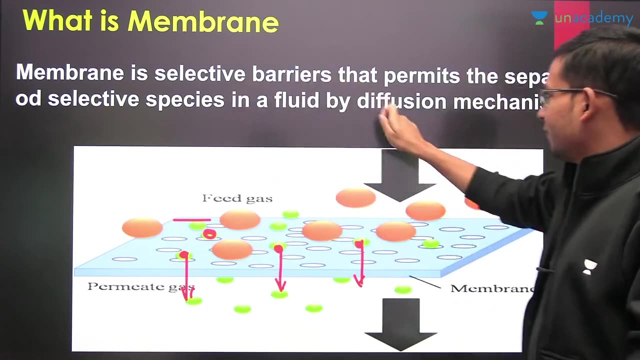 Now we will study this properly. So, first of all, we should understand that: membrane separation With the help of membrane, Membrane separation With the help of membrane. Okay, So you understood membrane, It is the selective variable that permits the separation of the selective species. 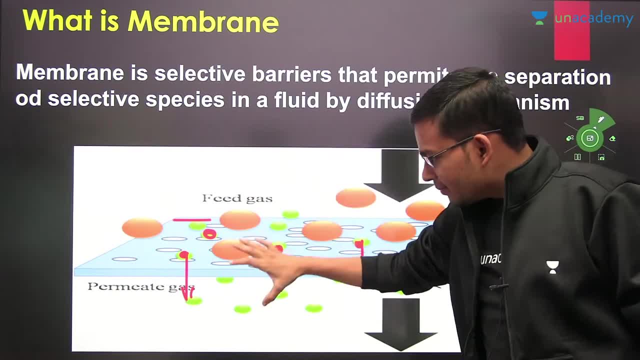 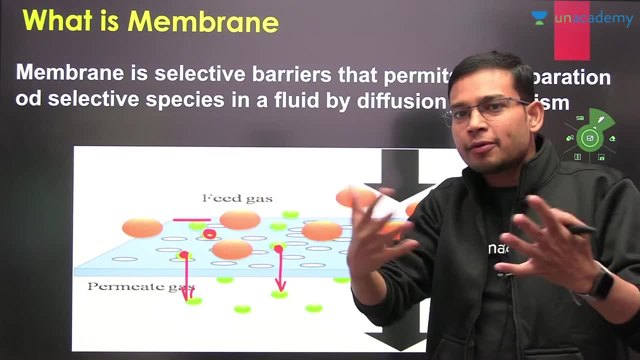 It will allow some selective species to permeate. Permeate means what is removed. This is the permeate. This can be gas or this can be liquid. Right, It is not necessary that only liquid will be separated. No, This gas is also in the membrane separation chapter. 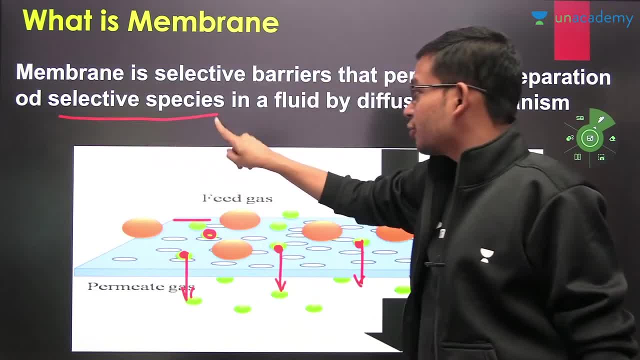 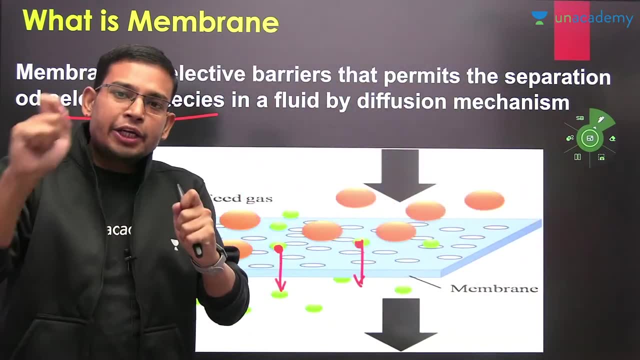 So gas is also there. Some selective species will be passed. What will be its mechanism? Diffusion, Whatever mass transfer you will see here due to diffusion Right. So what will you see its mechanism here? Diffusion Particles will be diffused. 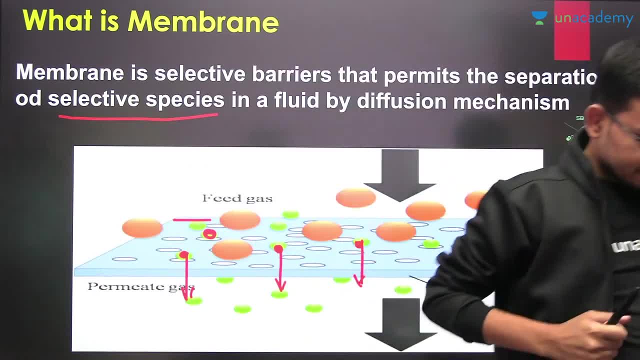 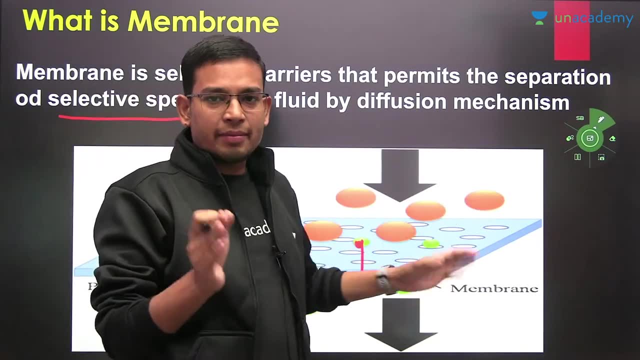 Right, Particles will be diffused here. Okay, Very good. So what is this? Yes, Semi-permeable membrane, Very good. So how is this membrane? Semi-permeable Means it will stop some parts, It will pass some parts. 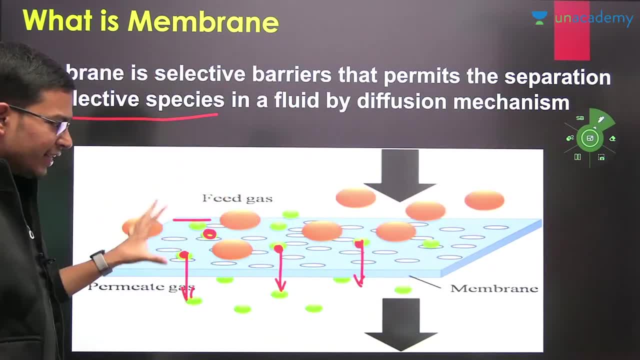 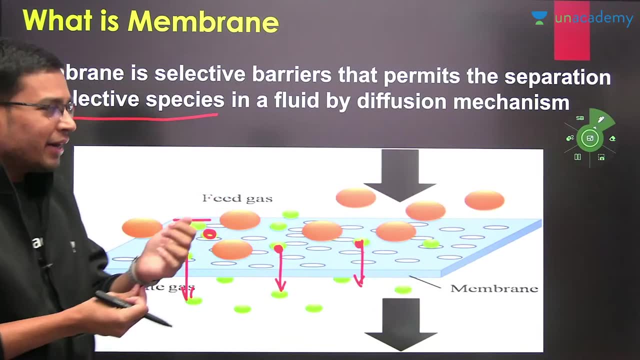 Okay. So this much we should understand. Everyone will write in one line in a very nice way, Characteristic of the membrane. Read it at the speed of 2x. Yes, Absolutely Okay. Everyone will write: What is the definition of the membrane. 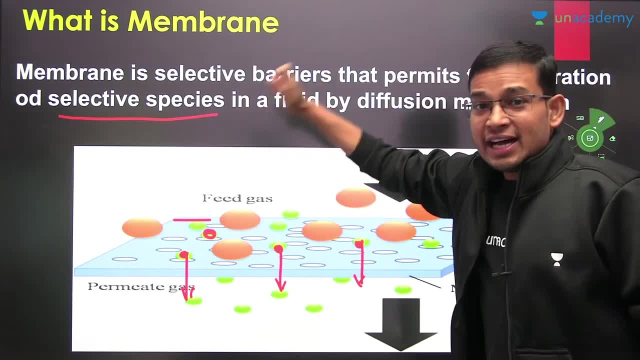 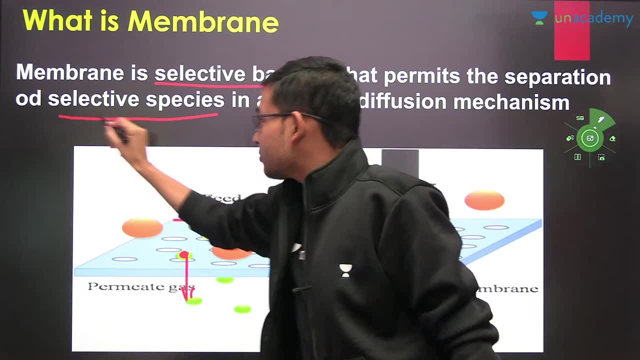 First of all, membrane is the selective barrier. It is the selective barrier. We will underline What is this selective variable That permits the separation of the selective species. This is a selective variable that permits the separation of the selective species. This is a selective variable. 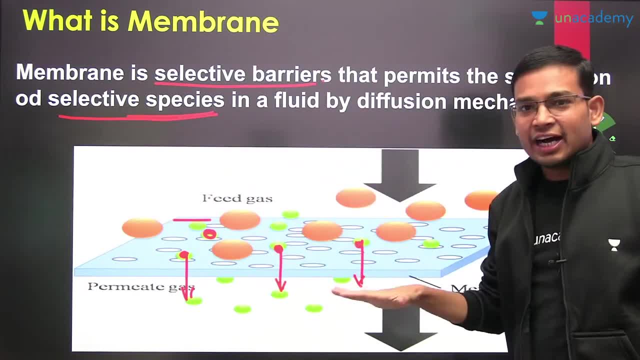 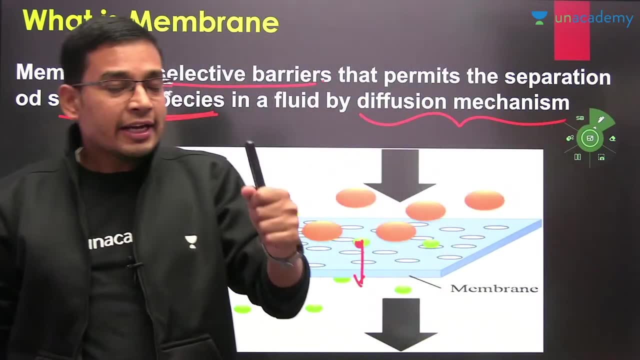 A characteristic: More species to permeate. that is called membrane take. it is key to make me. am I go? mechanism cat diffusion is key. mechanism cat diffusion, Sarah, look at them. it's not mention carrying it for me. I give it to him. it's not sorry, look at. 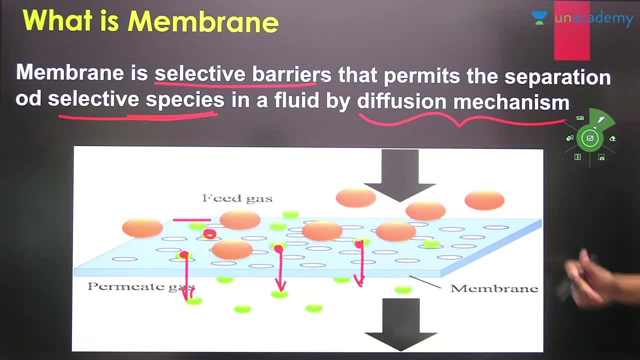 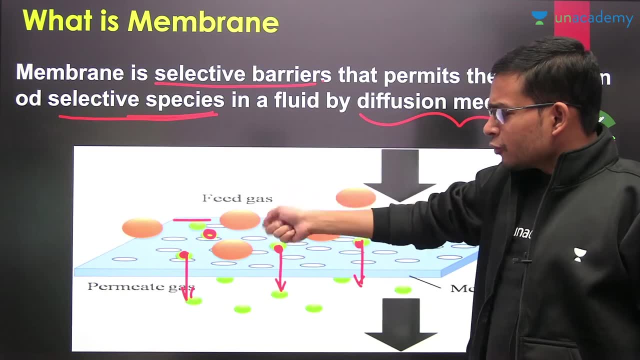 me copy my mention, carrying it, then we will move. for next, take it to you biblical, up to clear. oh yeah, oh god, key membrane kiya hai to membrane ke bari me buku, samajh me aagaya kiya, we are selective of barrier a jo ki selective. 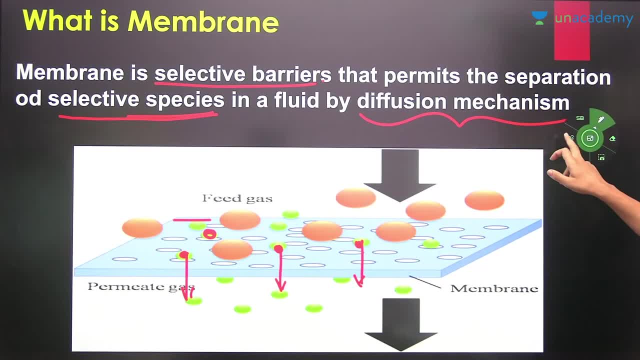 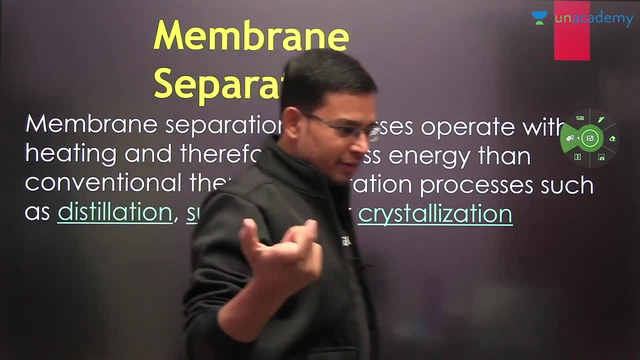 species ko pass karega right. this is called membrane. now come to the next point. I may suggest bottom of. what is the membrane separation, guru membrane separation kiya hai? take a quite absolutely put today what is the membrane separation? the membrane separation came a paper about Karuna. 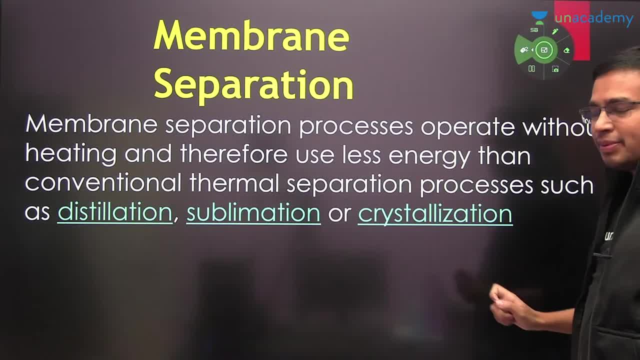 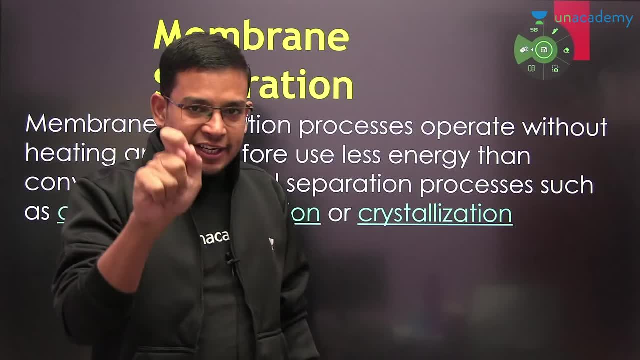 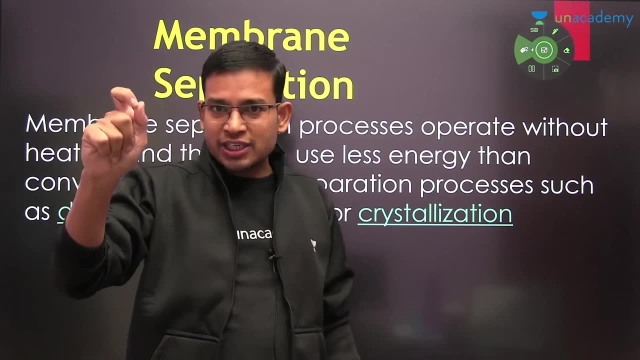 membrane separation is the process that operate without heating. take a: yes, honey, Yogi heating k threw up. it's no blue Colibri eating in. involving Yogi energy in wall. Maxine Minam energy restraint. ller Heating energy involved. less energy involved. without energy involved. 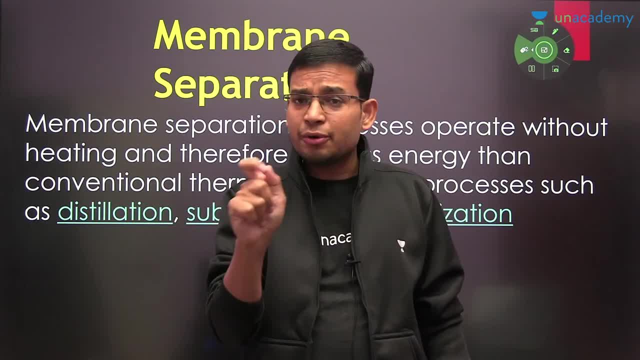 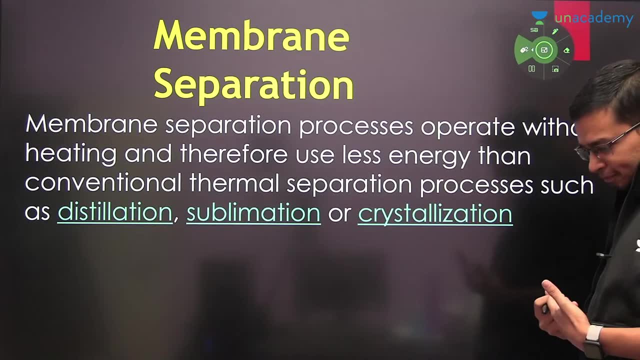 You can make such options. So what will happen in membrane separation? What happens is that energy is very less involved. Otherwise it will become a heat transfer process. So everyone will see what is the membrane separation. What is membrane separation? 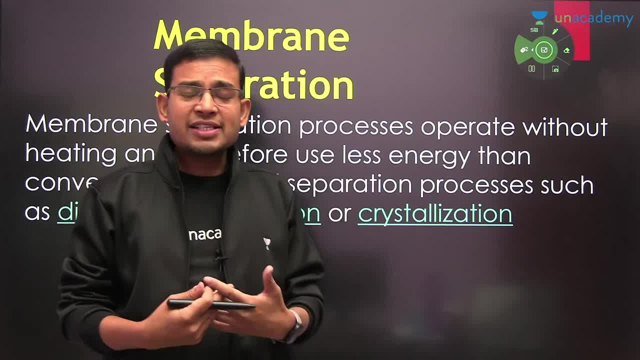 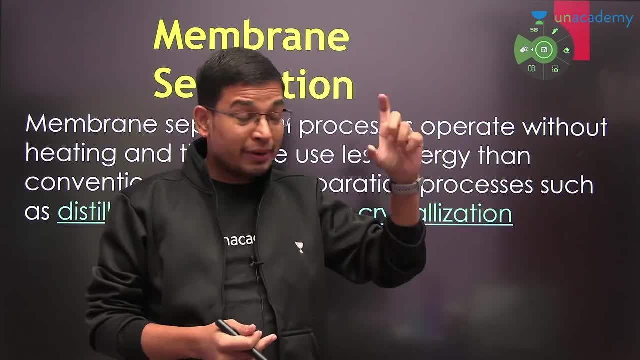 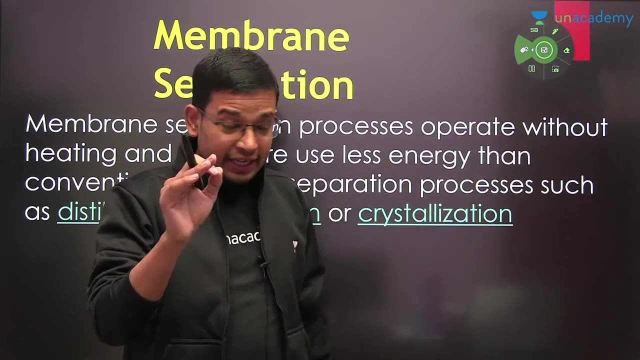 It is also separation technique. What is membrane separation? It is also separation technique which separates some particular species of eye. What will it do? It will separate particular species, As you saw in membrane. What will happen Without energy? There is one more important point. 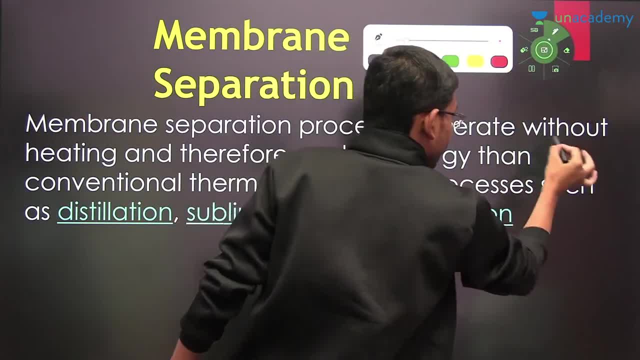 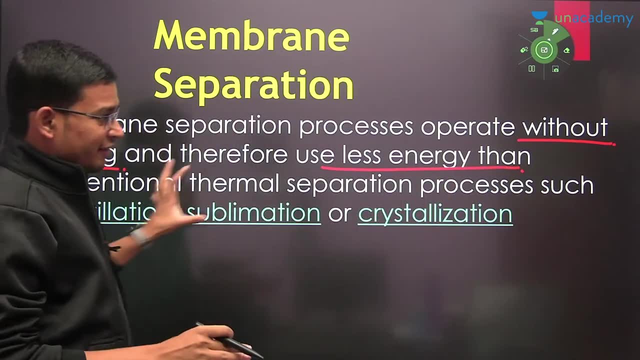 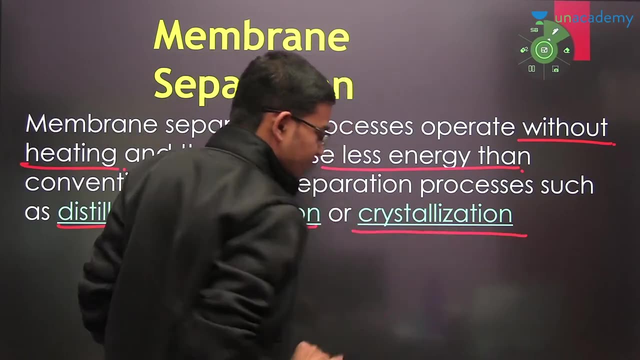 What will operate without energy, Without heating? Therefore, less energy than conventional process. Conventional process means, like you had studied, distillation, sublimation, crystallization, Sublimation is also part of separation. Okay, You didn't talk about this yet, but yes, you must have studied thermodynamics. 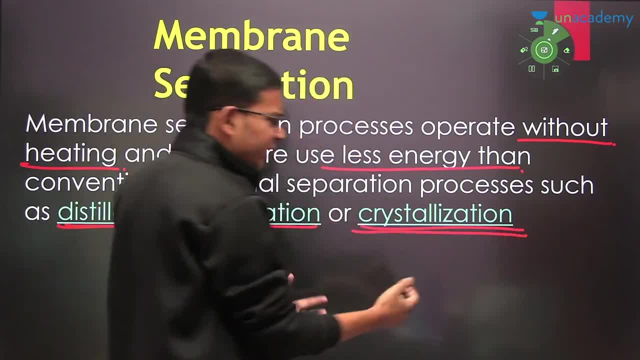 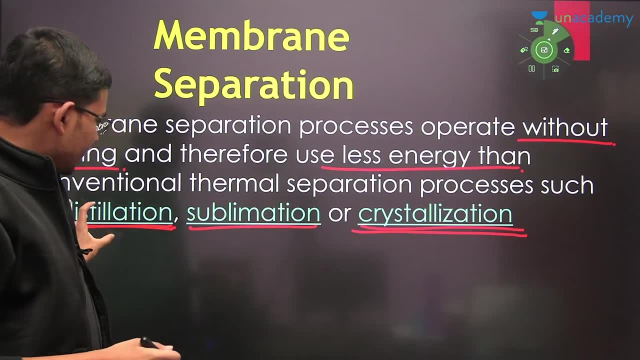 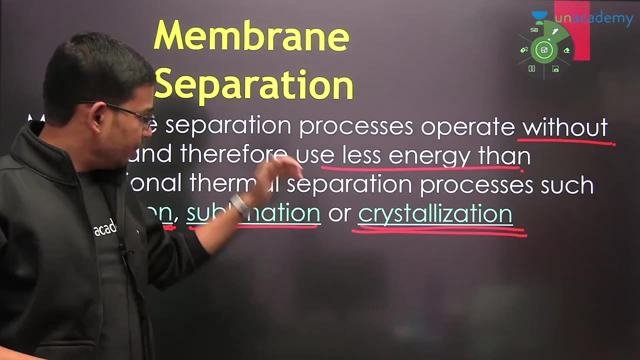 So what was the distillation here and what was crystallization here? Heating was involved here, right. What was here? Heat was involved, but heat is not involved in membrane separation, right? So in distillation you saw that this is also separation technique, this is also separation technique, this is also separation technique, but your heat was involved here. 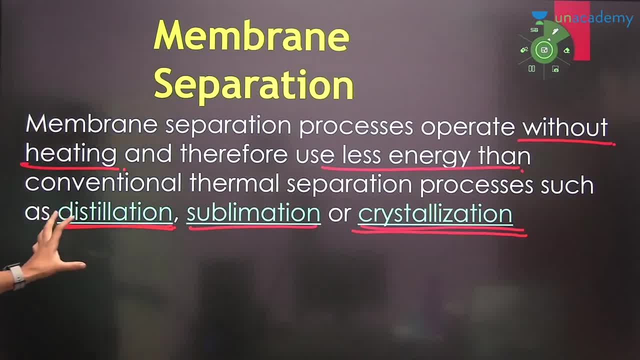 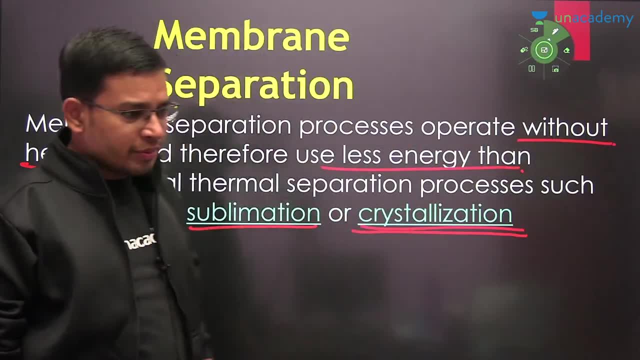 But here there is no heat involved. Everyone will write the definition of this. then we will move forward in a nice way. Everyone will also write the definition of this. Yes, I will tell you the driving force. now, Yogesh, We will come forward. now we will make all the things one by one. 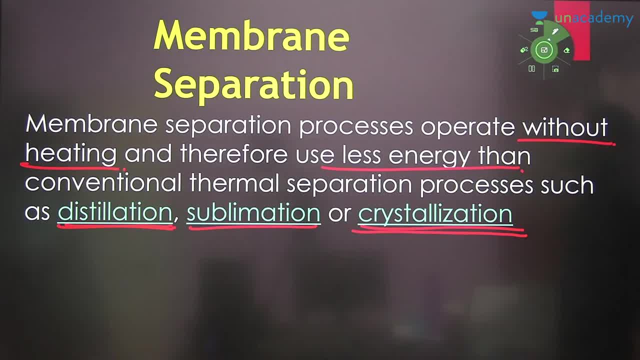 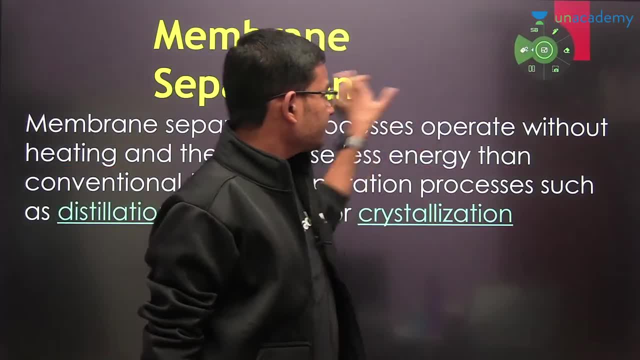 Right now the very basic things are going on. Okay, in this there will be different, different driving forces for different, different processes. We will talk about it later. First, take a big idea. what is the process? Now? I will talk from here. 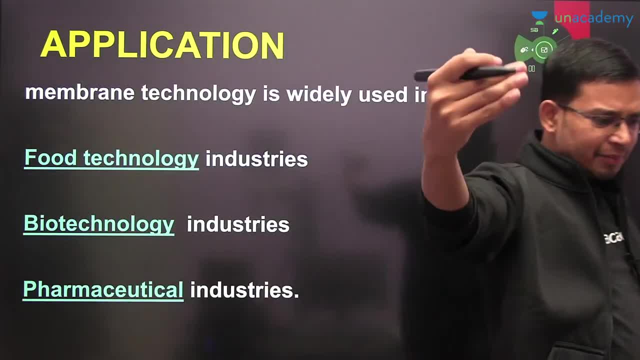 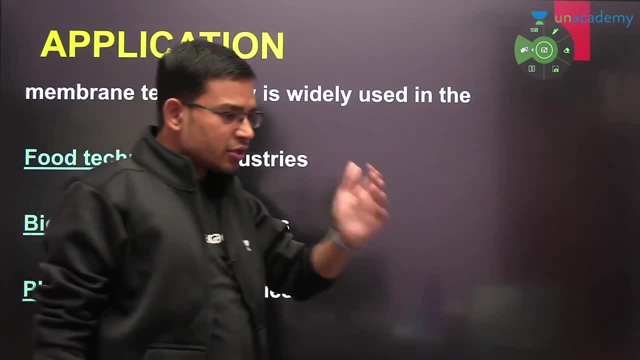 Applications. Where will you get to see the application of membrane separation? Yes, so due to concentration difference, your membrane separation will also happen. Here also, the separation will happen- Concentration difference. Like your temple, Like what will happen to you. 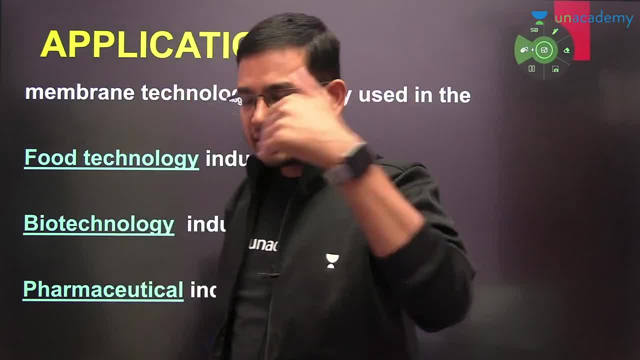 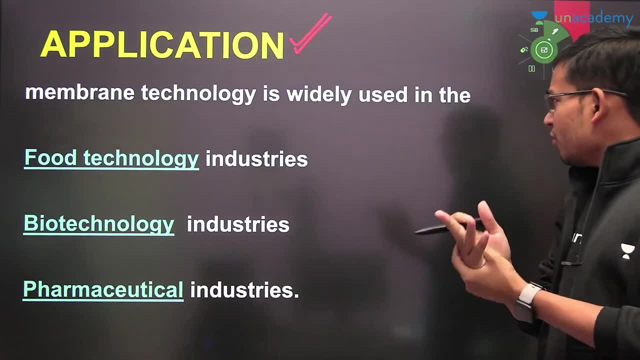 Ultrafiltration, nanofiltration, where do they all depend? Concentration difference- Okay, now it will come forward. So first take a big idea: where do they use it? So the application of membrane separation: where is it widely used? 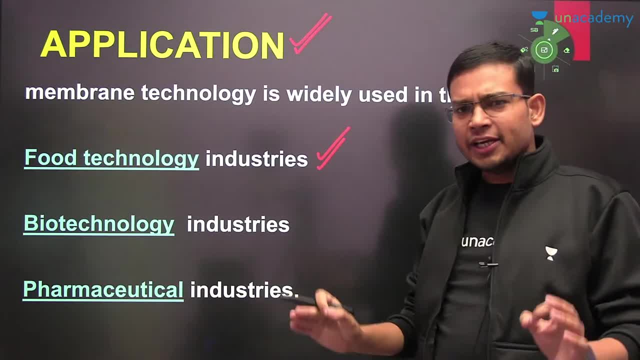 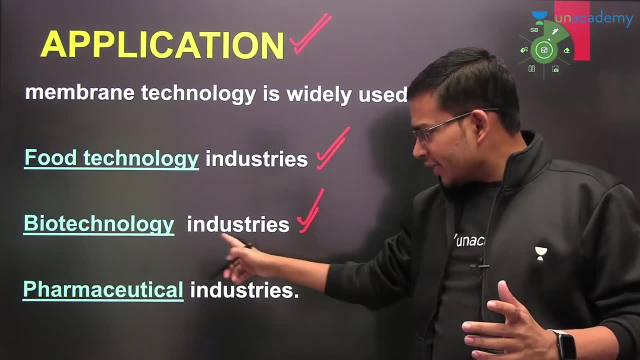 Food technology: Okay, in all the food industries there you will get to see the use of membrane separation. Second, biotechnology industry. Okay, where is all this biotechnology? Where it works at your normal temperature, Okay, biotechnology industries. 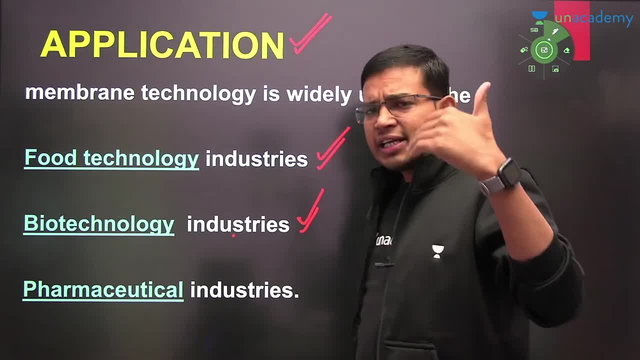 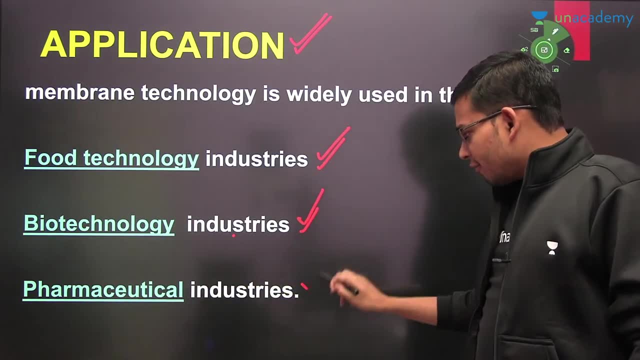 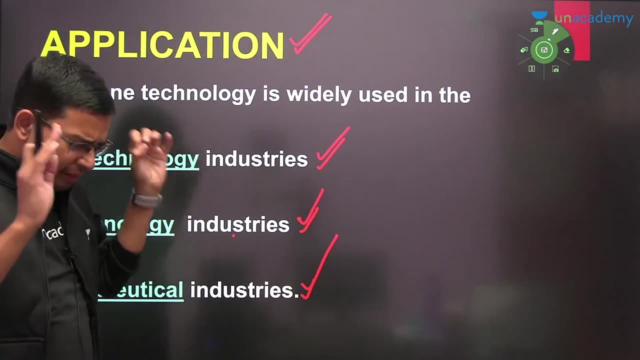 Here. what is your membrane separation, Where your particles are heat sensitive. So what will you use? there, too, You will use membrane separation. Okay, like pharmaceutical industries, Membrane separation is widely used in the pharmaceutical industry too. Right, so we should understand this much that, where it is used, 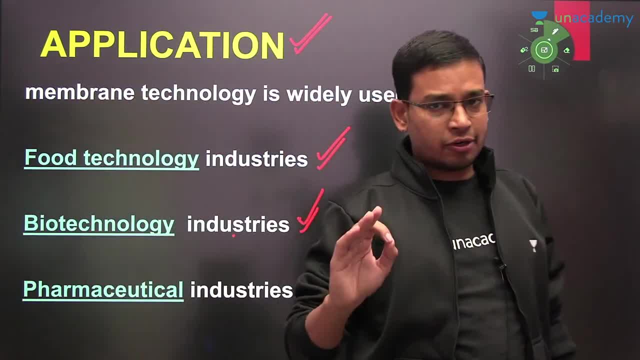 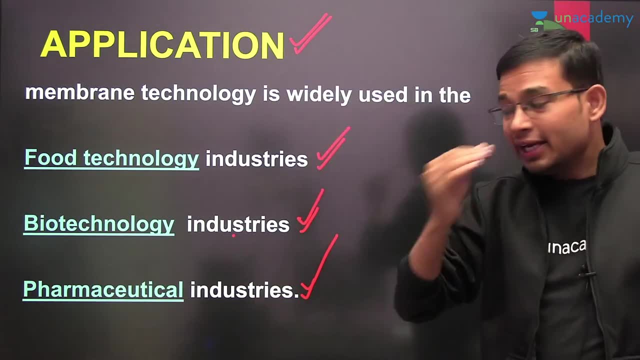 Number one, which is used the most drastically. that is the food technology. Okay, food technology is used a lot in industries. Second, biotech and pharma. It is used in many other places too, But the major use of it is food, bio and pharma. 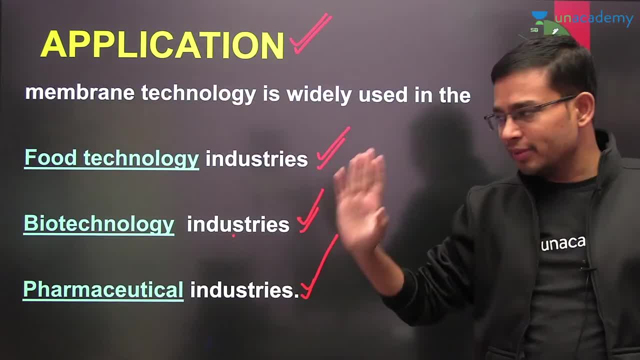 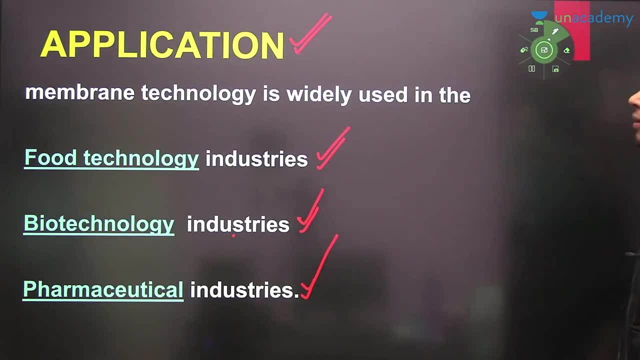 Okay, in these three industries you will get to see a lot of use of it, Right? so all these three people will keep writing applications, one by one. They will keep mentioning one thing in the company: Okay, there is application of the membrane separation. 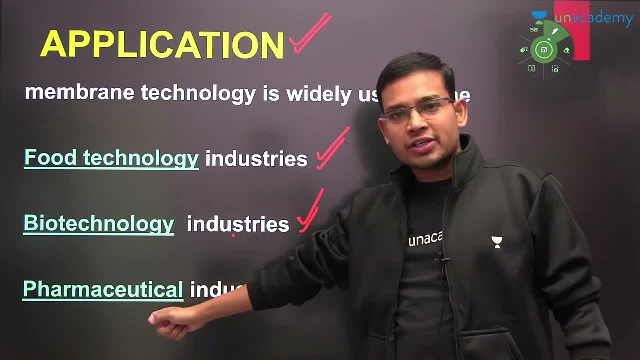 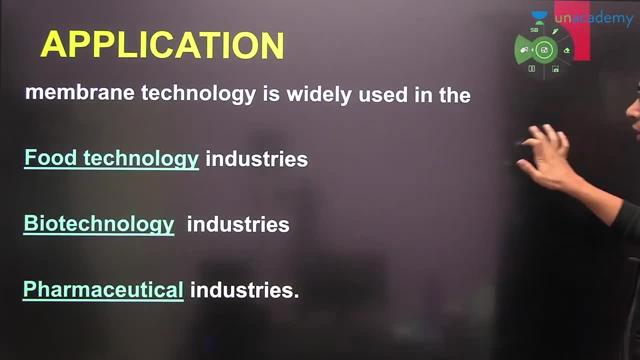 Okay, so where will it come? In? food technology, biotechnology and pharmaceutical? Okay, so in these three places you will get to see the application of membrane separation widely. Now come to the third point Now: types of the separation. 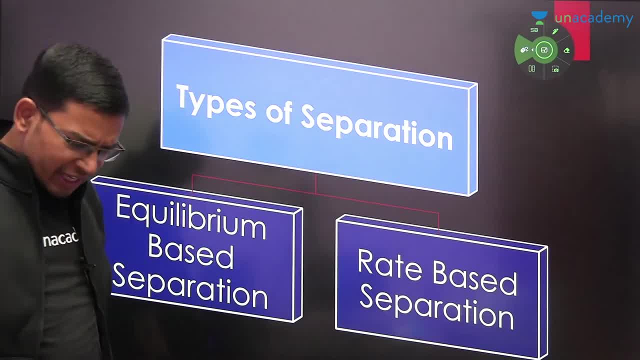 What we will talk about here, how many types of separation we will talk about. Now you are a little involved in the picture from here. You have started to get a little involved in the picture. You have started to get a little involved in the picture. 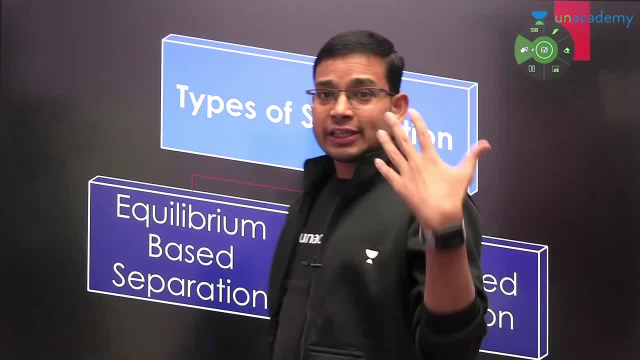 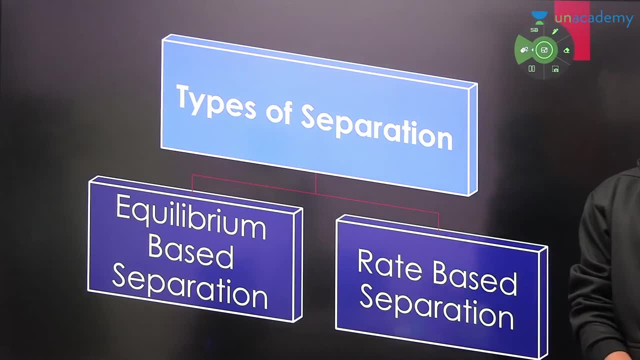 Yes, two gases can be separated from the membrane separation. Okay, gases and liquid. both can be separated by the membrane separation. Now, the driving force will come in the picture. Yogesh, just chill. Okay, the driving force will come in the picture. 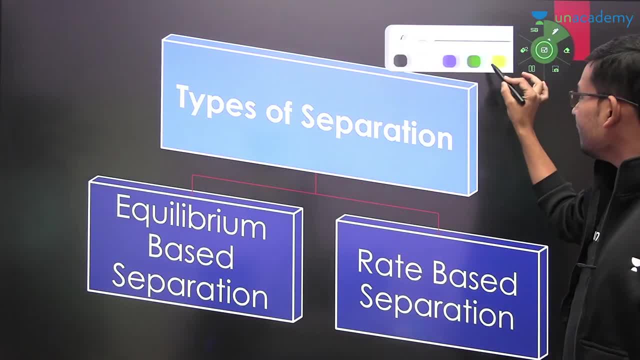 Now we have not talked about anything. Now we have not talked about anything mathematically. Okay, now I am giving you just an overview. So what will happen here? There are two types of separation. Okay, you have to see very carefully. 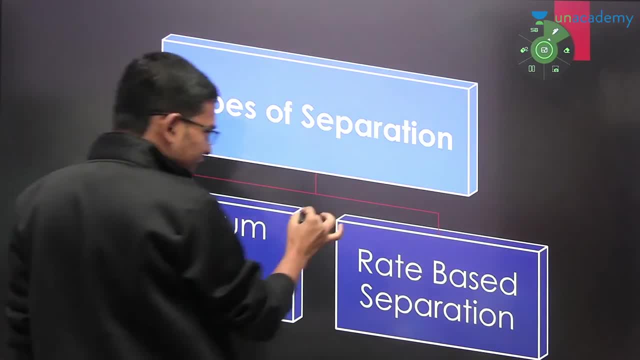 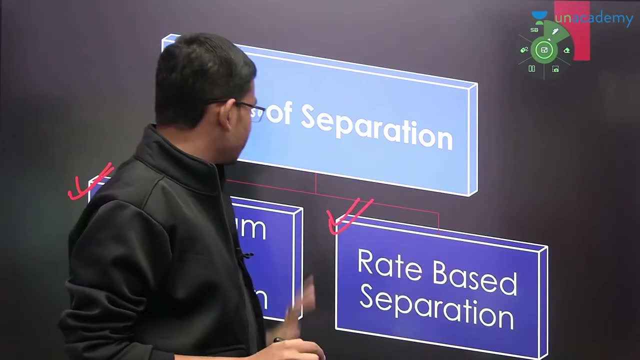 There are two types of the separation. One is the equilibrium waste, The other is the rate waste. Okay, one, you will get to see the separation- Equilibrium waste separation. The other, you will get to see the rate waste separation. Now look. 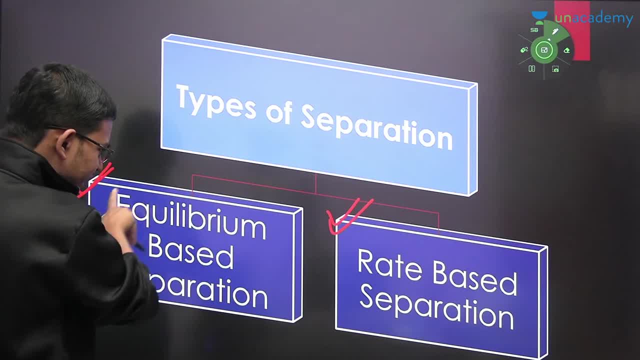 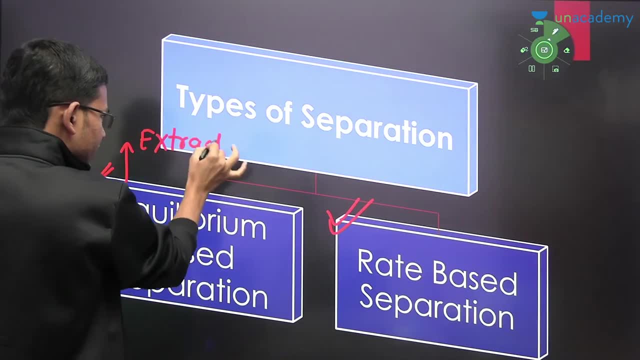 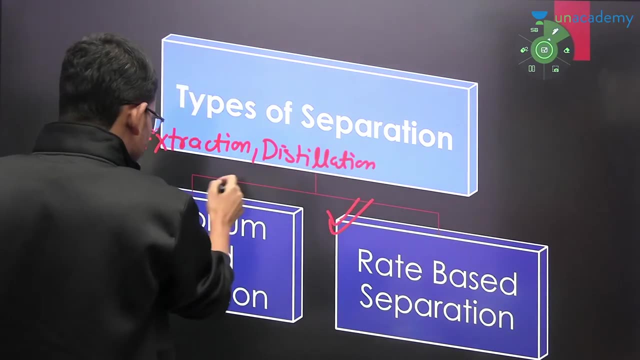 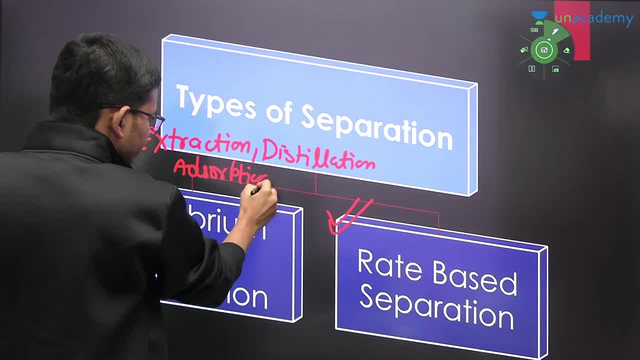 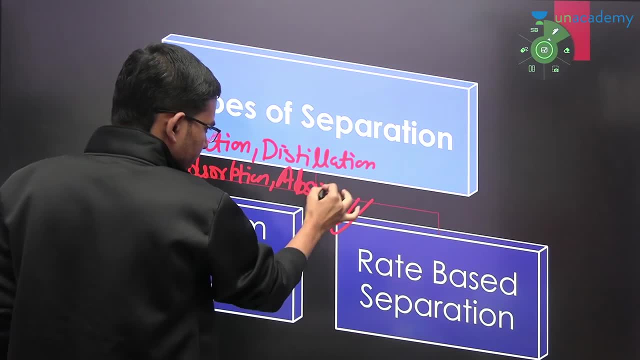 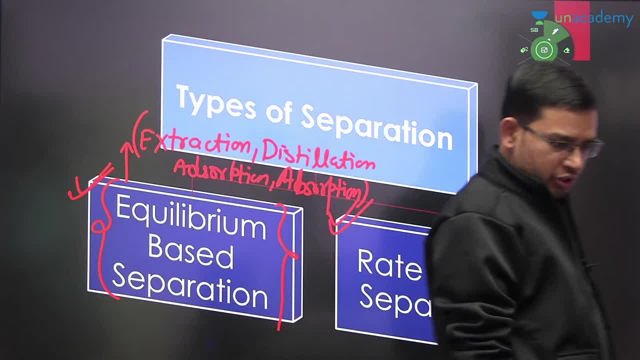 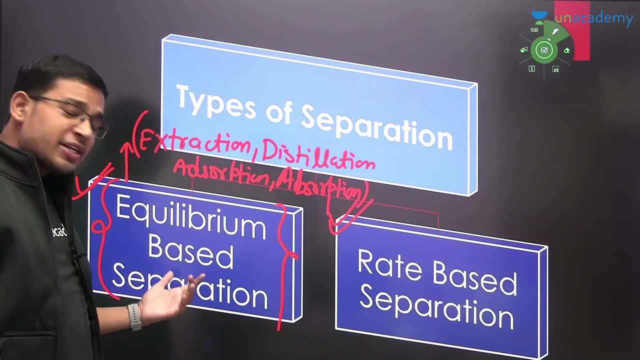 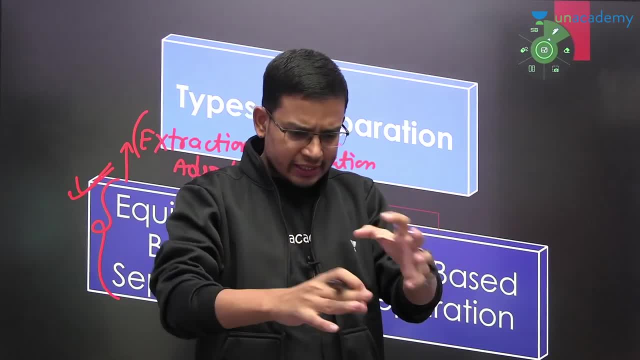 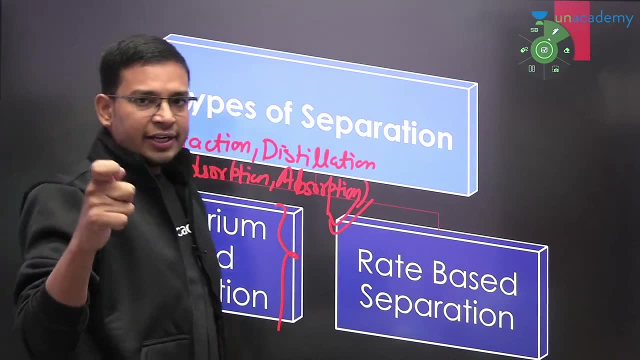 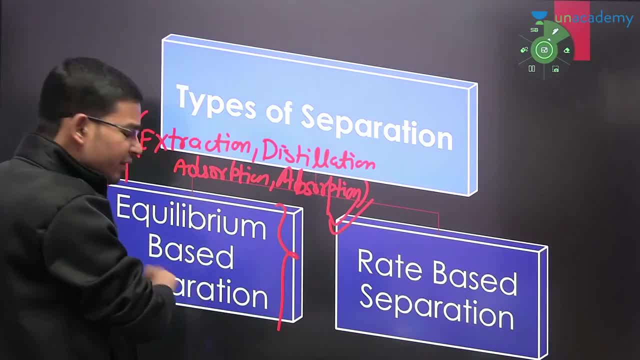 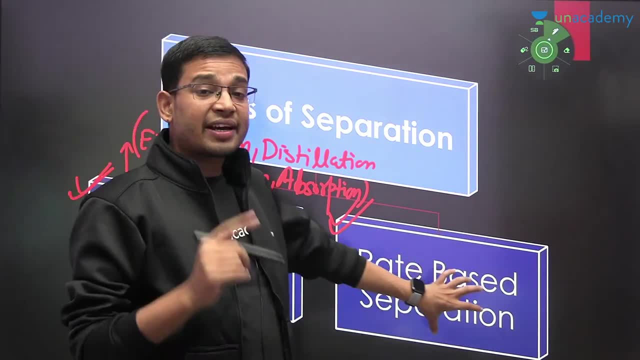 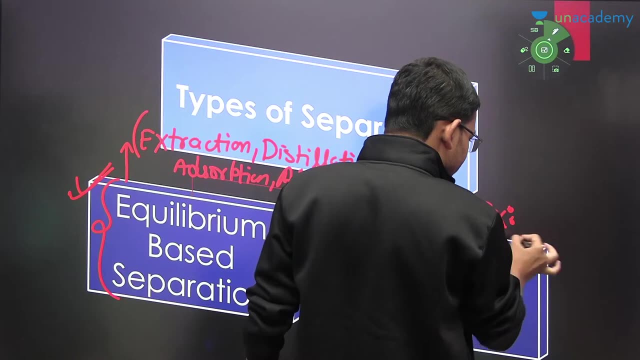 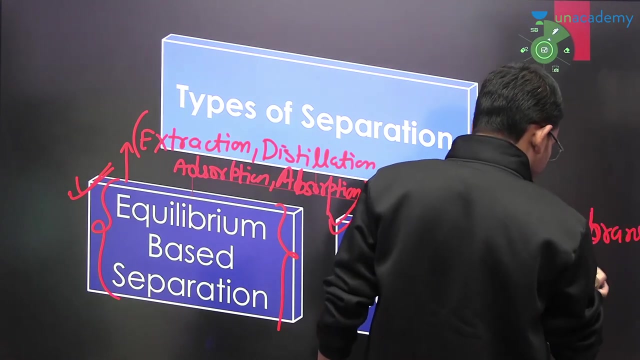 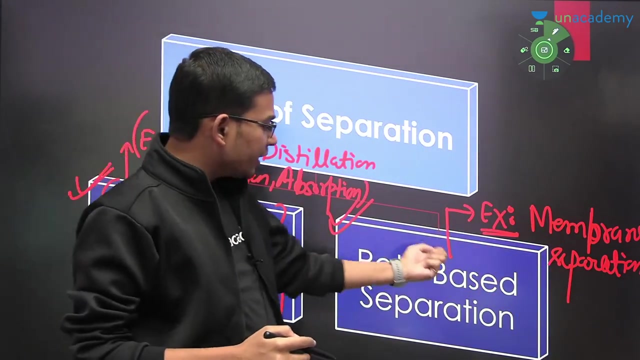 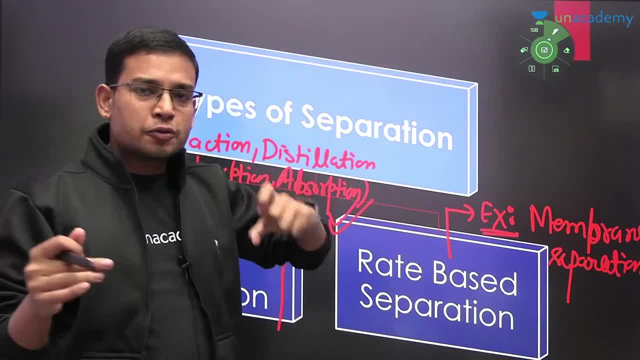 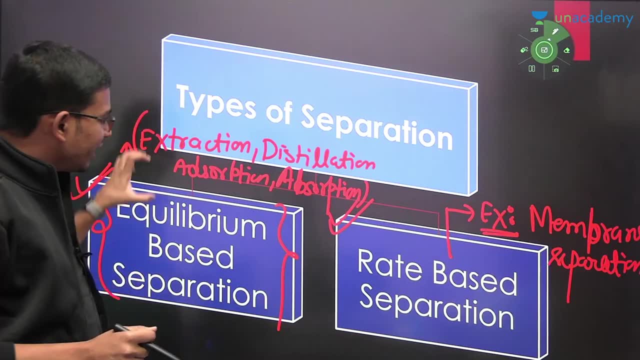 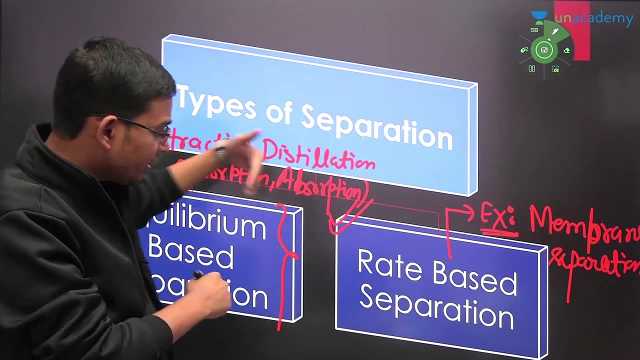 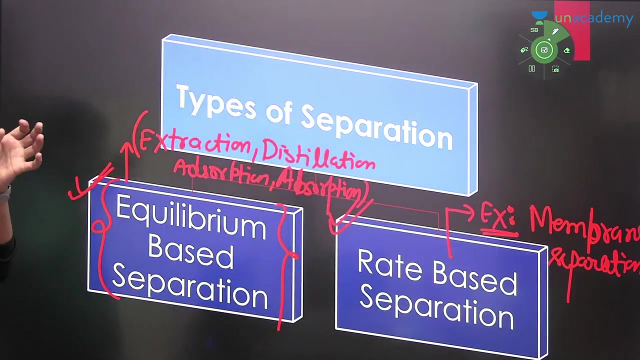 There are two types of separation. one is equilibrium waste and the other is rate waste. Membrane separation is Rate waste separation. Equilibrium separation is the separation of Extraction, Distillation, Absorption and Adsorption. Now we will talk about Membrane separation. Now let's start. 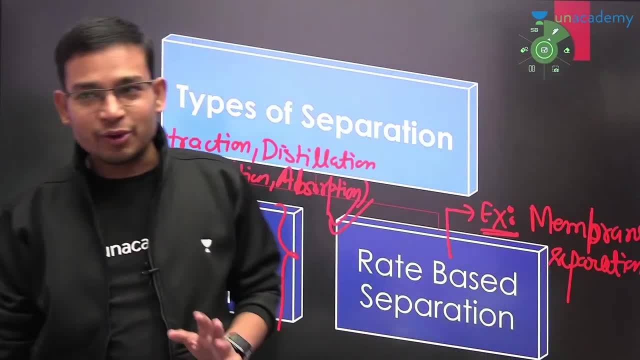 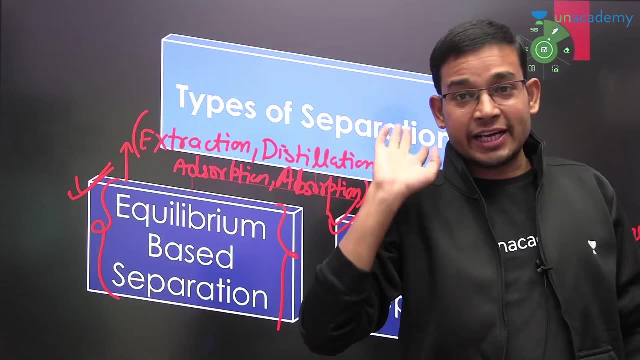 Please slow down a little bit. No, no, no, no. You will have to catch things now. it is not that the time is slow and then it will not end. Membrane separation will last for 10 days. You will have to manage it a little bit. things will be fast. 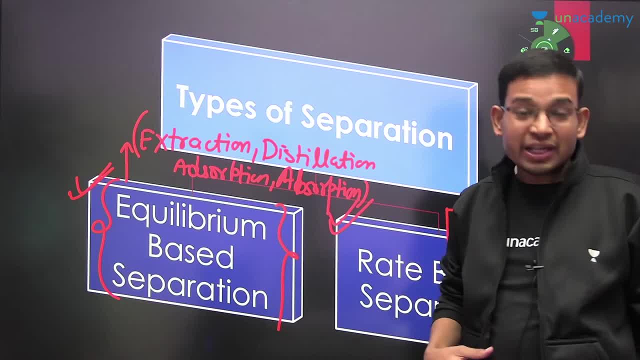 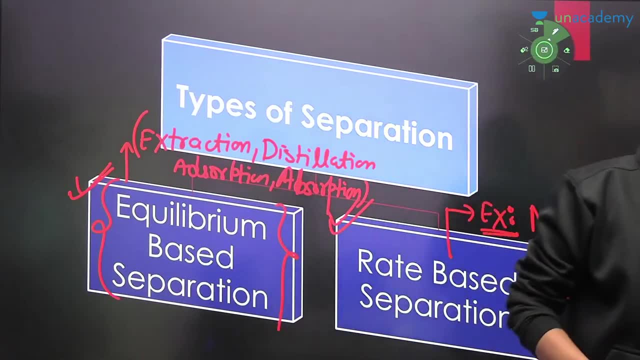 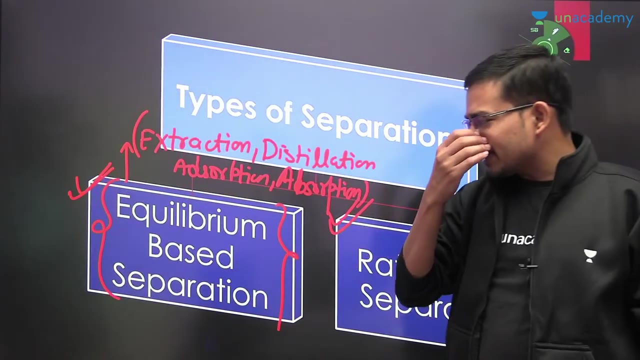 Is Membrane separation used for high temperature? No, We do not use it for high temperature. we generally work on low temperature. What is Membrane separation? It is clear that there is nothing in it. it is very simple. There must be no problem here. we have talked about the basics so far. 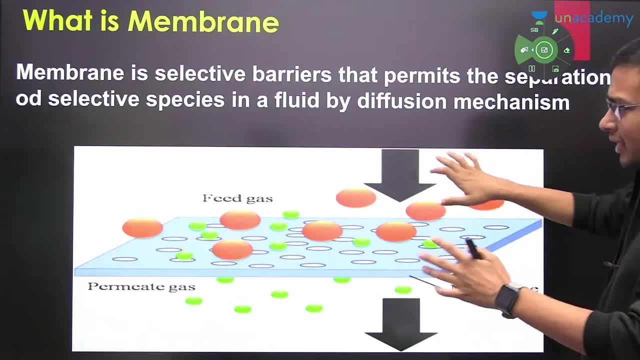 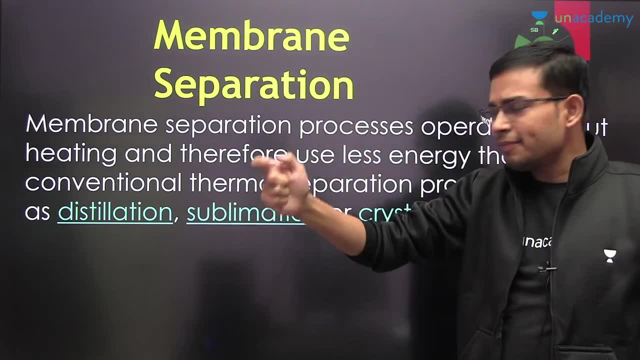 Let me just recall what we have talked about till now: Membrane is a barrier. what is Membrane separation? Membrane separation is also one type of separation in which heat and more energy is not involved. There will be separation here too, but without heat effect. 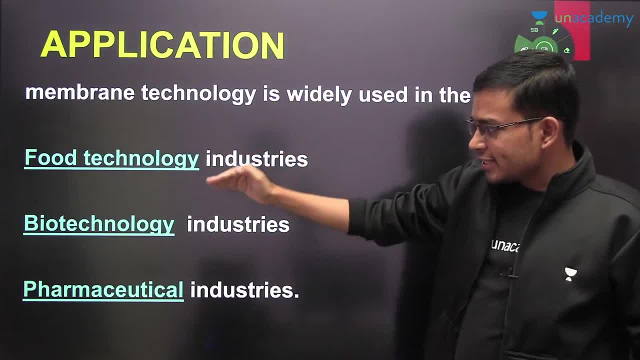 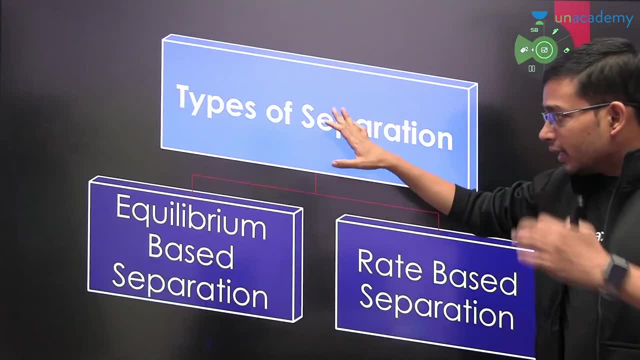 So you saw, from here, just see the application: Food industry, biotech and fire. From here, just Forma, biotech and food. You have seen its application in these three places. Types of the separation: one is equilibrium and the other is rate waste. 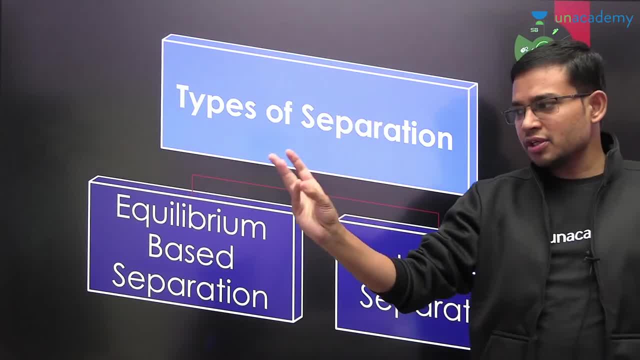 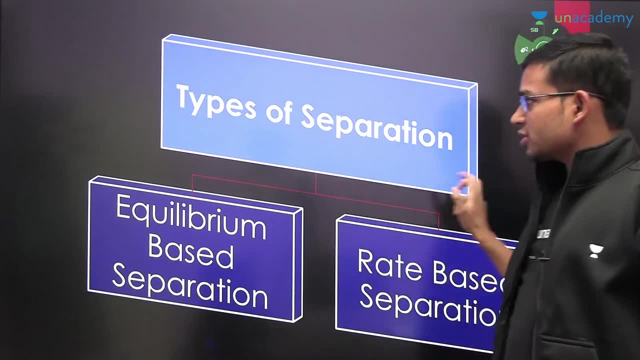 Equilibrium separation you will have to read, Like extraction, absorption and distillation. What was your equilibrium? waste Rate, waste separation: you will have to read The example of which I have told you, that is, Membrane separation. Now come to the next point. What is the drawback of it? 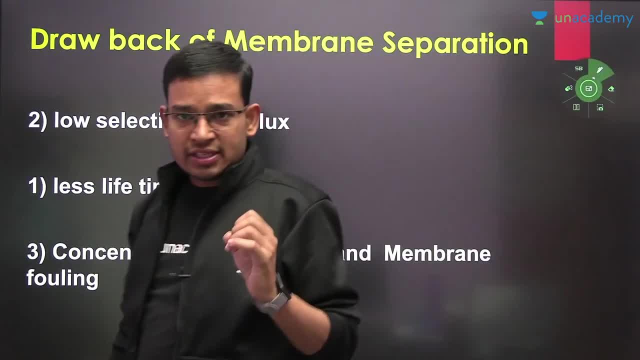 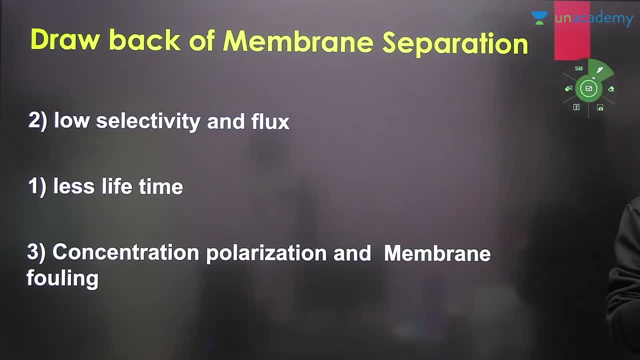 I will be involved in the theory part. What is the drawback of Membrane separation? This question can be asked in the interview, Sir, what is the drawback of the Membrane separation? What can be the drawback of Membrane separation? Okay, you are frequently using it in the industry. 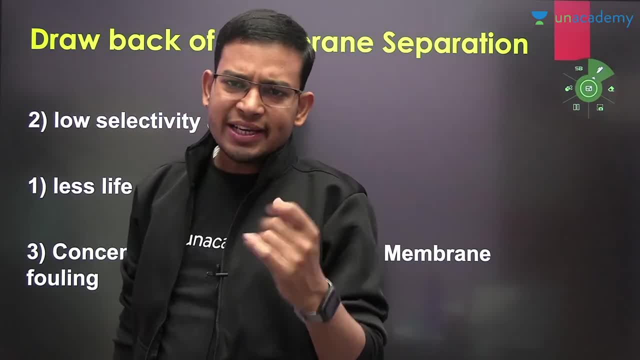 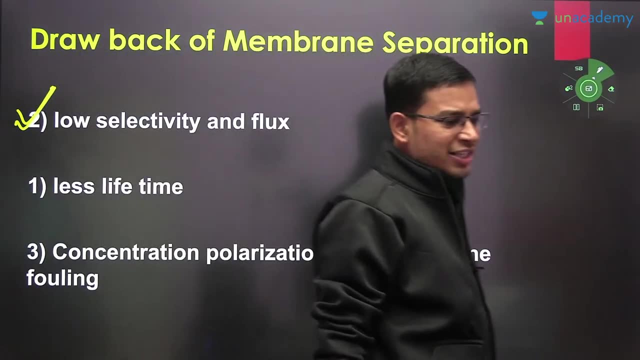 But we should know the drawbacks of it That we will not use in these places. The most important drawback is: What is this? Low selectivity and flux. Through this, you will get to see very little flux. Sir, will this PPT be shared? Yes, Akash, if you want, I will share it. 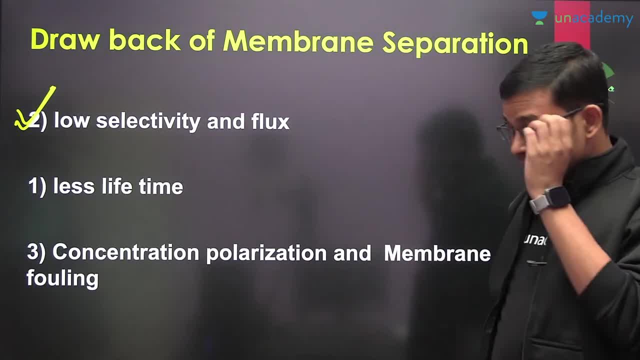 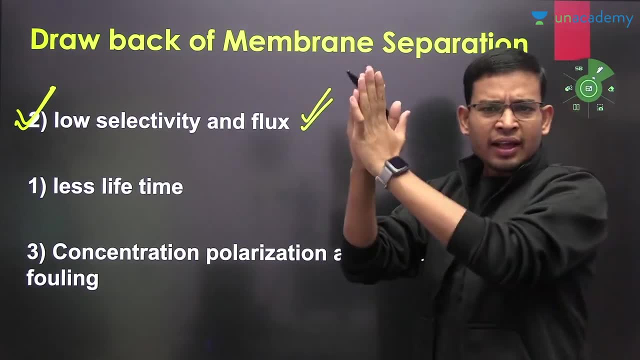 Okay, I will share it in the group, don't worry. Okay, now focus here. The major drawback of Membrane separation is You will get to see your flux very slowly. You must have seen it Like: the RO system is installed. RO is installed, right. 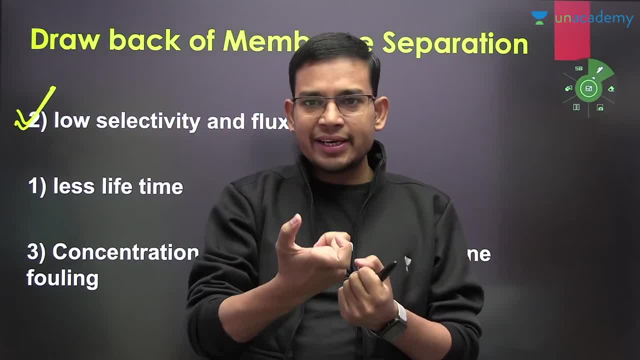 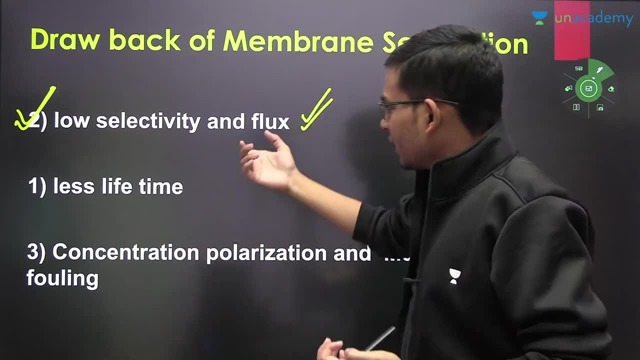 So you must have seen You take out water from RO to drink In case. I talk about a large amount of water So you can't take it out so quickly, Right? So you must have seen. You will get to see very little flux in it Because it will pass through a lot of membranes. 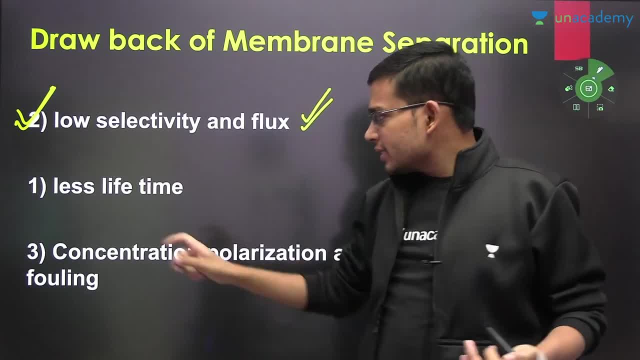 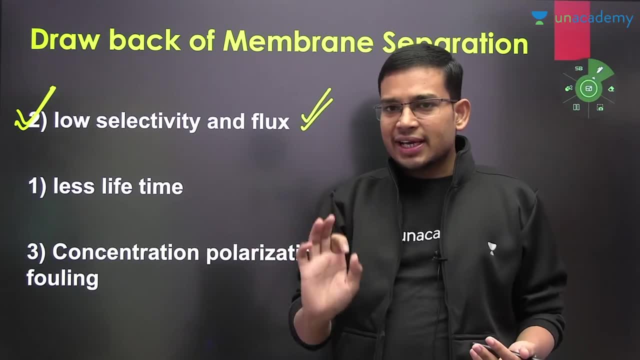 Second, You will get to see very little selectivity in it. Third, The drawback of this is Less lifetime Membrane. Its lifetime is very less Okay. It turned out to be one to one and a half years of lifetime And then you had to change. So this is one of its drawbacks. 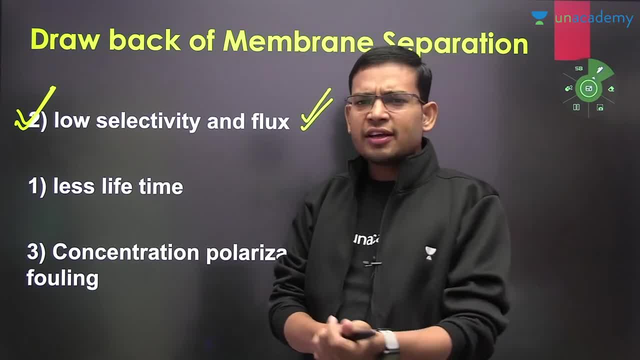 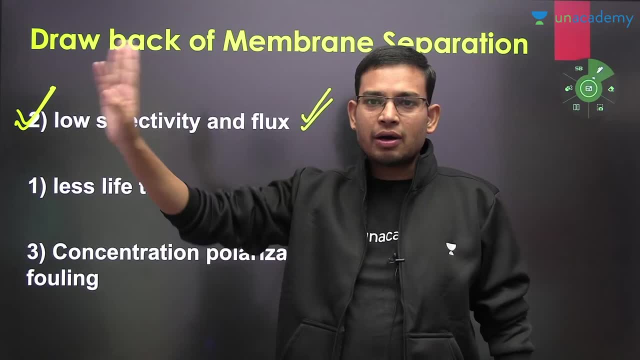 Why? Because crores etc. fall in it. So what does this mean? The better quality you take Membrane, Its lifetime is less, Like you use filters etc. So what do you want to say in a year, Brother? now this water is not coming properly. 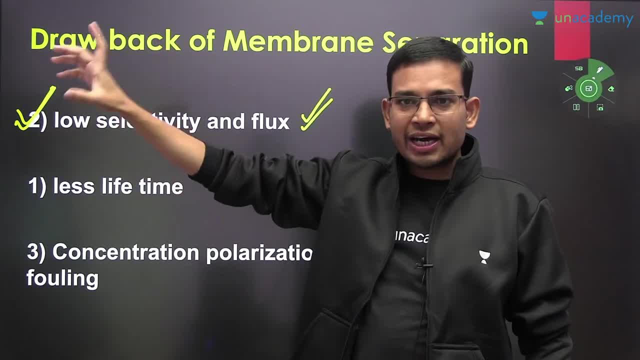 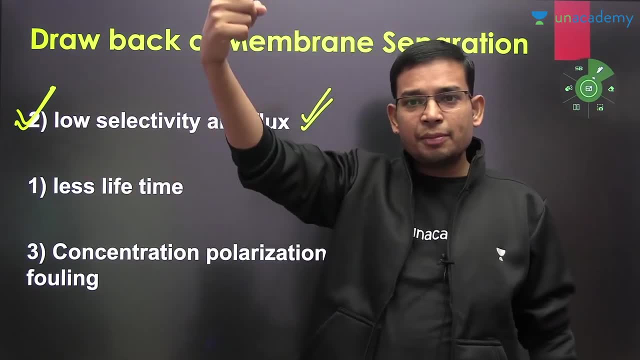 Change the filter, So this means its lifetime is less. It will not happen that once the RO was installed and it went For ten years, You must have seen something like this. Okay, So less lifetime. Now this is on a small scale, Then it is on a large scale. 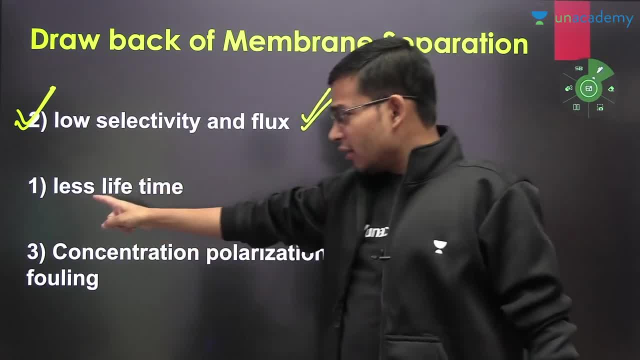 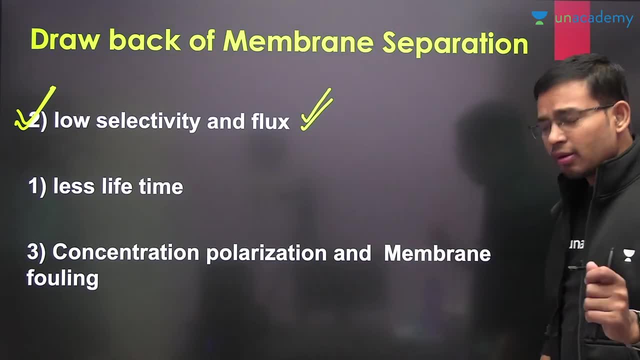 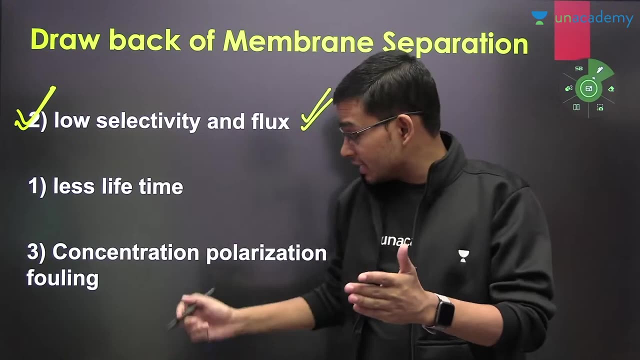 So it has to change the membrane more quickly. So this is also one type of the drawback: Less lifetime. What is its lifetime? Less, Second, Concentration polarization. Here the problem is seen a lot. What is the concentration polarization? Everyone understand the meaning. What is the concentration polarization of this term? 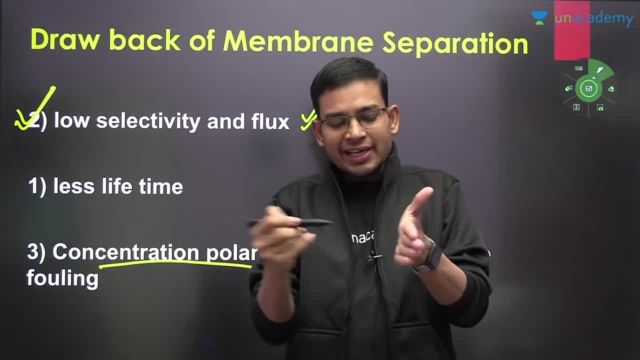 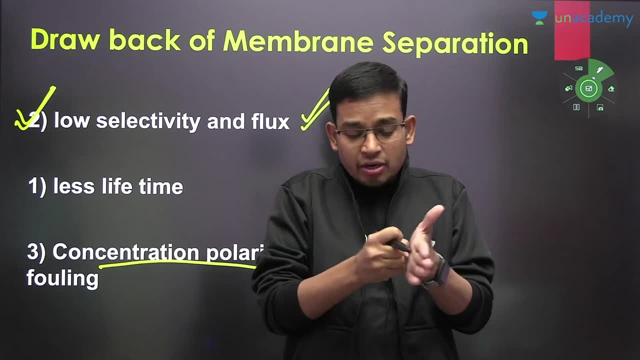 What does it mean? Means, Suppose, this is your membrane. Okay, What happened here? Deposition happened. What happened here? Deposition happened. Now, what does polarization mean? What happened? This deposition particle? Okay, It will dissolve in the feed that was coming again. So here you will see. 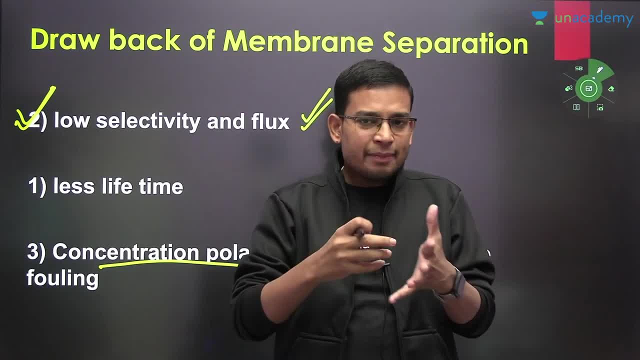 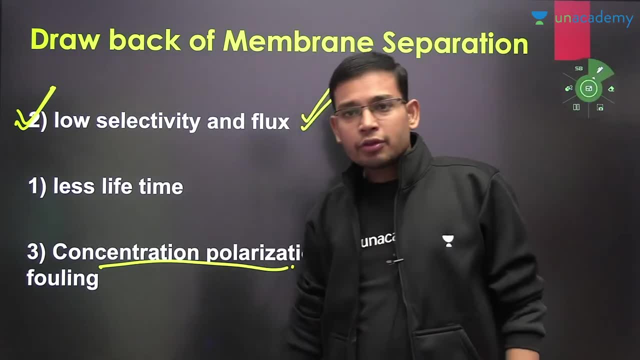 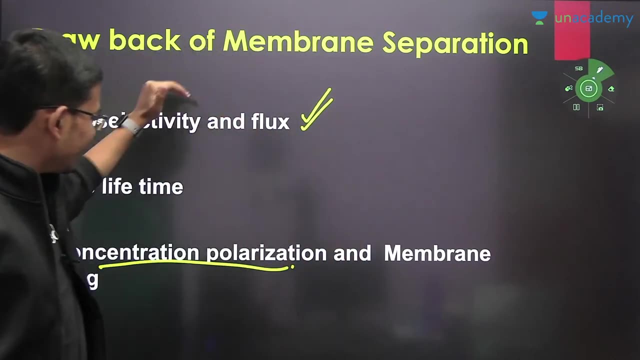 Concentration polarization- Okay. It is reversed Where your particle is reversed. So there, you will see concentration polarization, Okay. Third important thing: Membrane falling. So you will get to see one more drawback That, the membrane. There are many chances of falling, Okay. So these are three major drawbacks. 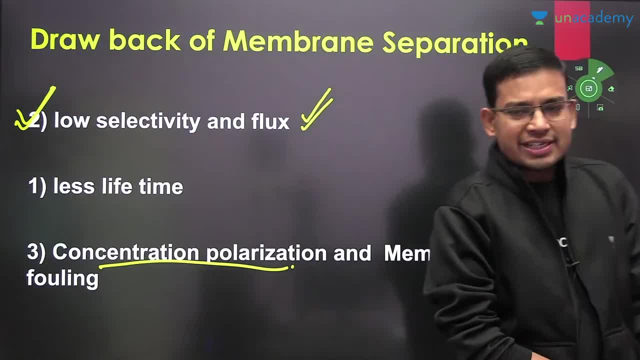 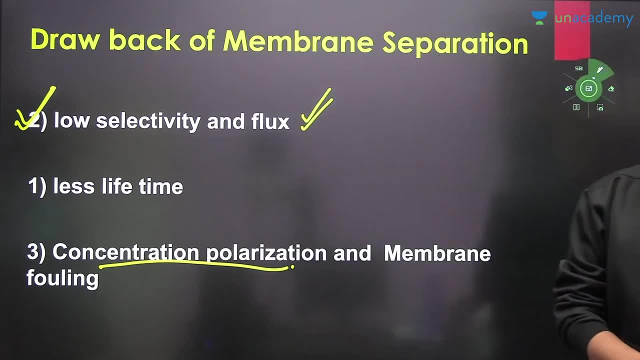 Otherwise, drawbacks. There are many small drawbacks, But in case you are ever asked in the interview, See, These three things will not come in the gate exam. But yes, You should know this As an engineer. As an engineer, You should know: Sorry, Manish, Yes, yes, Everything is going well. 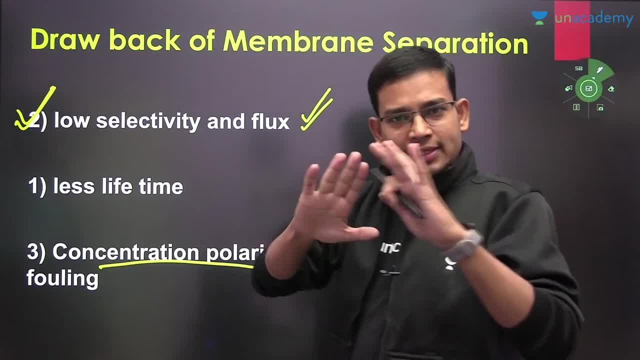 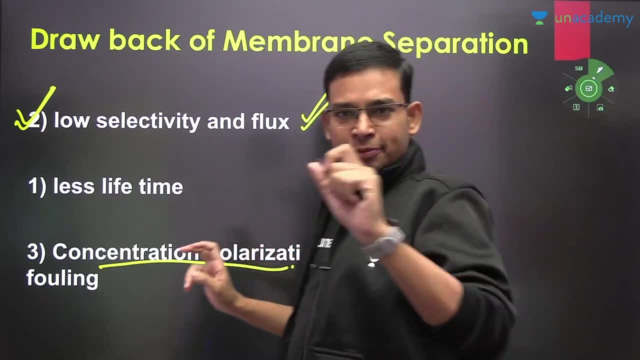 Yes, yes, Everything is fine. Till now, everyone is able to catch, Not too fast. This speed is perfect. This speed is absolutely correct. Once everyone will tell me something, This speed is absolutely perfect. Is there any problem in this speed? Anyone. No one has any problem. No one should have any problem. 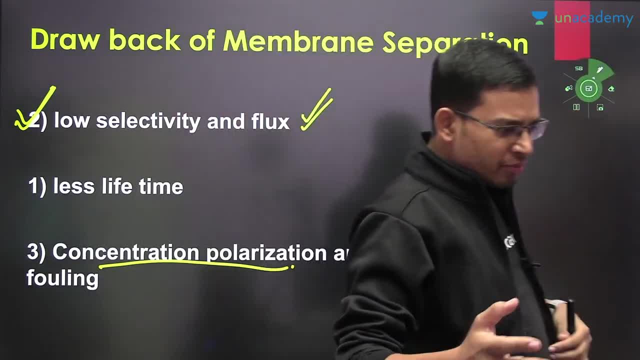 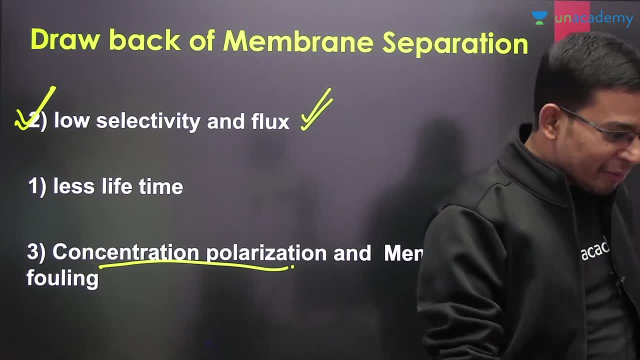 There are very basic things. You know all this. I assumed this, That I thought I knew all this, That I will tell you. I said I talk straight, Fat, Okay, You must know all this. It's fun, Great. What is membrane falling In heat exchanger? I must have read. 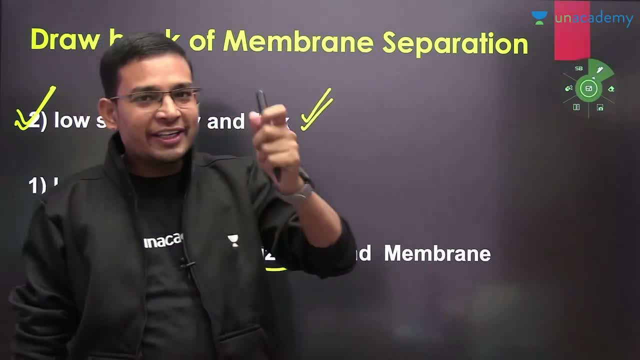 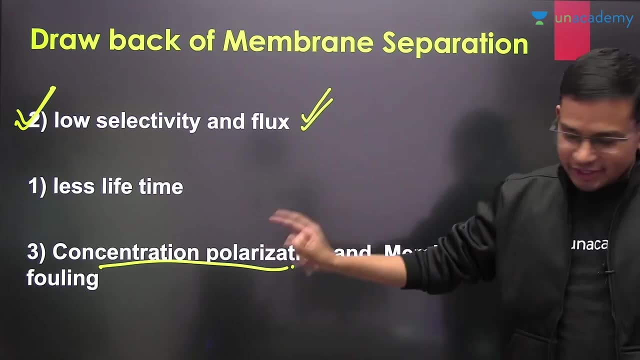 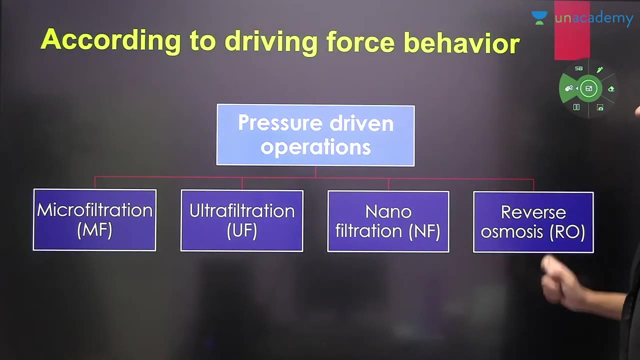 The same falling In heat exchanger. The same falling In heat exchanger. The same falling Similarly. here, Membrane falling Will be Okay, It was fun. Okay, See, now I will tell you All these terms. will go in detail, Yogis, Don't worry. Now see, According to the driving force behavior. 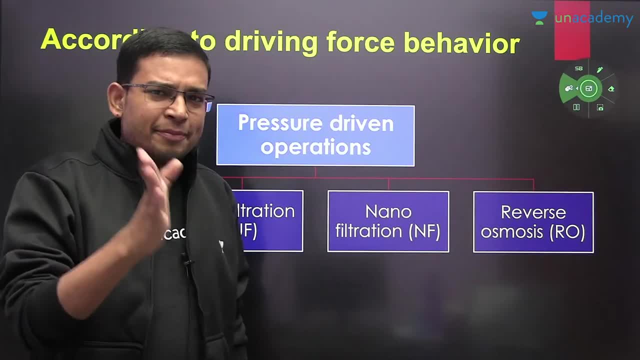 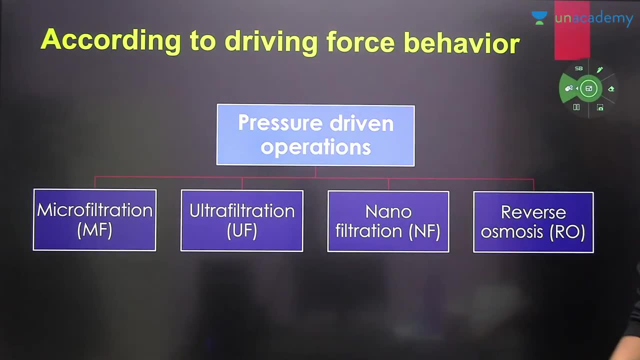 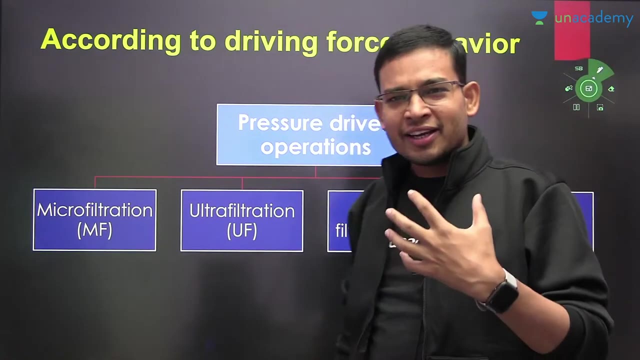 According to the behavior of the driving force. How many types of membranes are there? Okay, How many types of membranes? separation, Heating sixes, Yes, yes, Lovely, Superb, Good speed, Very good, Very good. You have to work with this. accelerate, You are young, Right, You are young. 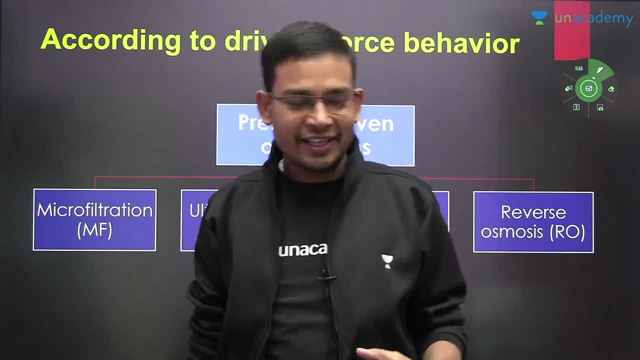 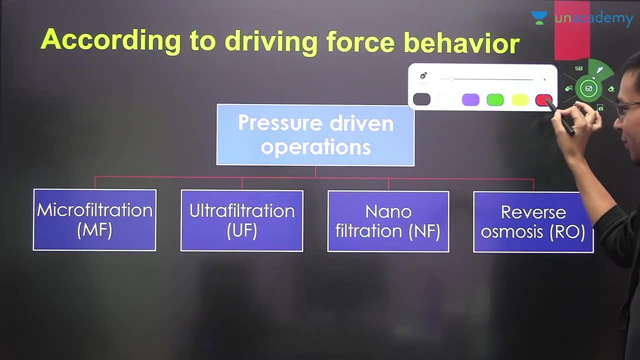 I am also young. We are within equilibrium. Okay, We will work with speed, Don't worry about that. Okay, So now I will talk from here. According to driving force Yogis, Look at your picture. I told you to wait a little. Now see The membrane separation. There you have. 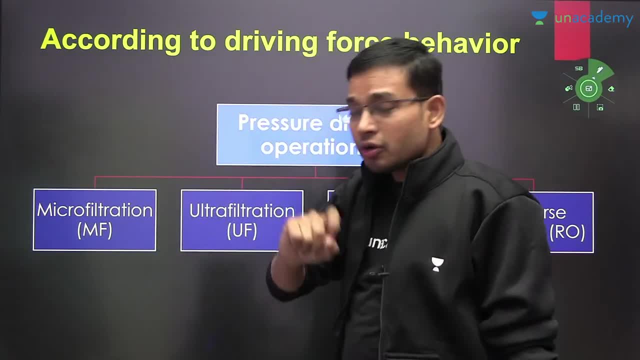 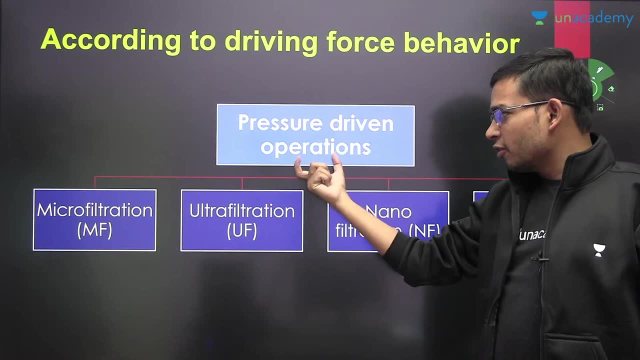 On the basis of different, different driving forces, Your separation, Not only single driving force. So somewhere You will get to see Pressure difference Drive-in means difference Right Pressure drive-in operation. So pressure drive-in operation, There is some specific filtration. Second, You will get to see Concentration. 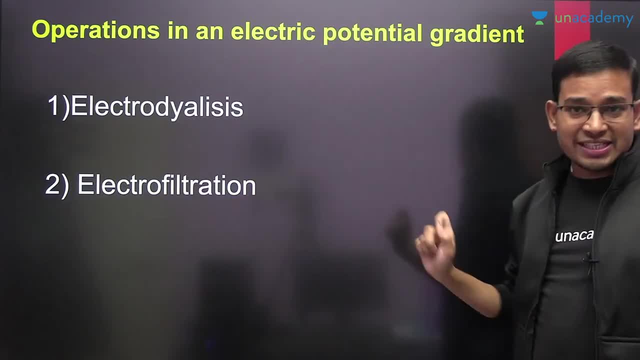 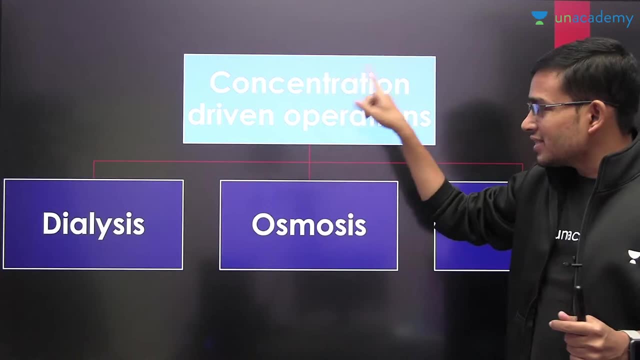 Third, You will get to see Electric potential. So from these three places, From these three places, Your membrane separation Process will be going on. So, one Electric potential, You will get to see Driving force. Second, You will get to see Concentration. And first You will get to see 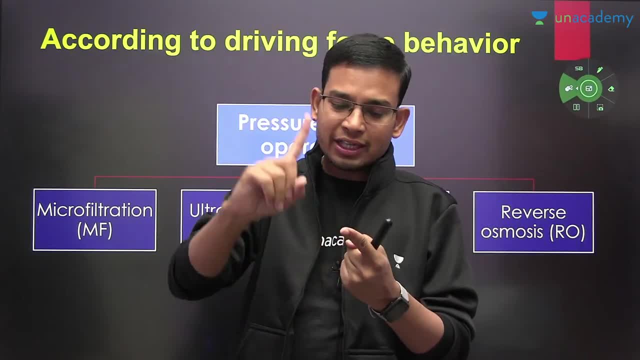 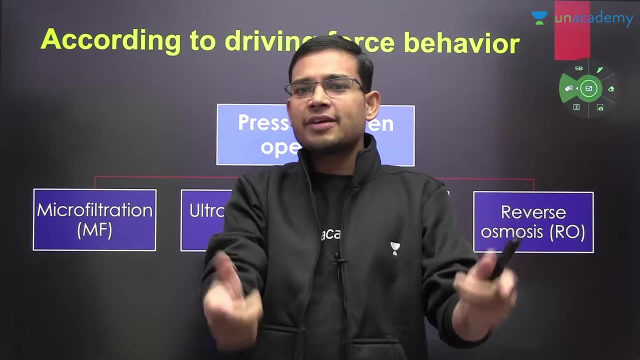 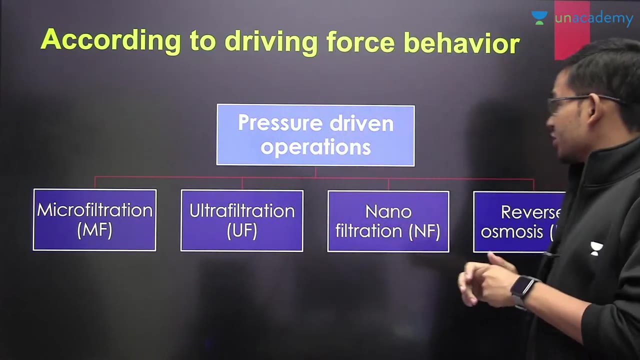 Pressure driving force. So here, How many types of driving forces Will be available? Because of pressure, Membrane separation Can happen. Second, Concentration difference Membrane separation Can happen. Third, Electric force Right, So this is the most important For your gate, That is, the Pressure drive-in operation. 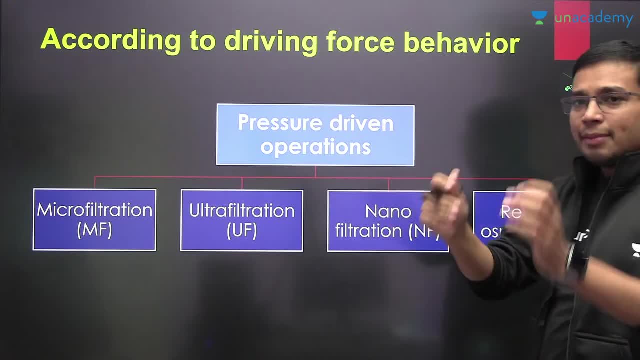 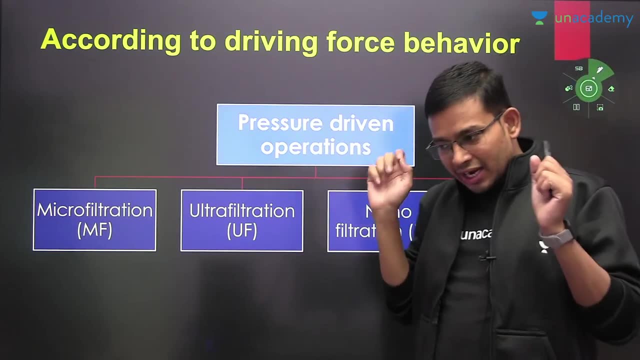 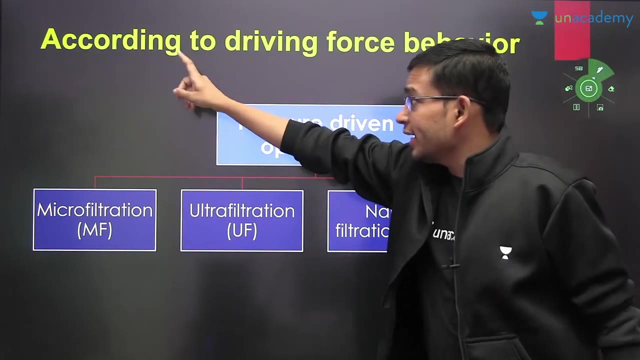 Right, That is the Pressure difference. Drive-in means Pressure difference Operation. Right Drive-in means Synonym is difference Right, So pressure driving operation. So where, Because of pressure difference, Operation will be happening, We will call it Pressure drive-in operation. So everyone will write According to the Driving force behavior. 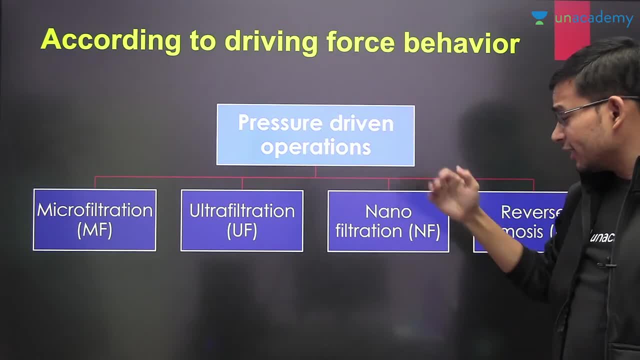 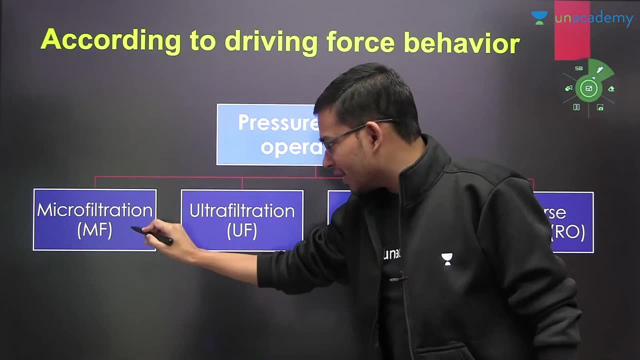 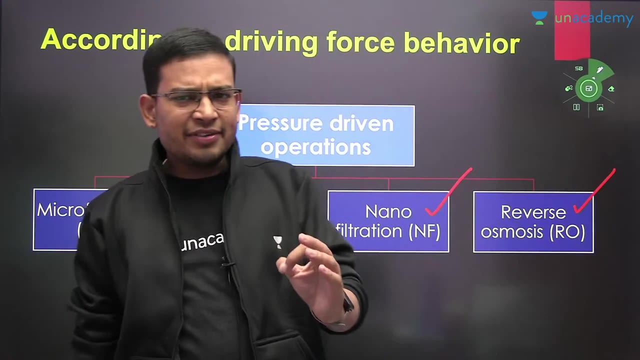 So, according to Driving force, You have Character. You have Divided into different, Different types. Before that I will talk about Pressure driving operation. So here You will see Micro filtration. Second, You have Ultra filtration. Third, You have Nano filtration. Fourth, You have Reverse osmosis. Okay, There is one preparation. 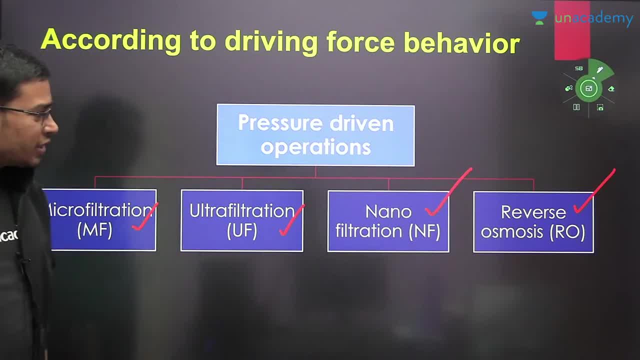 But it is not of that work. These are four of your work. Four of your work. Fan of MRN Dead. Very good, Yes, So everyone will write Where Pressure difference Driving force Will be available. You will get to see Pressure difference Driving force Similarly here In these four operations. 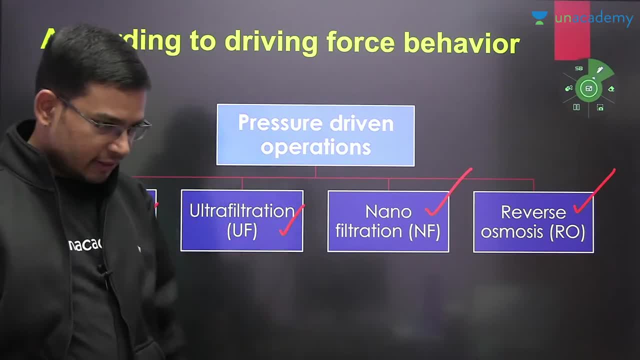 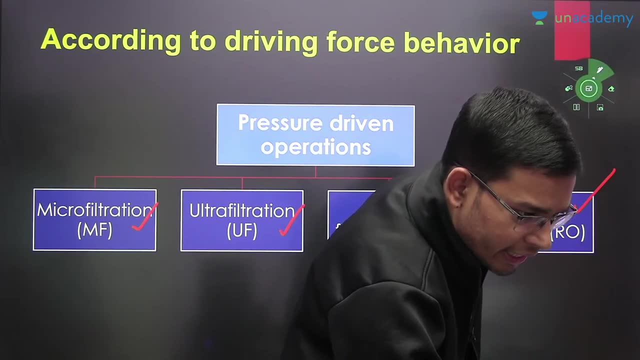 You will get to see Driving force. That is the Pressure difference. Okay, Now let's talk about 1 by 1. What is this? What is this? What is this Right? What is this? I will talk about Here. I will talk about What is Micro filtration, What is the? 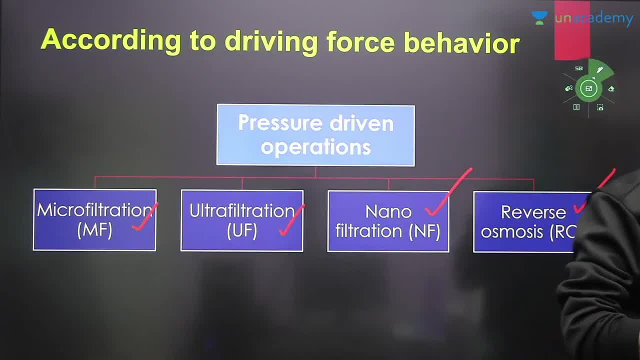 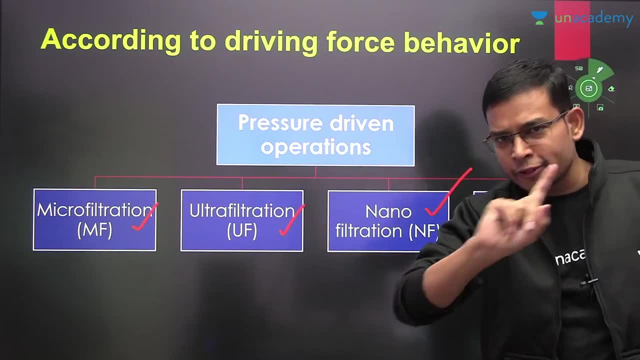 Ultra nano And reverse osmosis. What is this? I will talk about 1 by 1, Easy, Okay. So where There are three filtration, There are four filtration. Pressure difference, Driving force will be involved. That's it. That was the purpose of this slide. Now The next point. 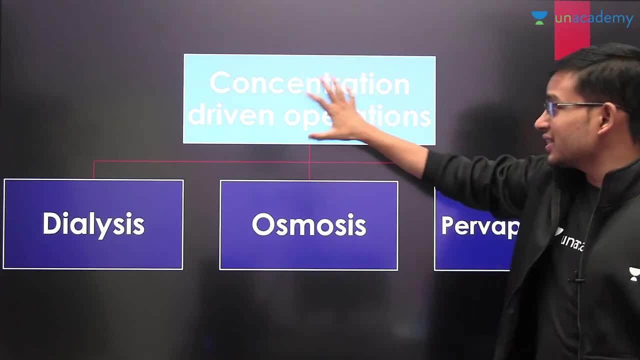 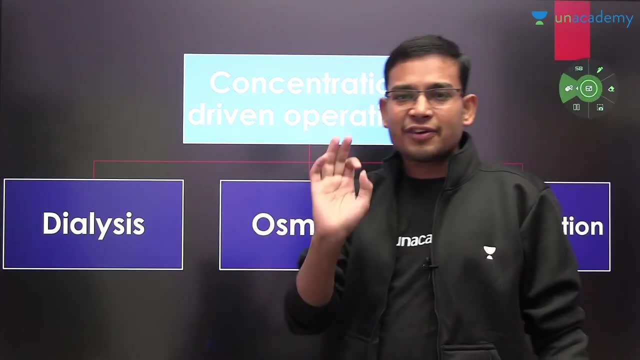 I will talk about here Concentration driving force, Where you will get to see Concentration difference. Like dialysis, There is osmosis, There is pervaporation. So here you will get to see Concentration difference. You will get to see Count, Count. One is the dialysis. 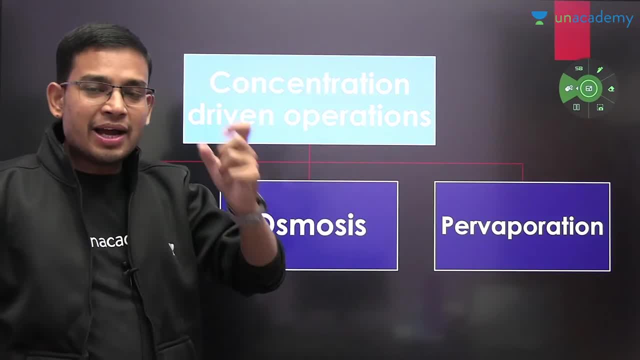 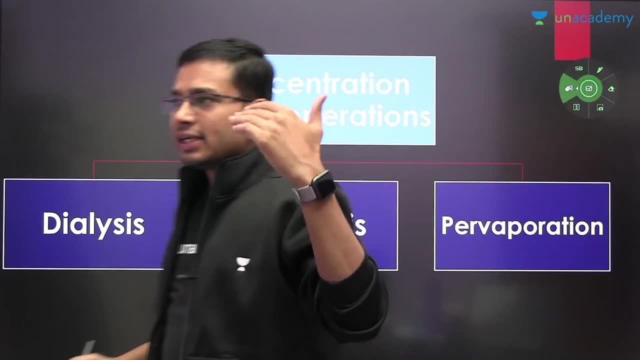 Second, osmosis, Third, pervaporation. Okay, In these operations Driving force will be involved. That is the Concentration difference Here, The driving force Which will be available, That is the Concentration difference Everyone will mention In their copy In a nice way. Everyone will write it In the copy. 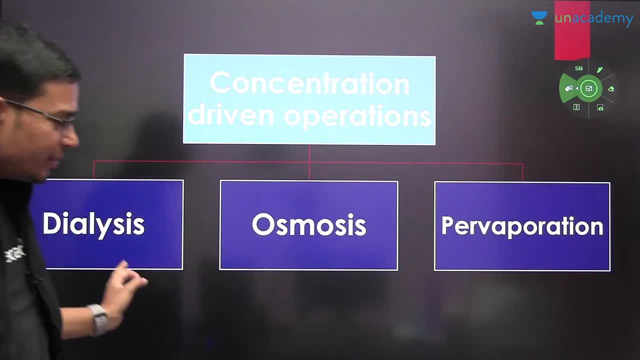 All this is useful. All this is useful. A to Z Things will be mentioned In your copy. A to Z Things will be mentioned. All of you. Now, This much is good. Till here, It is perfect, Come on. Till here, It is perfect, There is no problem. Till here. 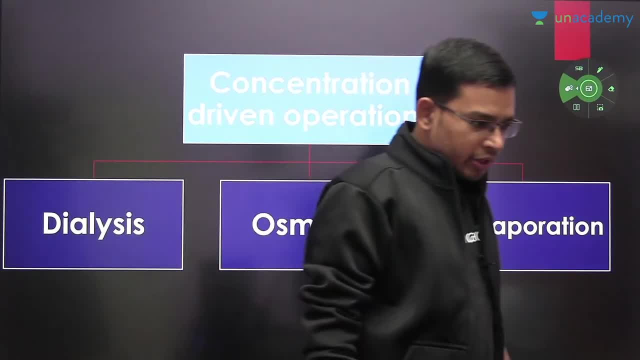 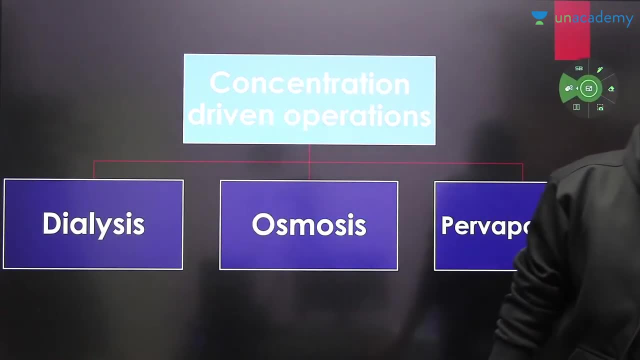 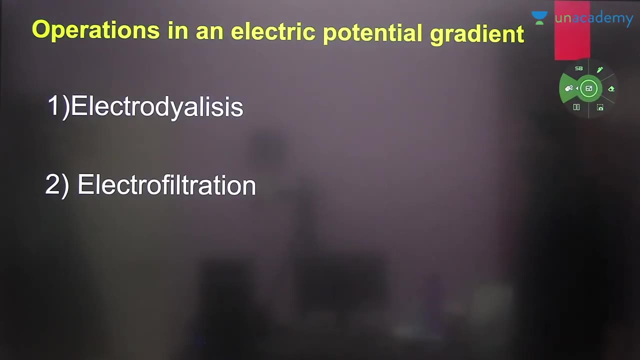 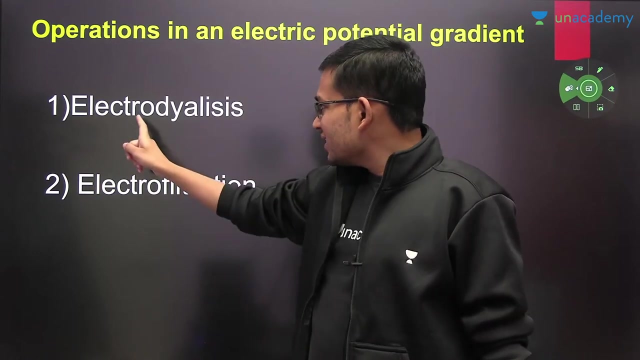 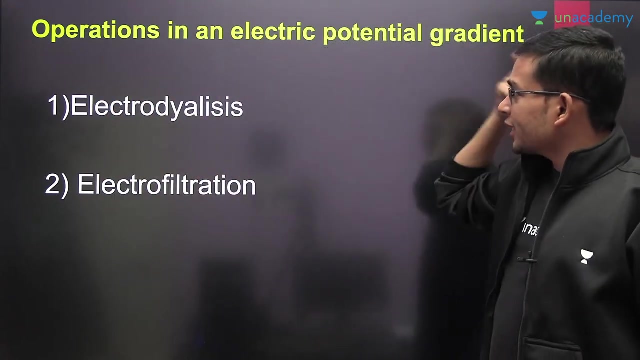 Sir. Recorded video. Sir, Sir, This video is Very much Alicia Masuka Very good. So, Sir, Thank you so much. Thank you so much For your love, Kind Chalk Bعد. Now Let me talk Third, Or 30 Monsters. There are Plenty of Project. Let me All of you, 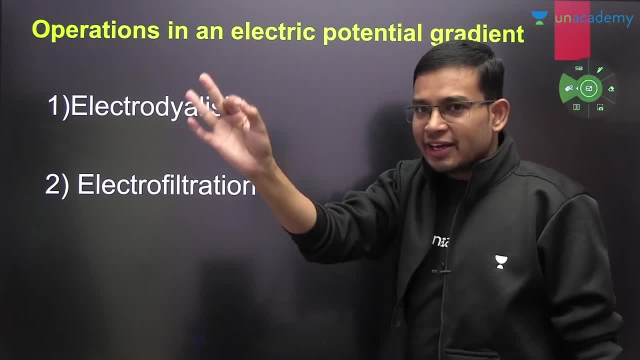 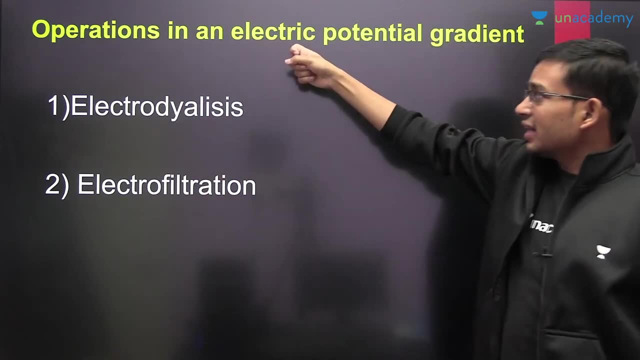 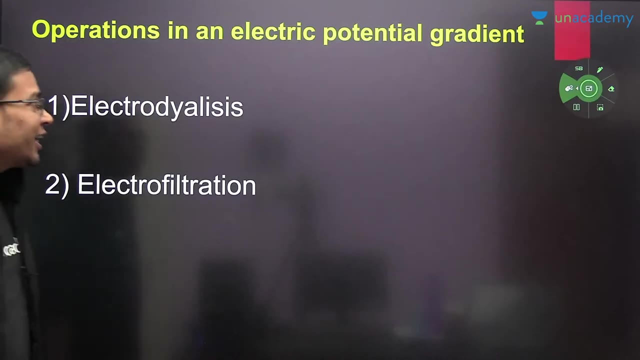 electric potential, where you will get to see driving force. one is the electro dialysis. second is the electro filtration, where these two operations will take place. your driving force will be electric potential- all of you will mention this- where your driving force will be electric potential. these are all useful things. once you should have an idea. once you 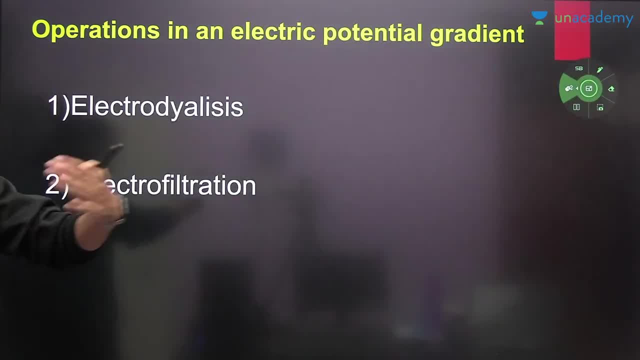 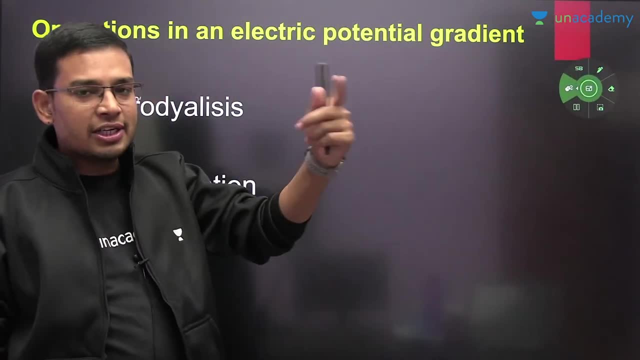 should have an idea about all these things. just now the theory part is going on. you will be involved in the mathematics part because your session is for one hour. after one hour your second session will start of mass transfer distillation. so once we cover the theory part, 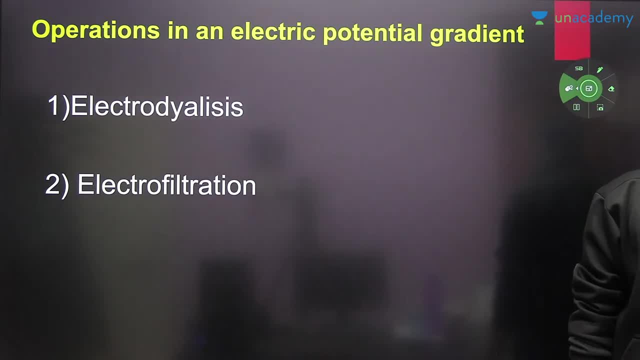 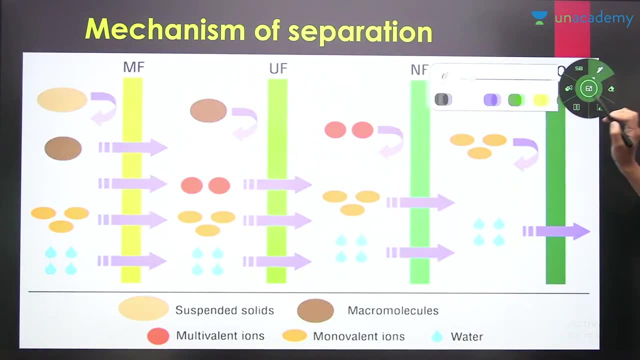 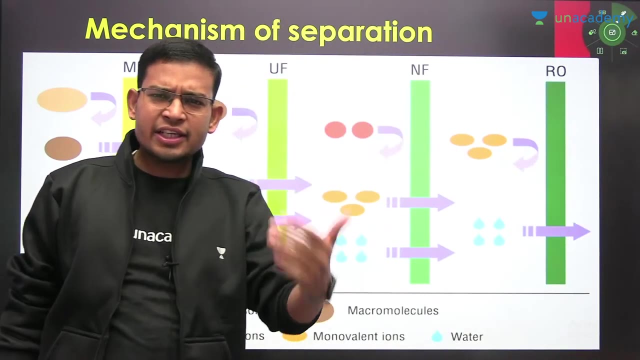 the mathematics part will be done. perfect here, we have no problem. sir, all of you will mention now mechanism of the separation. now all of you should understand a little from here. see from here where there is something to understand there you should understand. otherwise you know, I am writing the definition of ultra filtration of two pages there is. 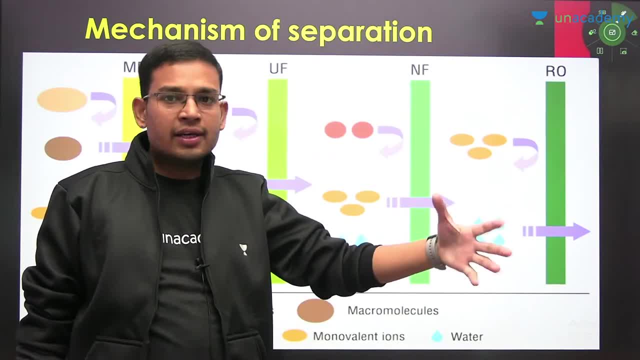 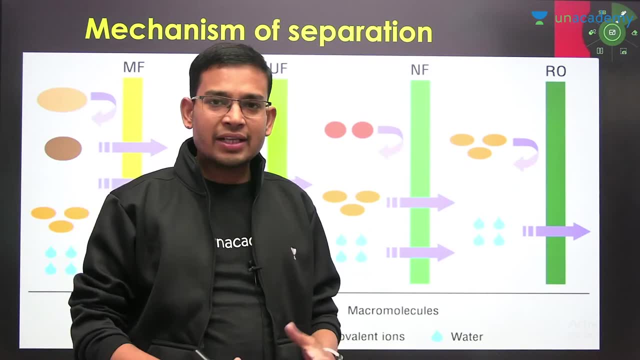 no meaning of it. understand what is the meaning of ultra filtration. if you know this much, then this much is enough, because in numerical your gate will never come. put ultra filtration heading, ultra filtration. now I am writing it for half an hour. there is no meaning of this. we have to be goat gate. 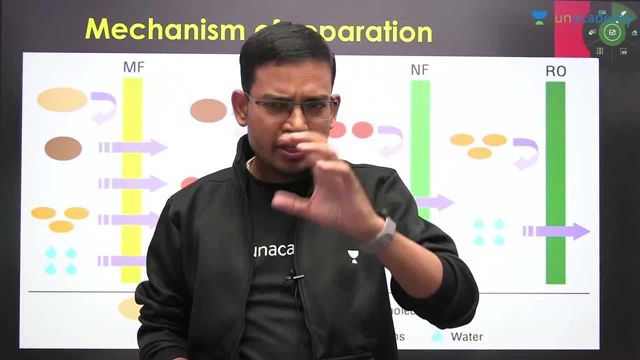 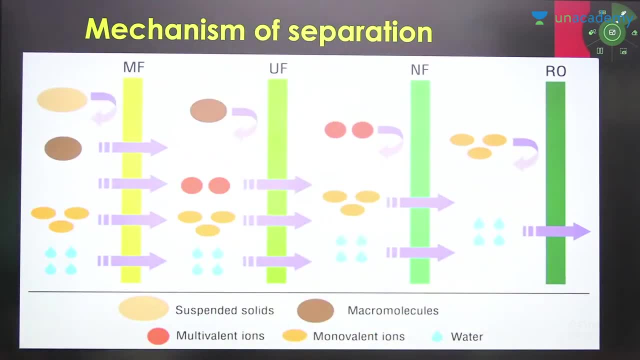 oriented. you have to think like a gate exam. theory is just to understand, write the concept and put the numericals also. so this much you have to always keep in mind. so I will talk from here. what is the mechanism of separation? what is the mechanism? so from here you have. 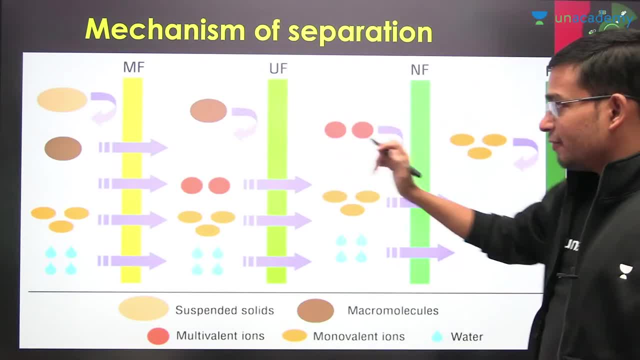 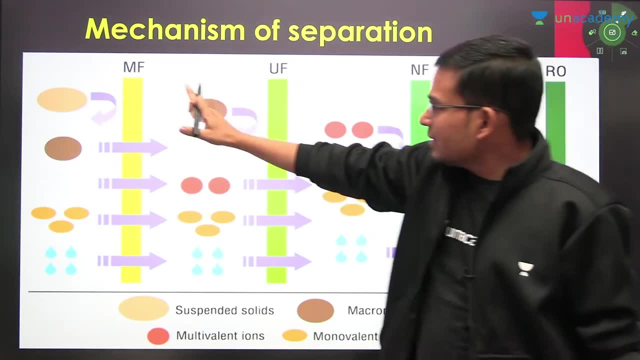 three filtration. I will tell you about the two filtration. these are the three types. then you need to listen carefully here. this is your three types of filtration. one is the micro filtration, the other ultra filtration. all of you are visible. all of you. you need to see the figure. one is the micro. second, ultra nano and arrow. all of you, this is visible. 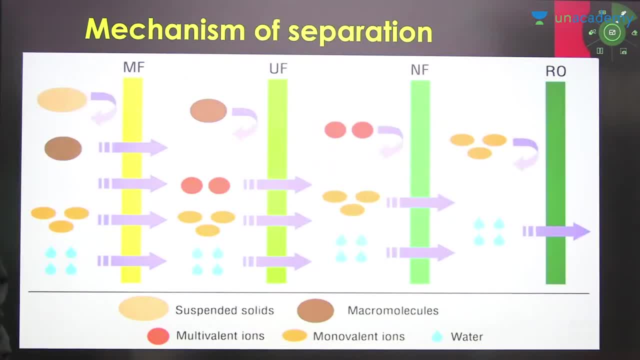 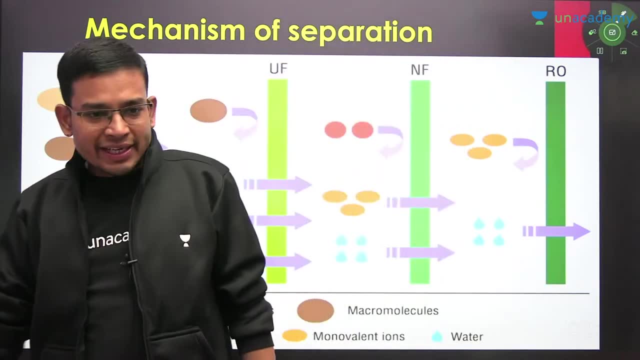 we will see. one time it is visible, right, completely, i will talk. only then i can talk, brother. what is the mechanism? how will this separation will be done. understand all of you. it is visible, then only i can talk, brother, man, sir, then only i can talk. but what is the? 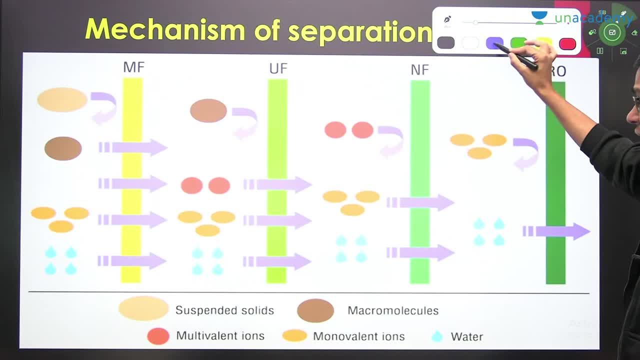 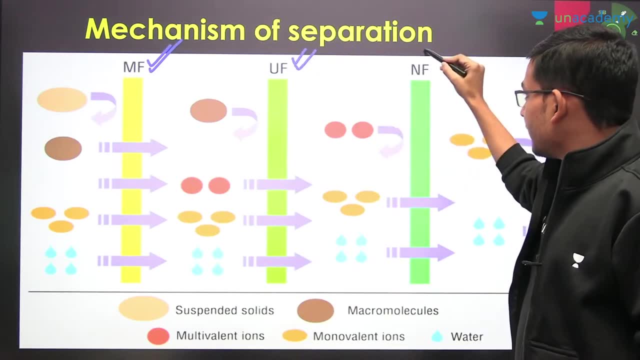 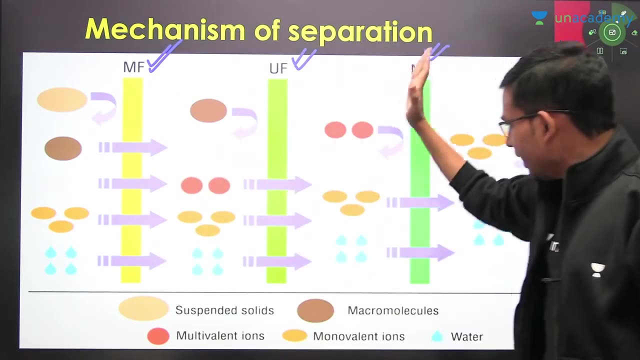 good sup. now I may also just walk around the group. you have some about Karuna. yes, after I, micro filtration. this is the micro filtration, because this is the ultra filtration. this is the nano filtration, this is the arrow. reverse osmosis up there, can I happen? yeah, filter media. yeah, filter media, yeah. 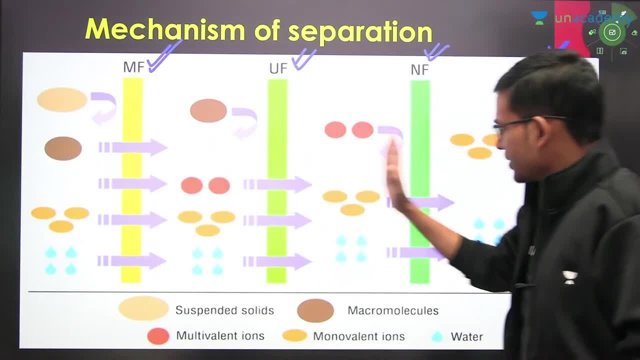 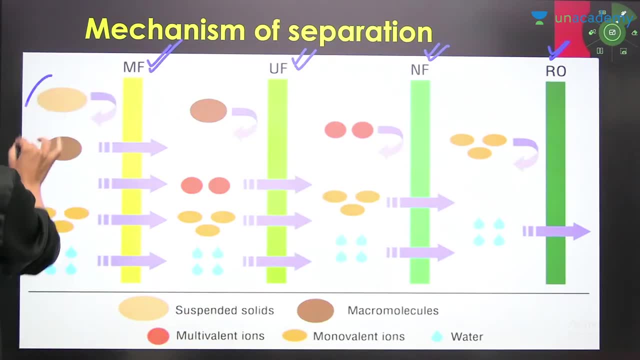 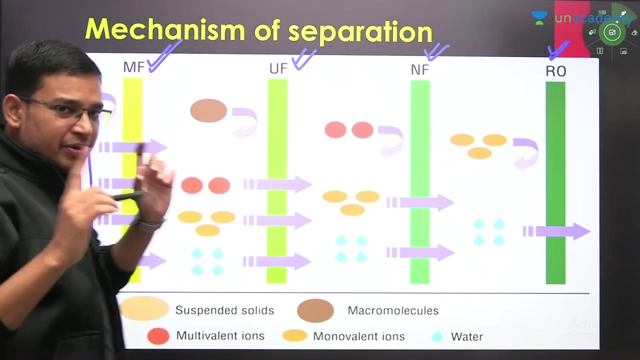 filter media. filter media means this is the membrane, this is the membrane. okay, okay, now up there upon casual feed away. this is the our feed, this is the our feed. both the answer? they cannot. if, Nick, I have roofie of a feed, same catch at the end pure water of feed. see catch at the key: Amara, pure water, nickel key I. 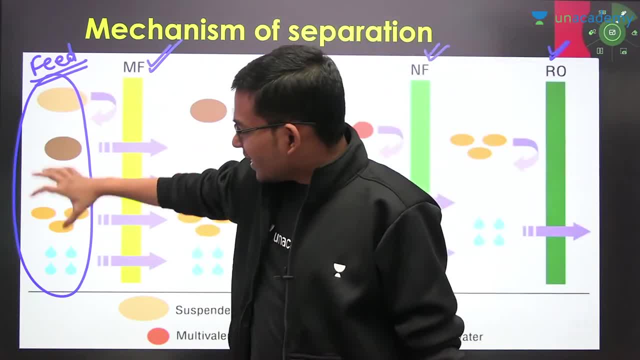 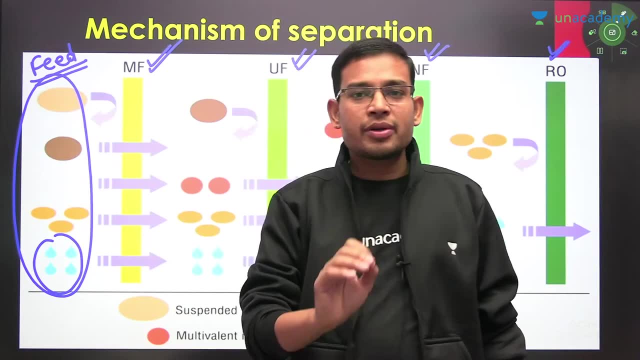 we want. I'm looking at a key to my feed, a yeah, see upon a jury. a panier jelly given a each other. take a year to panier. it's kinder jittery. we a particle in co-sup com. remove Karanach at me so that. 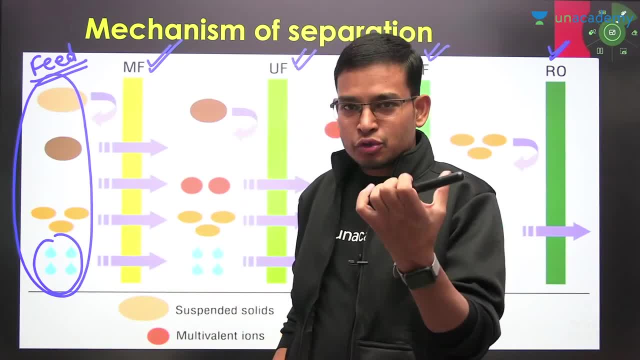 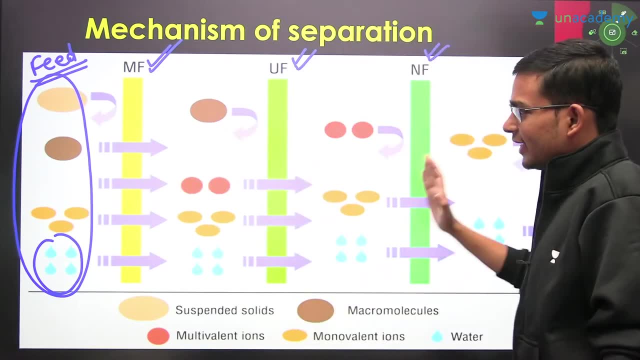 I'm a repass kyao day page on means: up to suit the gel or a boab come in, yeah, so yeah, I'm chatting so up: cases separation, carrying it so up, carrying a different, different top filter media, like I. need a different, different top membrane, like I. 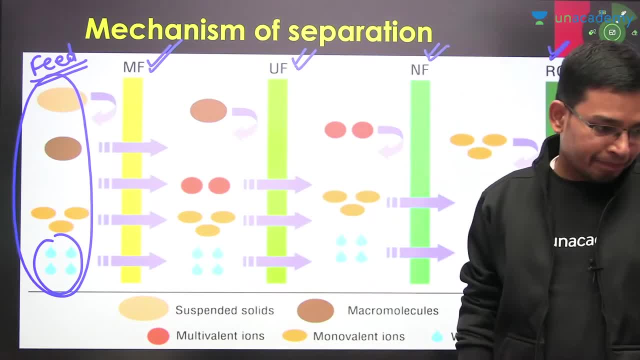 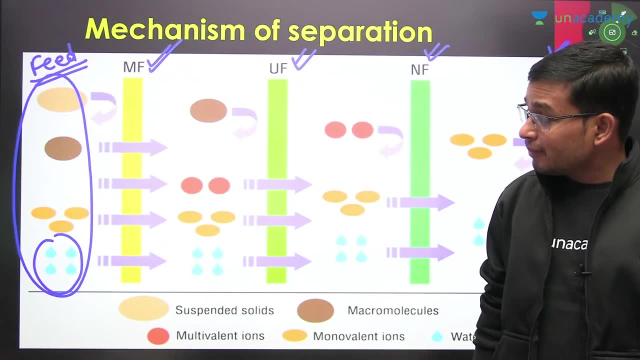 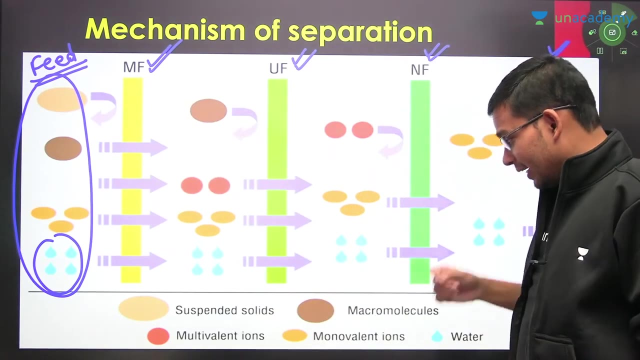 need a up a la la membrane ka la la come a heap a summer. no, take a both the answer. they cannot. both the answer. they cannot. a la la la me, a la la la membrane ka la la come a. this is the micro filtration up here. up is our look. they cannot do up a micro filtration, hey. 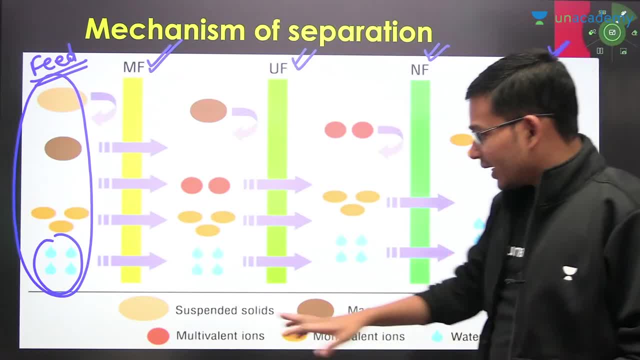 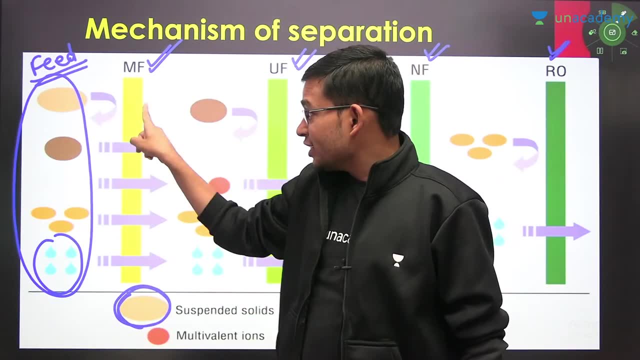 book can particle core location in particle core. ok, right, this is a suspended particle, Joe, micro filtration. they book can call your즈abrowska. here you have a bigger wake processes to past me on a Youron Joan. suspended particles on gay. okay, Joe, butter, butter particles on the anti spinning. 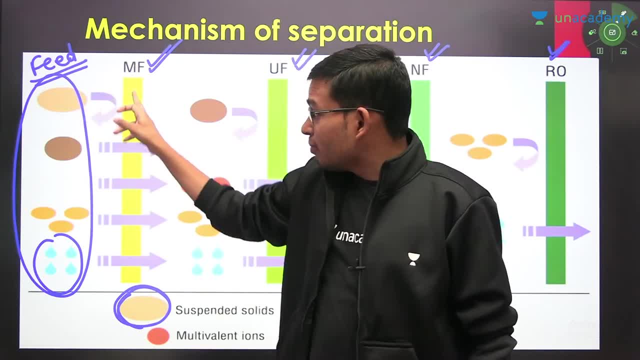 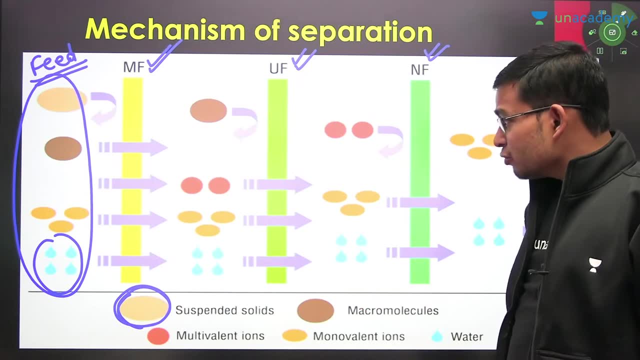 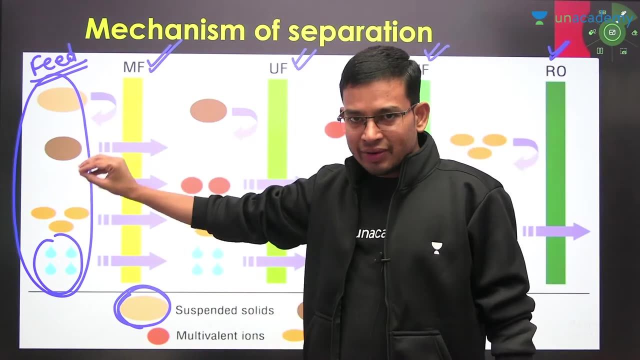 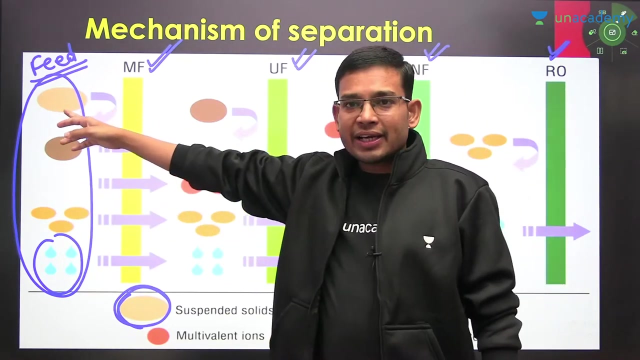 suspended right. Joe, suspended particle. no, scromedic, Ruth is very powerful micro molecules and this is your multivalent ions, monovalent ions, and water in this, your multivalent, monovalent micro component and your water will pass all this, but what will you do? this? 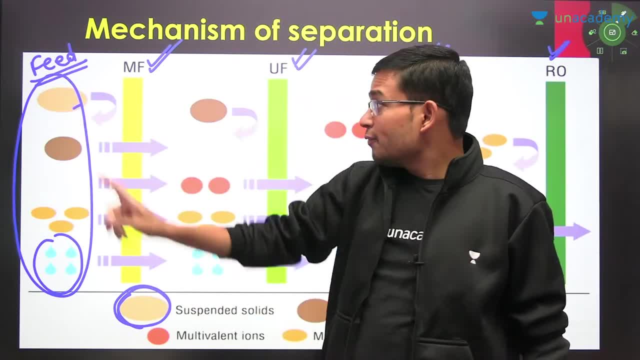 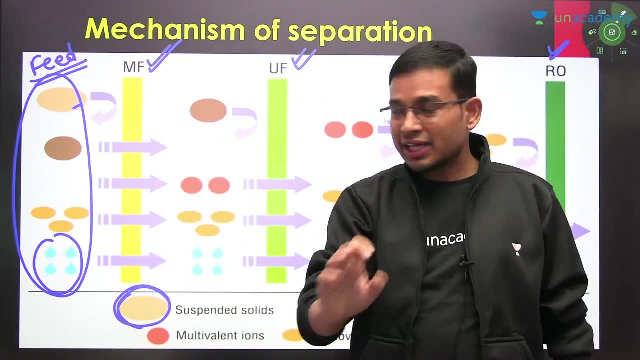 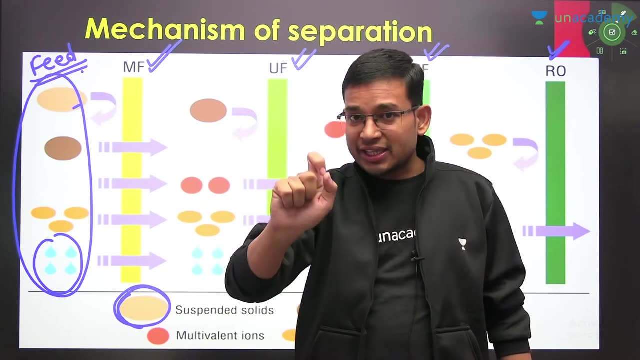 suspended solid will stop it. this is the purpose of microfiltration. that's it. this is the purpose of microfiltration. what is the purpose of microfiltration? that is to stop your suspended solids. stop them. ok, it does not let them pass. so this means this means there will be more. 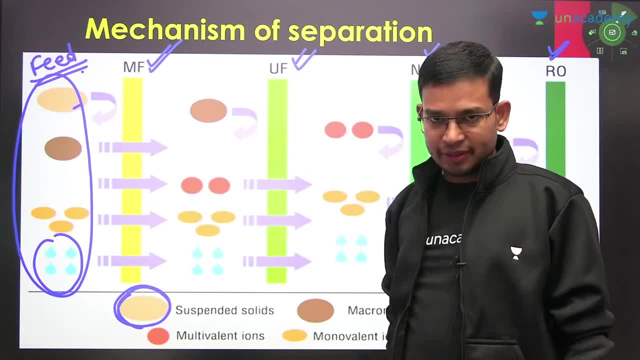 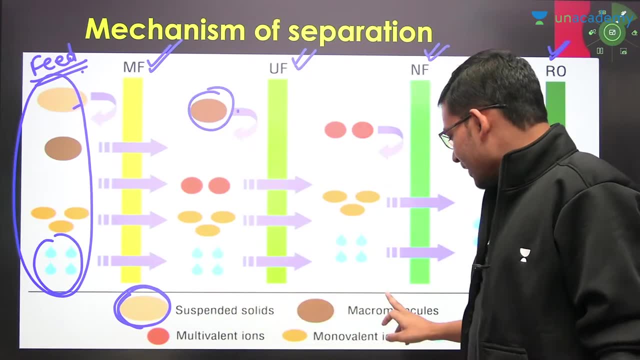 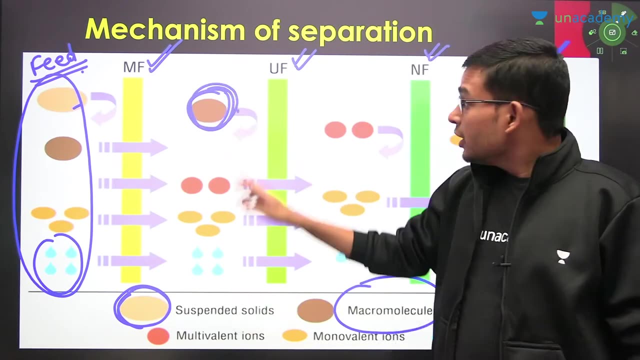 pore size than this. now see. now I come to ultrafiltration. what is the work of ultrafiltration? what will ultrafiltration do? what is this? what is this? what is this? your micro macromolecules? the macromolecules it stopped it. what did it do? the macromolecules it stopped it. who? 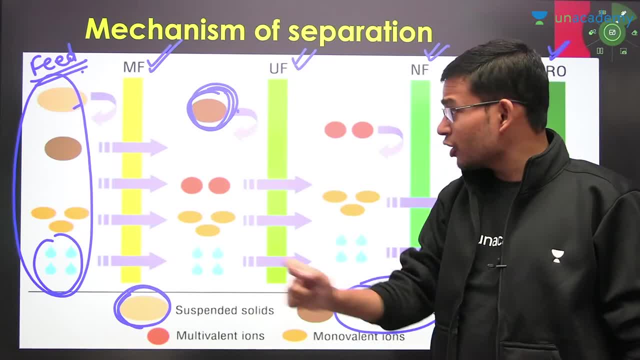 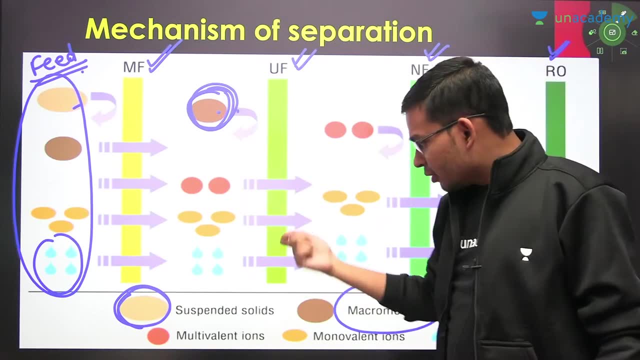 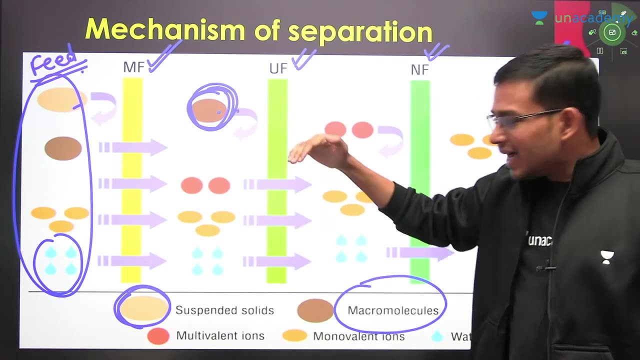 did ultrafiltration. when there will be ultrafiltration, then the macromolecules will stop here. what will be passed? your ions will pass, ok, your multivalent ions will pass, your monovalent ions will pass and your water will pass means ions will stop, right, ions will stop in ultrafiltration. now. 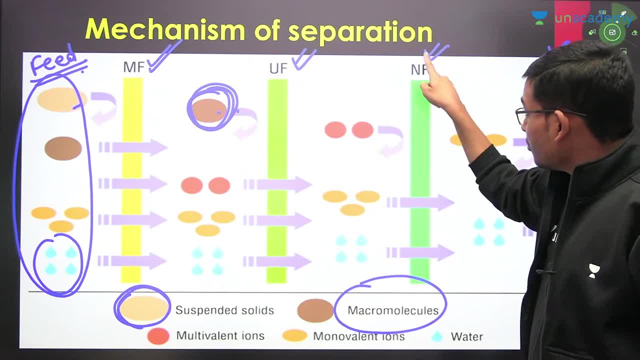 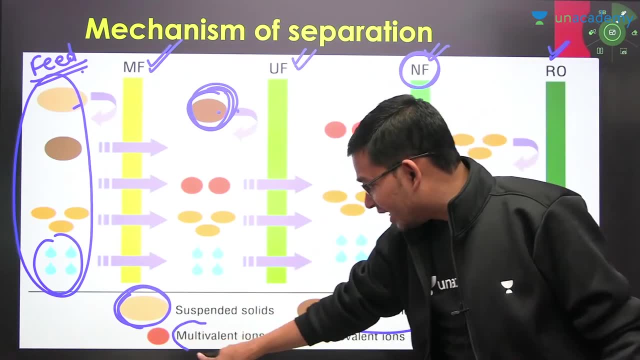 I will talk now. I will talk about nanofiltration. look carefully at nanofiltration. what will happen in nanofiltration? what will happen in nanofiltration? the macromolecules will stop. what will happen in nanofiltration? what will happen in product rotation? what will happen? 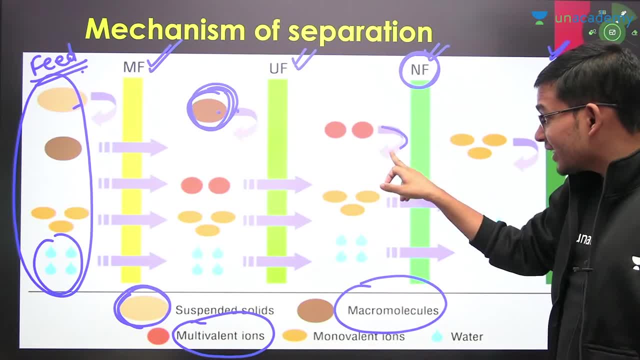 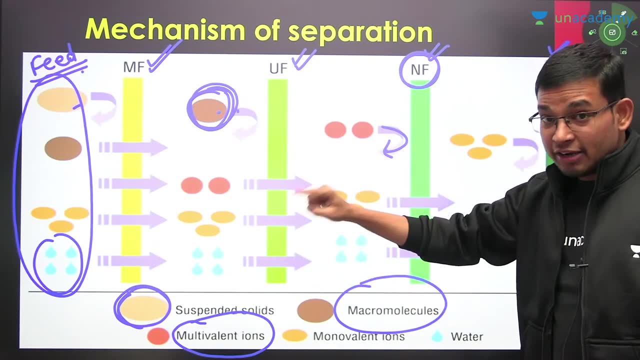 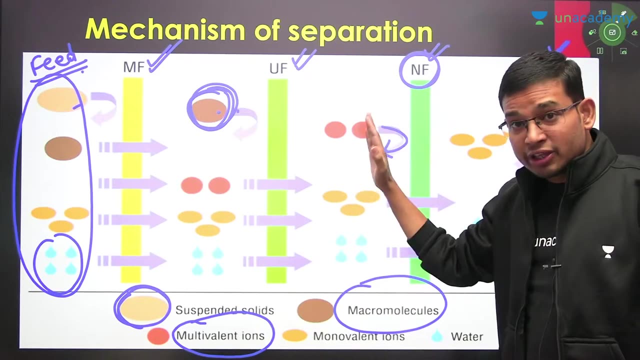 in product rotation. what will happen in product rotation. what will happen? what will happen in product rotation? what will happen in product rotation? your majority of ions are Respon to any icon policies that you have between neurons does not matter. the macromolecules will stop the unteroPower eurozone. 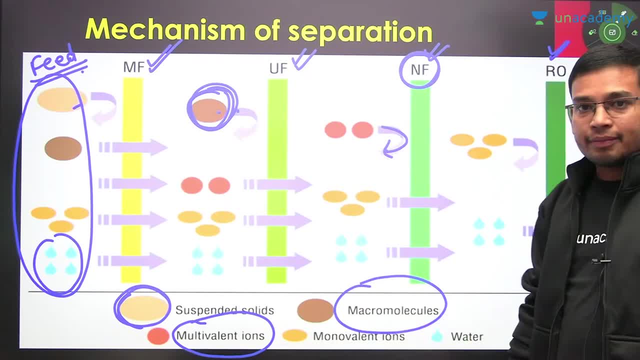 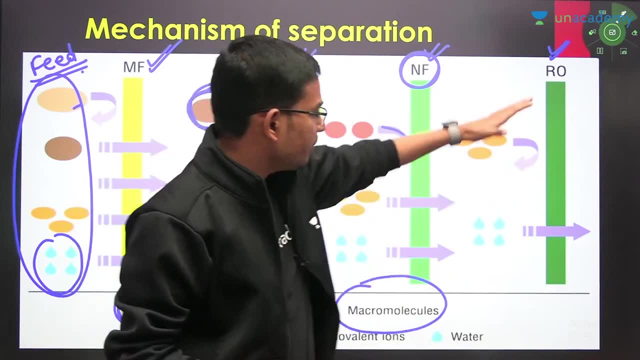 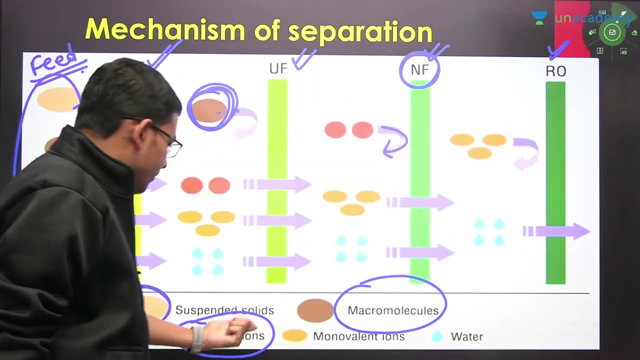 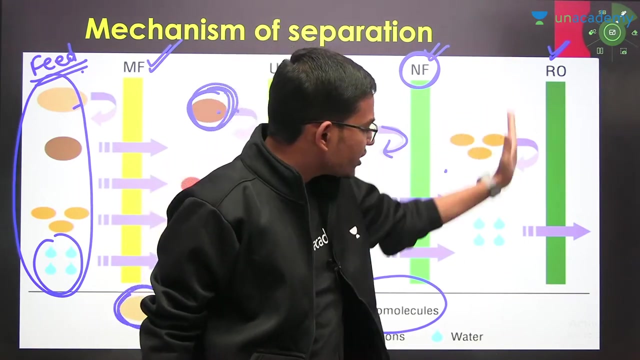 Scafree obliged to smartphone mil長 hands and water. Now in the picture we have reverse osmosis. What will it do? It will only allow water to pass. It has also stopped the monovalent ions. It has also stopped it, So it will only 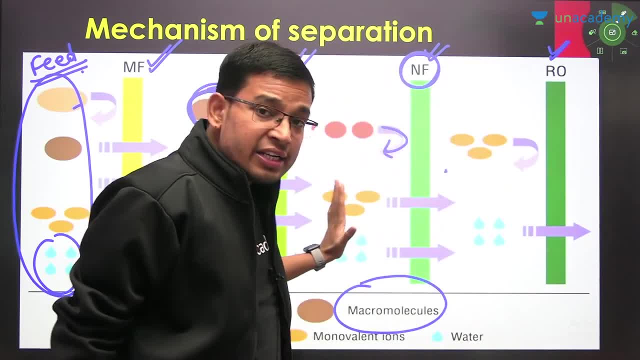 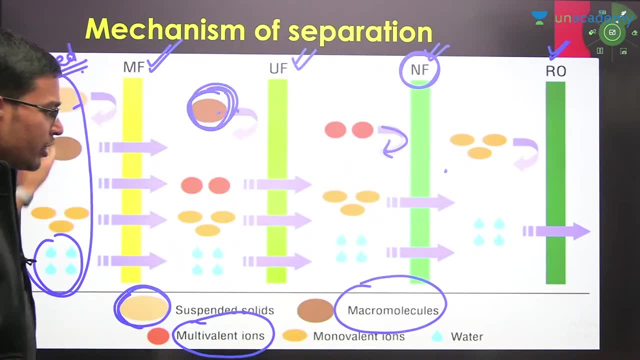 allow the molecules of water to pass. It will allow the molecules of water to pass. All the people have understood the mechanism. Yes or no, All the people will say that the mechanism is complete. What are the things that are being passed? What are the things that 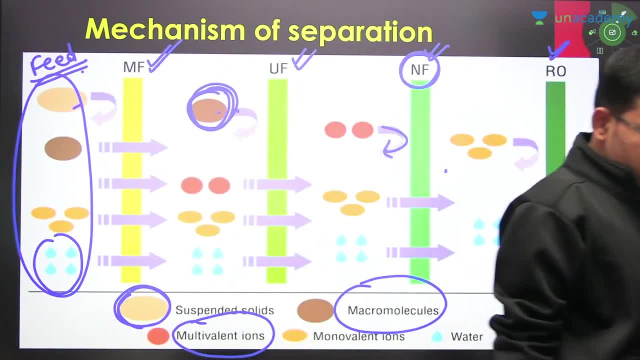 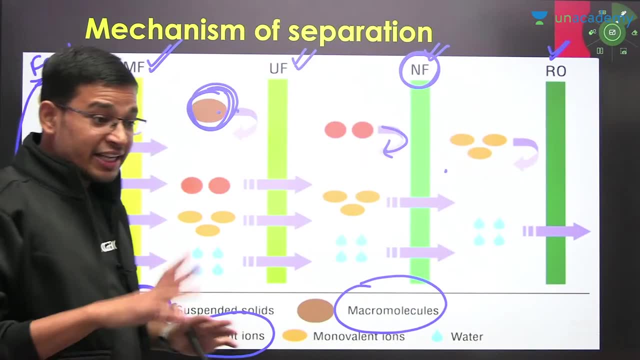 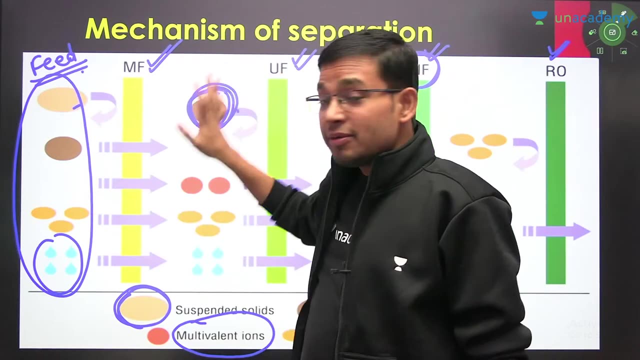 have been stopped. You should know this. See one thing in it Now: there is a lot of theory to be written in it. It is of one page. If I write microfiltration, The theory of one page is complete. If I talk about nanofiltration, 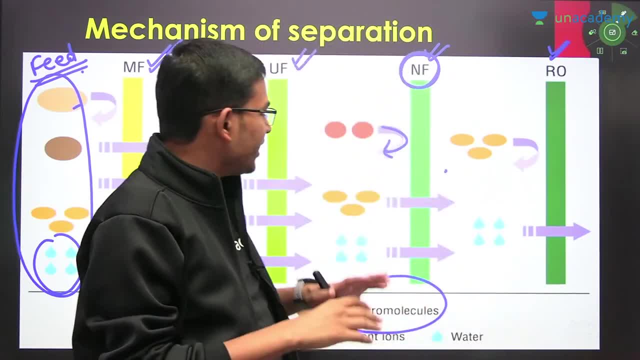 If I talk about nanofiltration. If I talk about nanofiltration, Then I will get to know the whole day. But what does it mean? The meaning of nanofiltration is that it is structuring the particles. This is your objective question. It is stopping which particles. 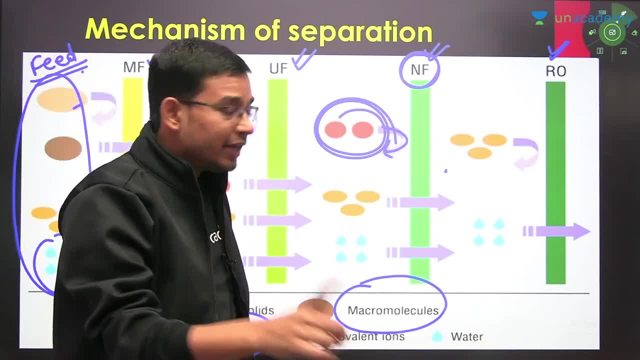 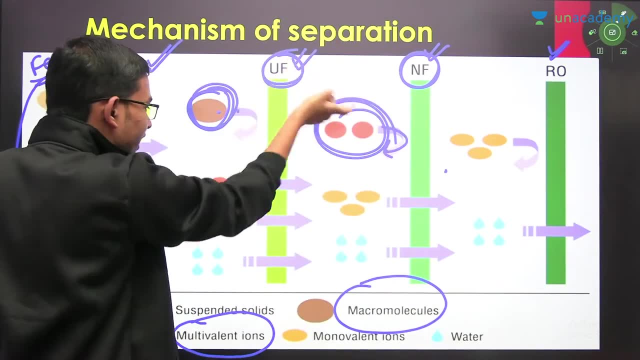 Simply your multi-valent ions. It stops them. This is its purpose. You just know this much that your work will be done. Okay, I will talk. What is the use of ultrafiltration, sir? What will it do in this? It will stop the macromolecules. This is the purpose of ultrafiltration. 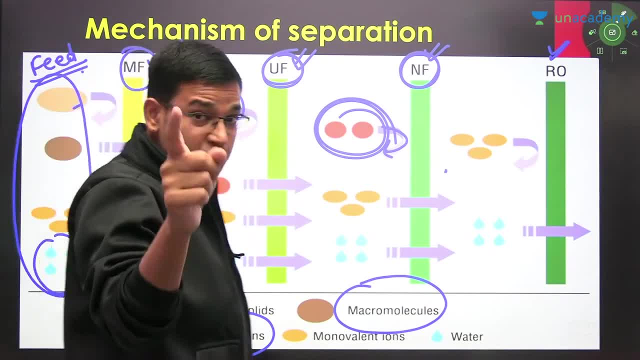 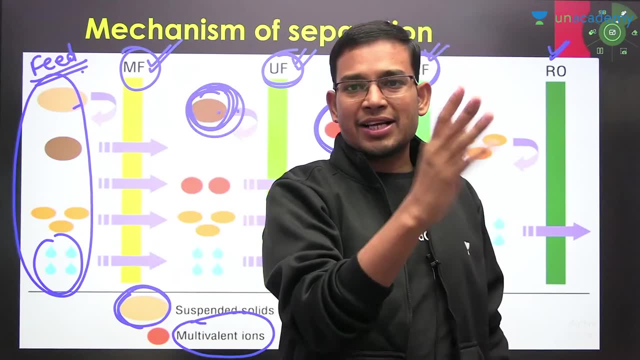 Sir, what is the purpose of the micro filtration? What is the purpose of suspended solid, solid solids? It will stop them, Multi-valent, mono-valent- and your macromolecules and water. What will it do to all of them? It will let them pass. This question can be asked in the. 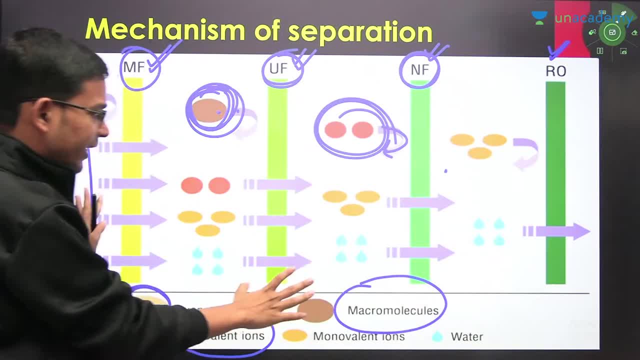 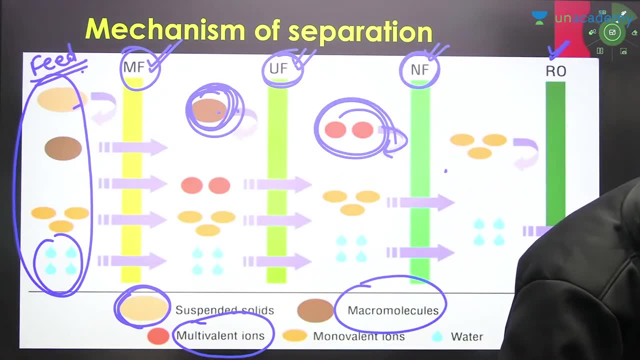 gate. One thing: all of you will make a good, beautiful figure In the same way. In the same way, all of you will make a figure and write: I am giving you two minutes of time. I am giving you two minutes of time, All of you will make a figure in the same way and 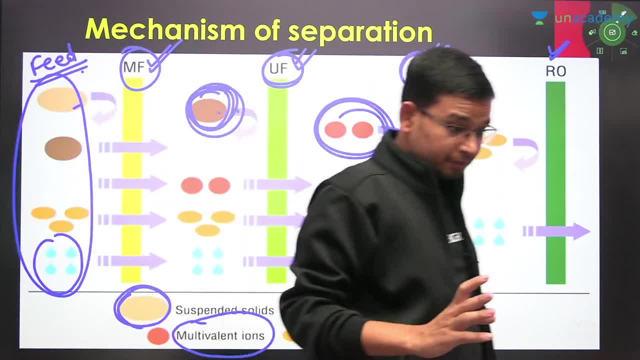 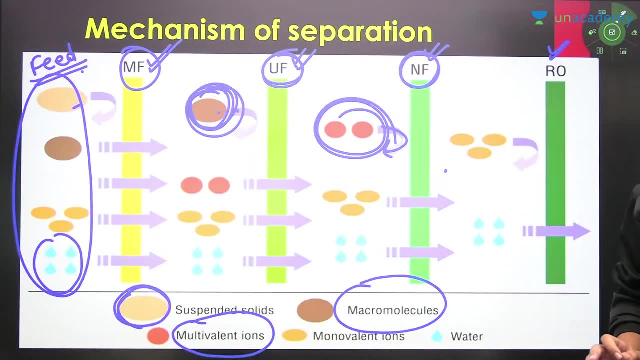 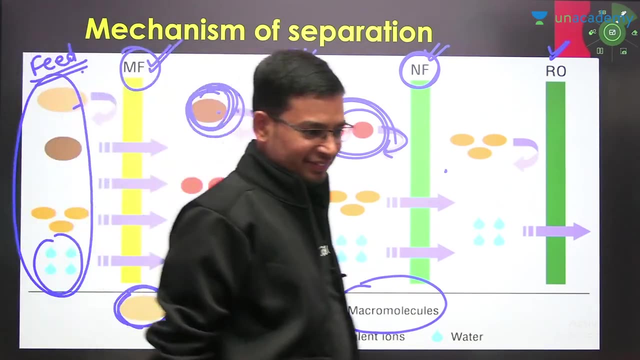 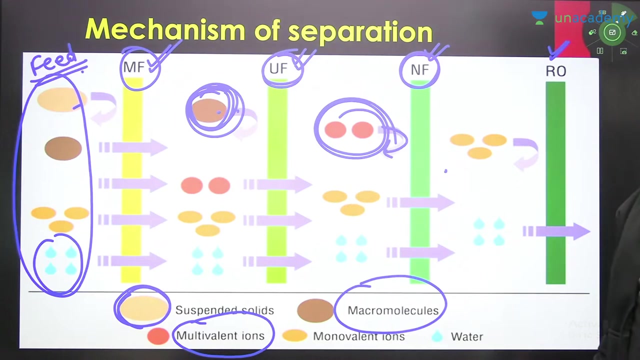 all of you will write in the same way, In the same way. What is the use of water molecules? Look, it does not stop the size, It is stopping the ions. It is fun. Very good. The molecules of water will be of minimum size, Okay. The 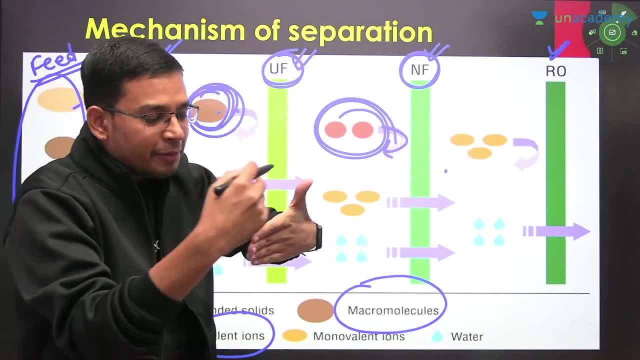 molecules will be of low size. The one with a large size than it your layer is coming Like. this is your filter media. So there is a layer here, So the particles which are suspended in it they will stop first, Then the ions will stop first, Then they will stop. 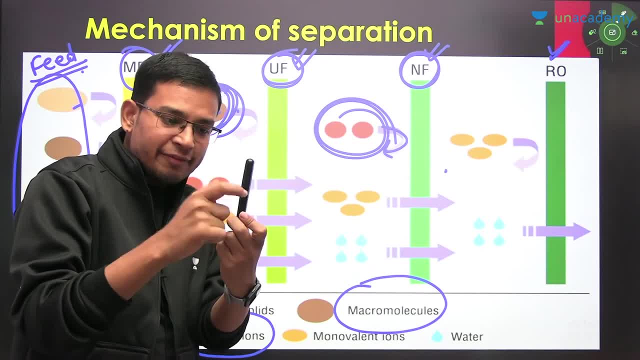 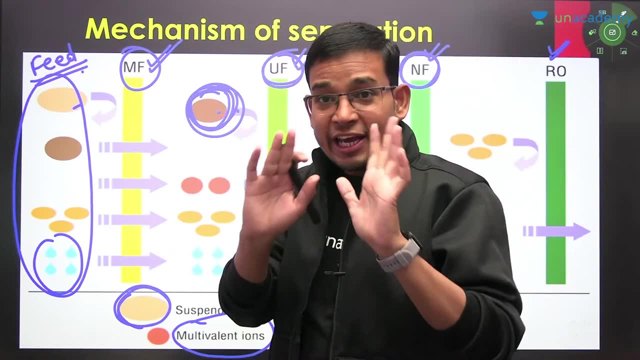 Then your molecules will be suspended for the second time. It will be suspended for one. Then your multivalent ions will stop. Then your water will pass there. There is everything in the feed. There is everything in the feed, Everything inside the feed. 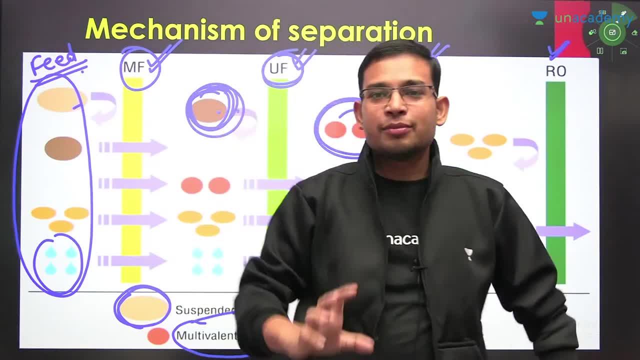 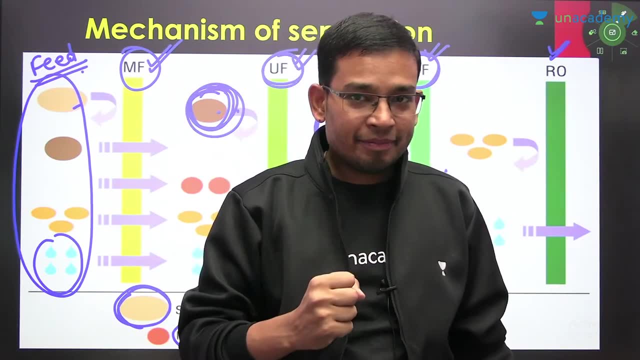 There is multivalent in the feed and there is also suspended in the feed. You understand this. There is the water of the river. That is the feed. You have to make it pure water. Okay, We were in IIT. This work used to happen there. 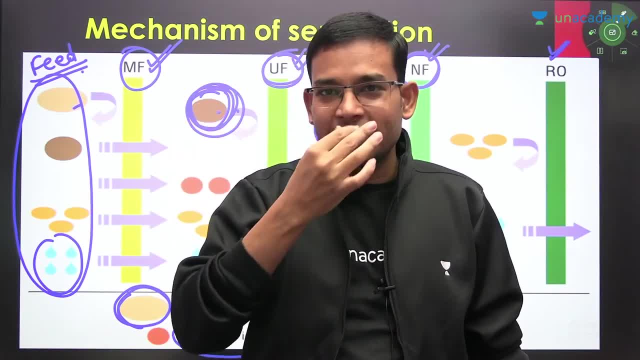 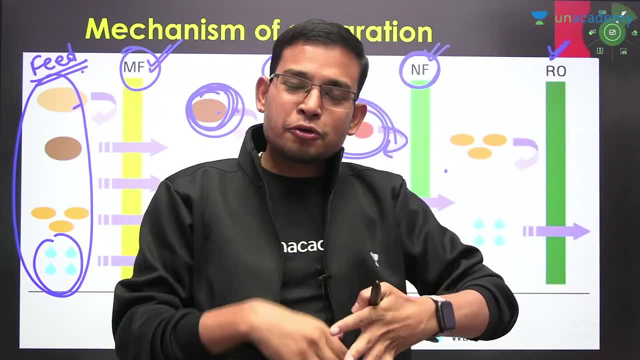 Although this was a little costlier. They had installed their own electricity In the form of electric medium. they used to bring Brahmaputra river. They used to supply it to the entire hostel to drink it. The entire hostel, professor, everyone used to drink the water. 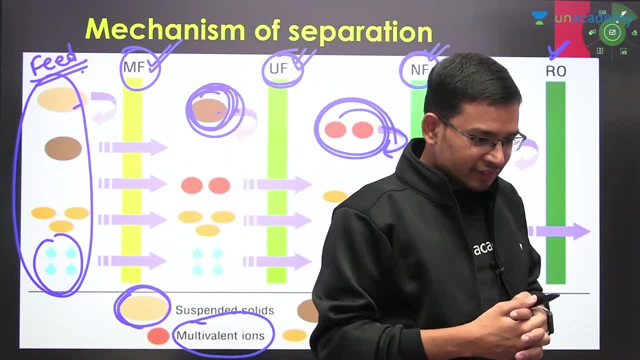 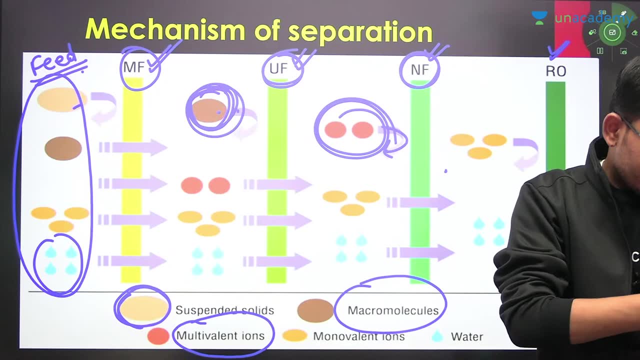 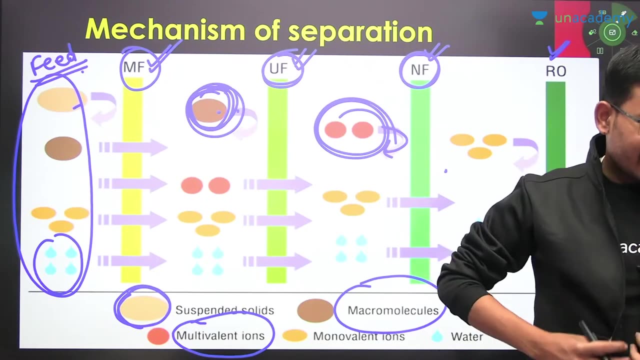 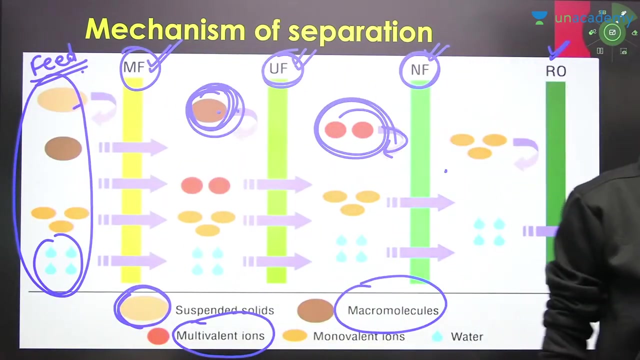 They used to filter it. so well, Very good, Let's go. So what does this mean? What is in the feed? After many days, the feeling of energy is coming. Yes, Okay, Lovely Right Now. see, Listen to me very carefully from here. 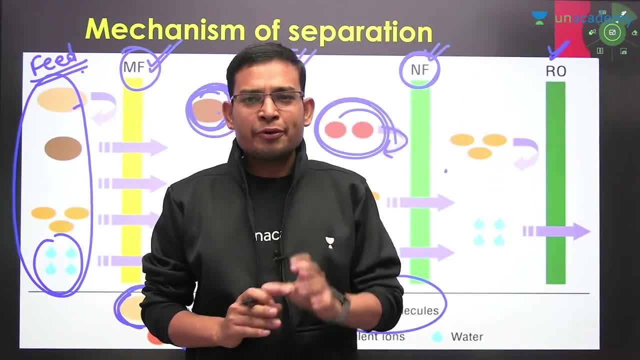 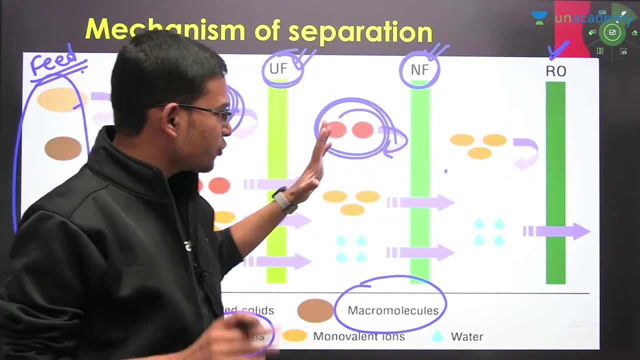 Now tell me this much: How will the gate ask questions from here? How will the gate ask questions? How will the gate think from this slide? You have to find out how the gate will think from this slide. Okay, Can any question come in the gate from this slide? 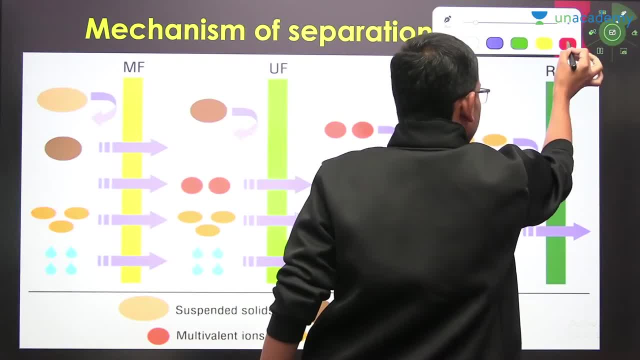 It can come. How will it think? Understand, sir, Look at how the question will come in the gate. Listen very carefully. The question that will come in the gate, The question that will come in the gate, Everyone tell me this. 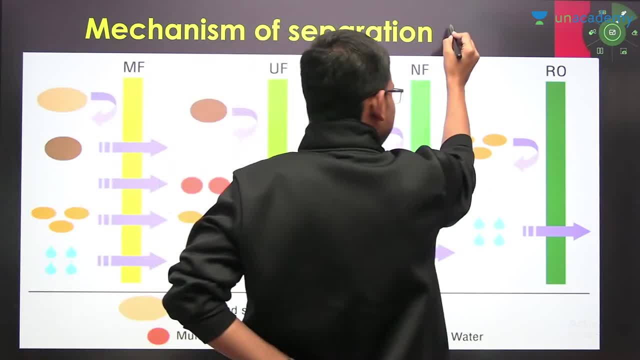 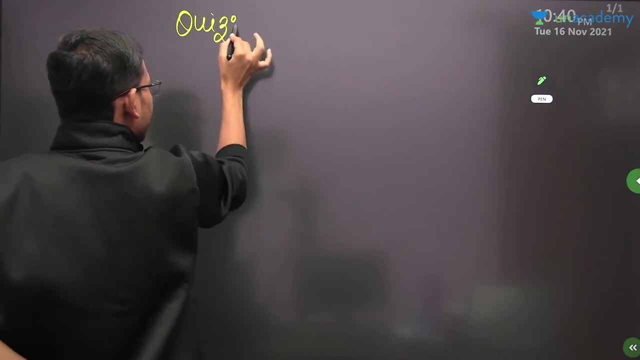 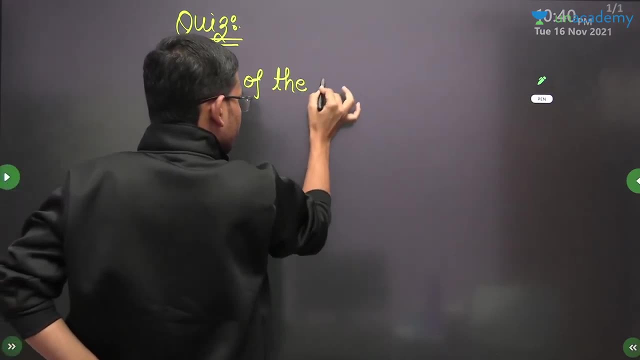 Order of the pores. Order of the pores. This is the gate question. Shall I tell you, Shall I tell you, Sir, take the question from this slide. Order of the pores. Order of the pores. What will be the order of the pores from all four filtrations? 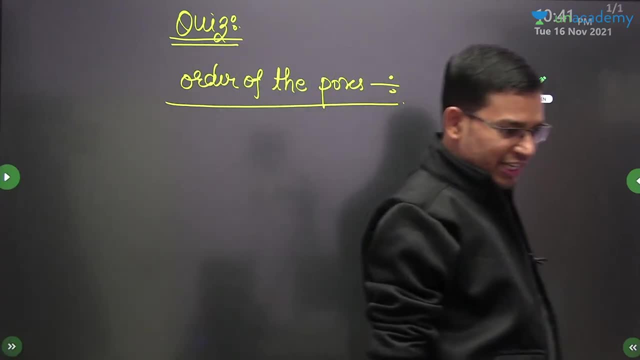 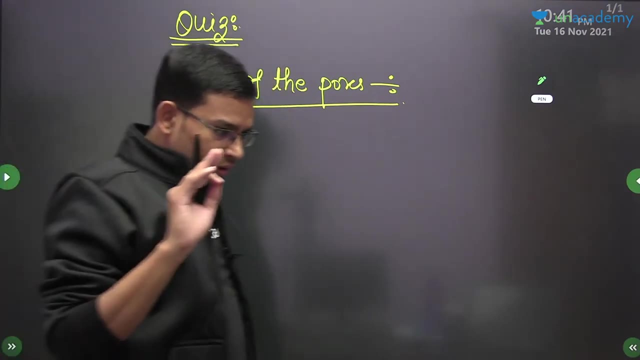 Everyone tell me What should be the order of the pore size. What will be the order of the pore size? This can be asked in the gate examination. Okay, What will be the order of the pore size? All four filtrations are sitting with you. 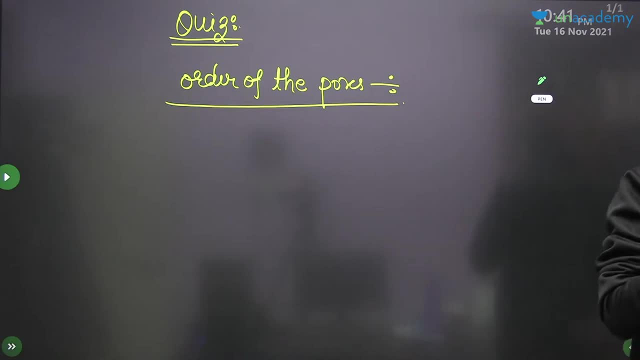 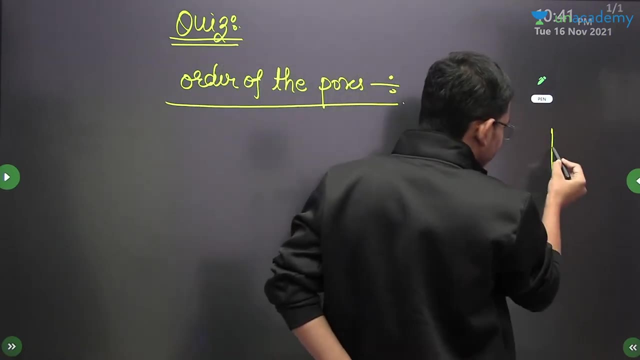 Everyone, tell me Everyone. Very good, What will be the most pore size? Suppose, what is your micro filtration? This is filter media. Now, what will be in this? There will be pores, Because it is semi-permeable. There will be pores. 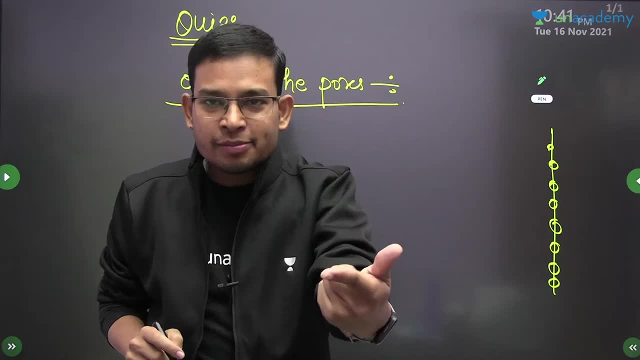 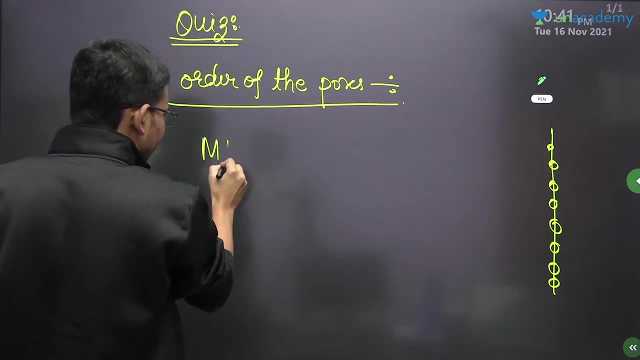 So now the size of the pore will be the most. What will be the most size? That can be asked in the gate exam. What will be the most size, sir? Macro filtration. The size of the most pore will be macro filtration. 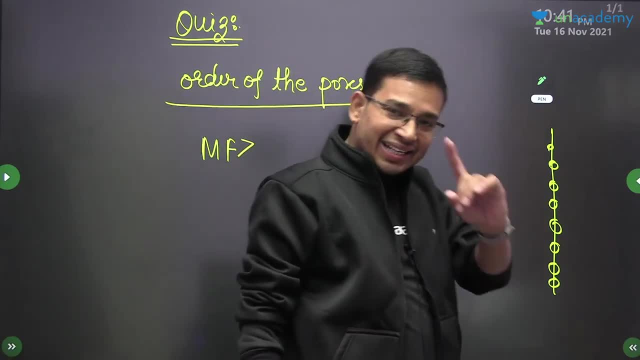 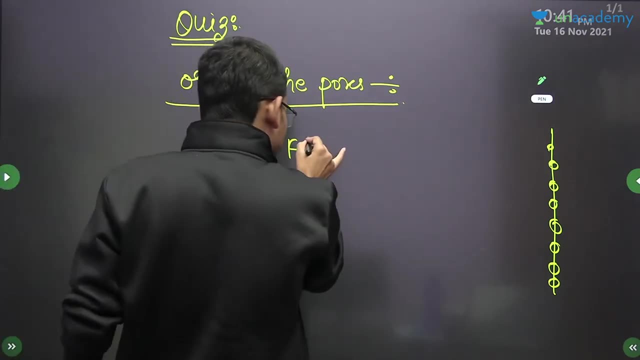 After that? After that, Ultra filtration? Yes, absolutely correct. After that, what will be the size of the pore, sir? Ultra filtration After that, who will have nano filtration? After that, the least pore size will be in the RO. 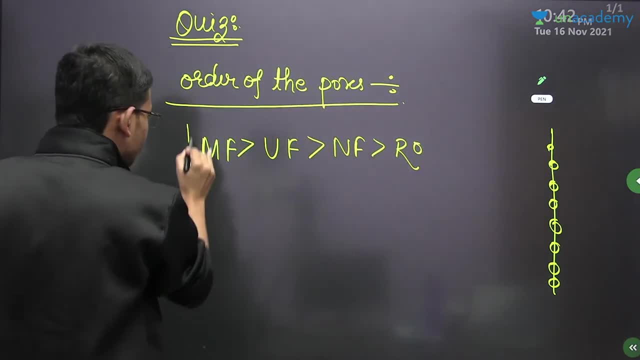 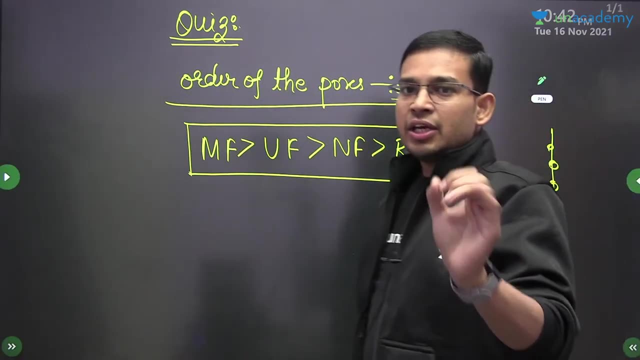 RO. It will be in the RO. This can easily be asked. this question can be asked. this is a poor size order. this is a poor size order. never in a GATE exam this question will not be asked. that this is the range of molecule. 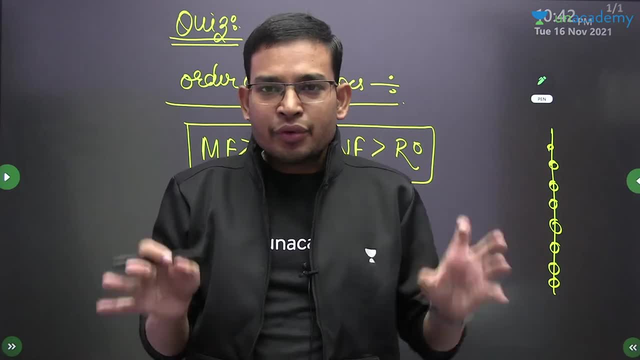 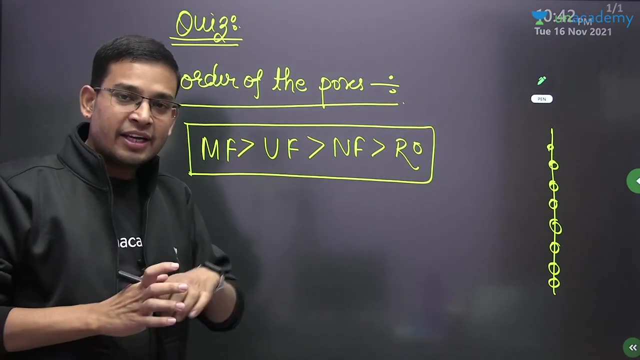 which one will fit in this? this question can never come in GATE because in different books the sum is different. so you know this GATE question can ask this, otherwise GATE itself will not get stuck in your talk. you know you have started studying 0.002 mm. 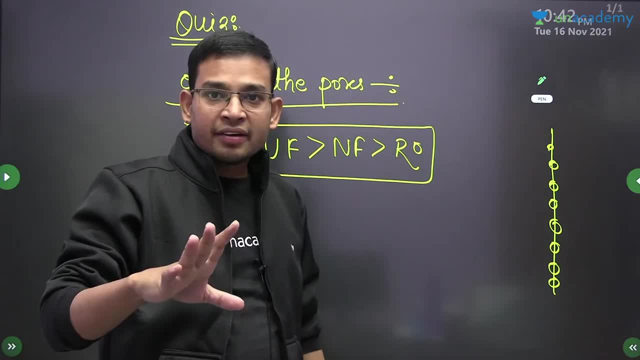 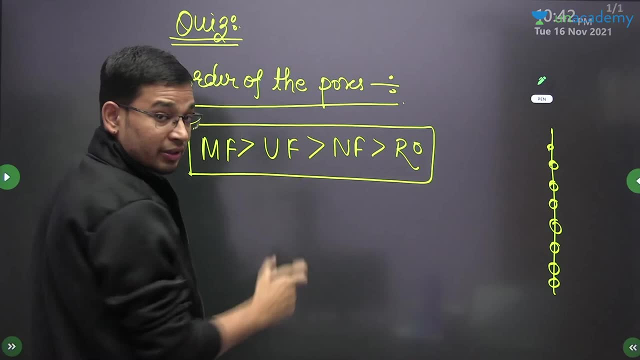 you don't have to remember all this. GATE can never ask you this. ok, you don't have to remember all this. GATE will only ask you an idea, and GATE will ask whether you have an idea or not. so you can ask this question. never start remembering the size. 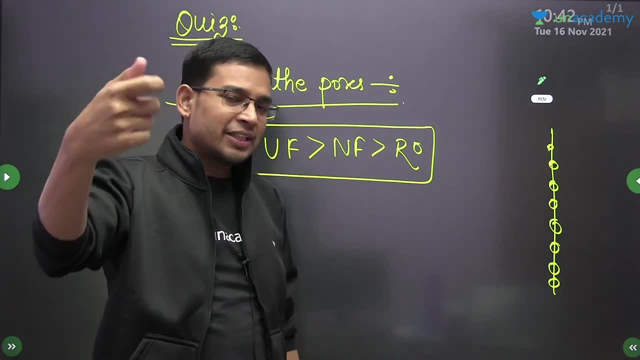 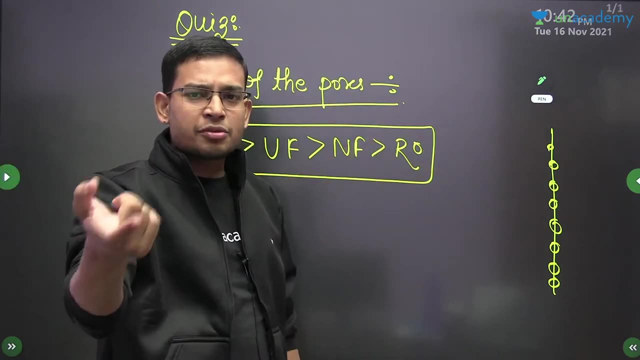 because the book will give you the size. I was looking at it today I said I will take the size and tell you this much size. so I gave a different size to Treval. I gave a different size to BK Dutta. I gave a different size to 2-3 research papers. so I said this question can never come in GATE because there are different, different, different. there are different in every standard book. so what will they give specifically? yes, that the smallest pore size will be in the RO. in which filter medium will the smallest pore size be? 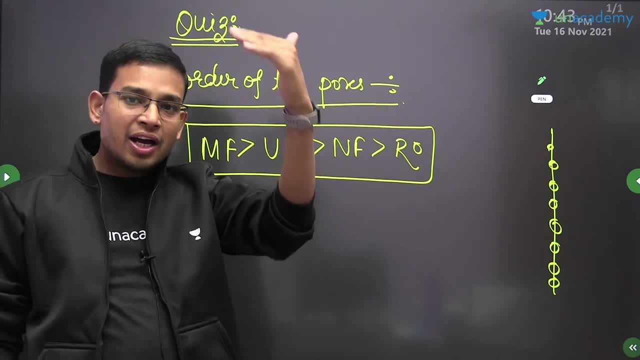 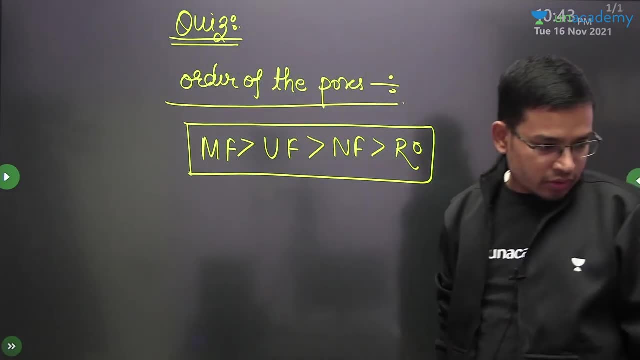 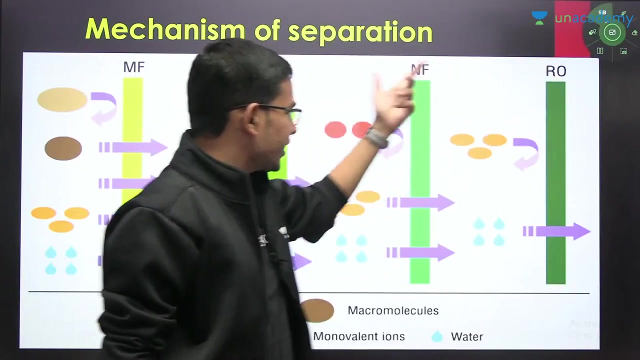 that is the RO system. the RO system will have the smallest pore size. this question can come in GATE. yes, yes, Vaishali, right, ok, pore size. can ask you. what else can GATE ask you? you guys think to yourself, sir, what change in this theory? 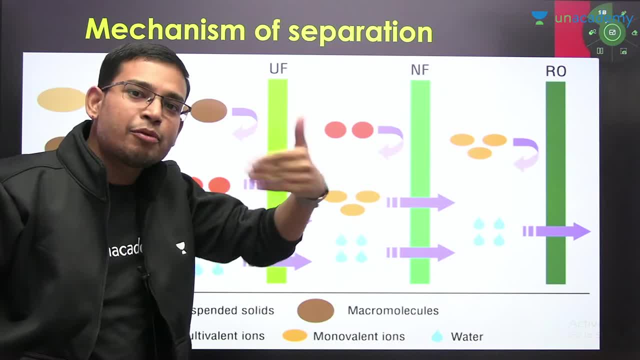 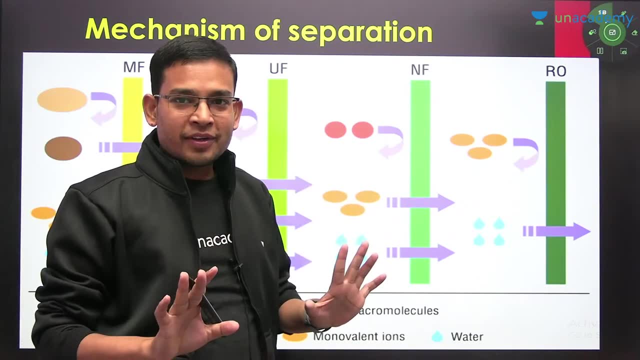 see, sir, theory is not from here. we will have to take the axe. what is the possibility? last year you attended my lecture. it was from his same lecture. you went to see the lecture where he said: reverse osmosis condition of equilendarum. it is also still there. 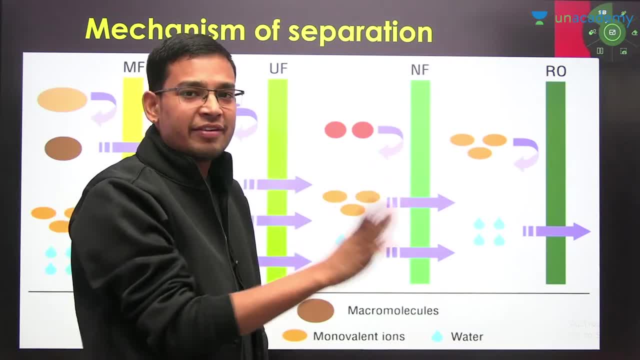 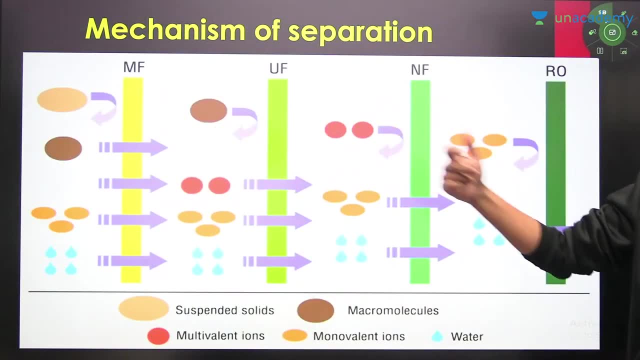 on an Academyff. he took the question straightly from the same. now we have to talk about a little advanced level. what else can it ask in GATE? what can tell everyone and how is the second question question from this slide? what can be the second question? 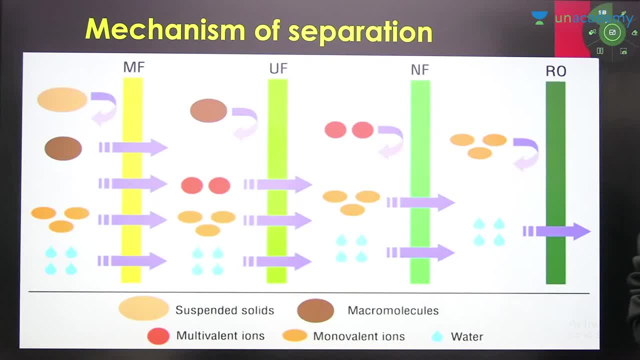 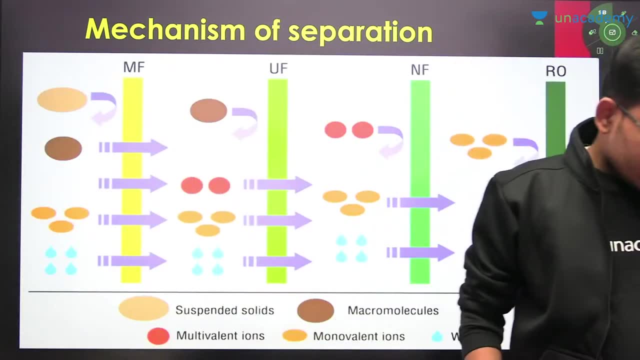 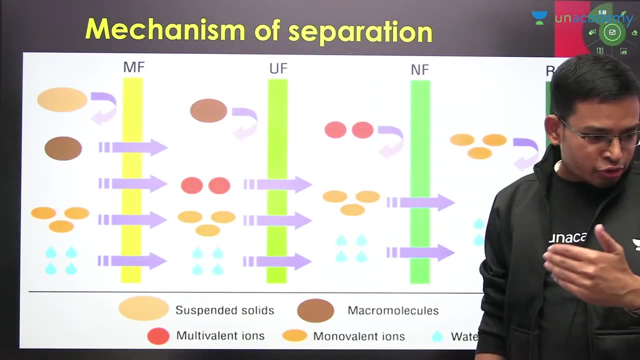 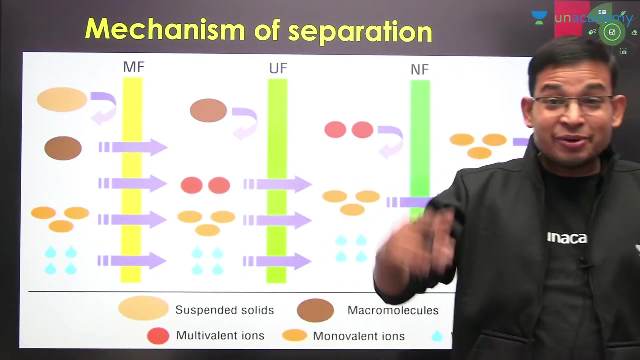 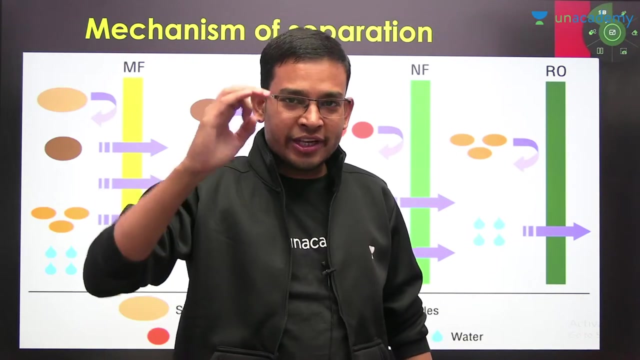 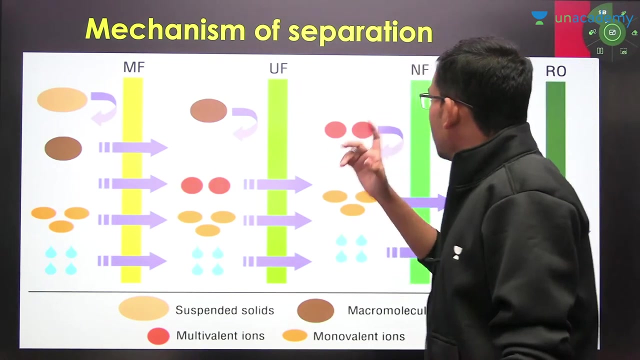 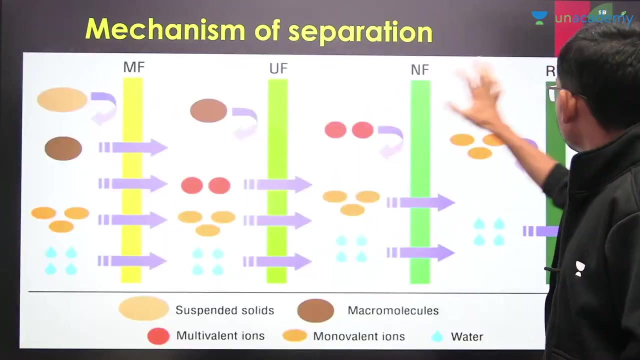 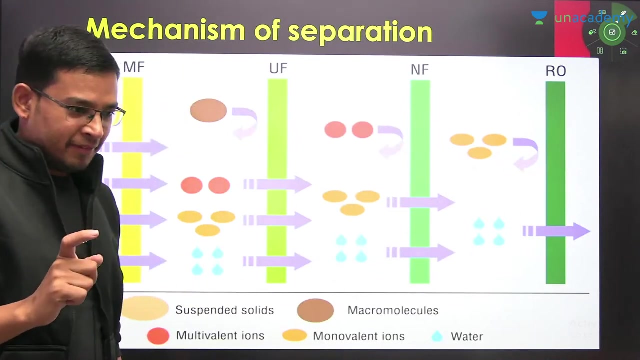 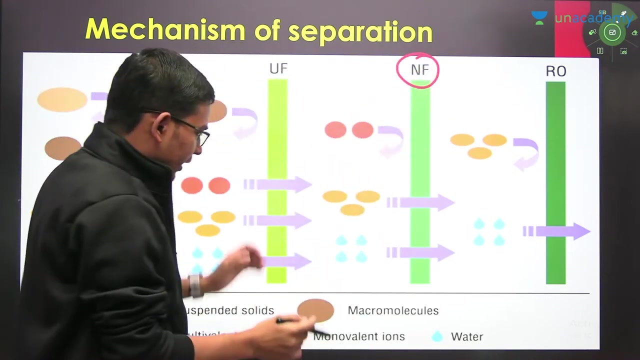 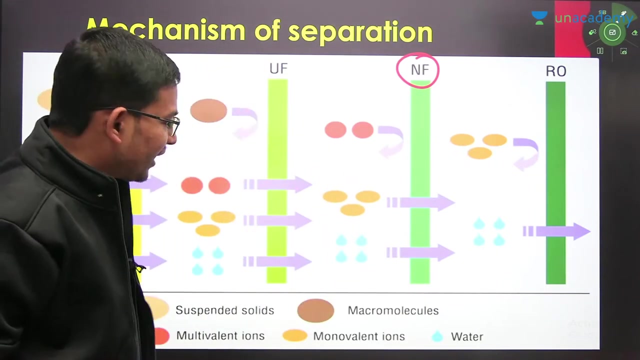 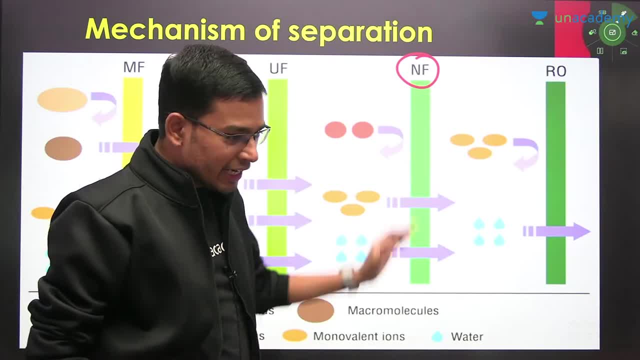 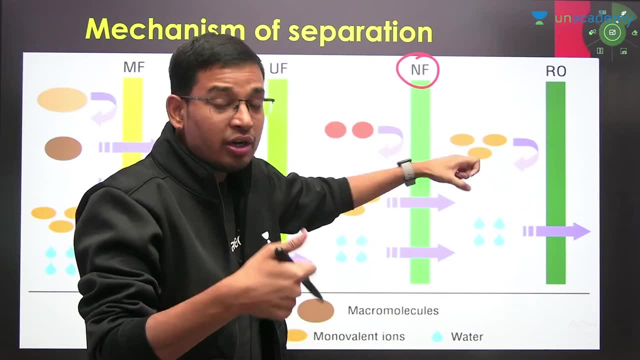 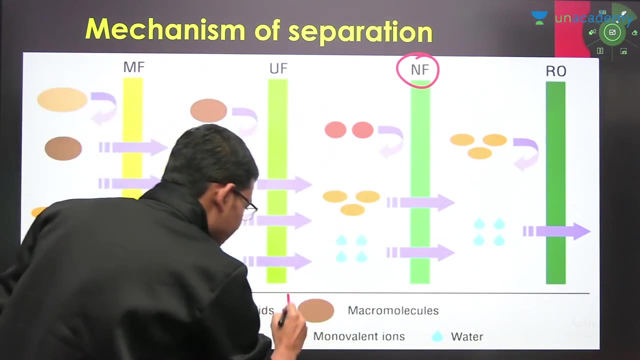 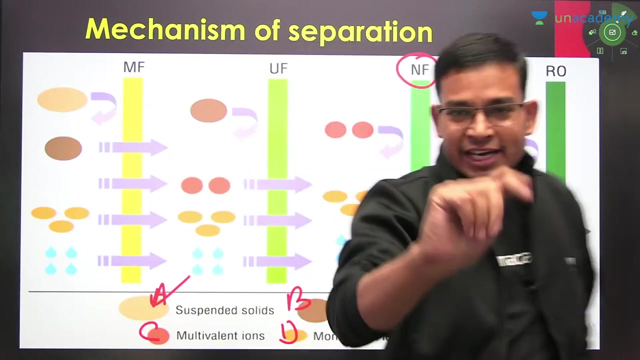 sir, sir, sir, sir, sir, sir. What will be the molecule passing through the nano? You have option A, option B, option C, option D, option E: Water will not be there. everyone knows that. These are the four options. You have these four options. 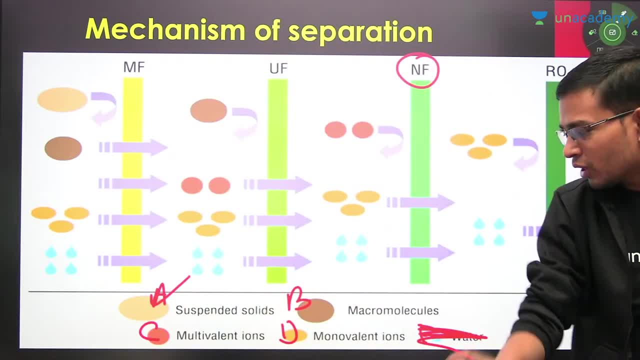 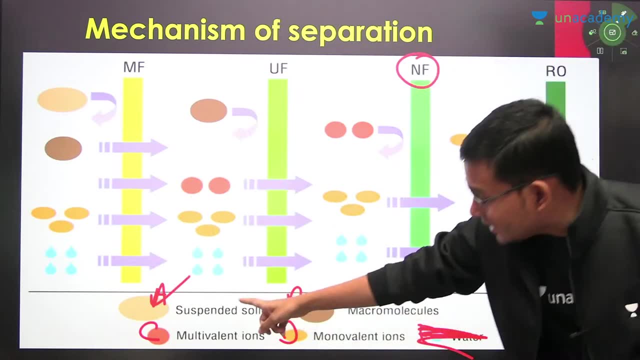 A, B, C, D. What molecule will pass through the nano Except water? Tell everyone What molecule will pass through the filtration through the nano. These four options can be there in the GATE exam. Keep in mind this question can be asked. 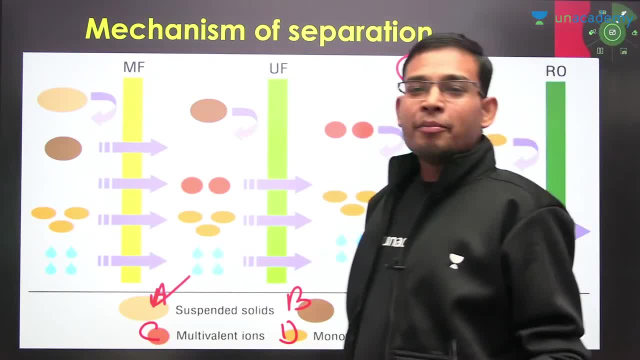 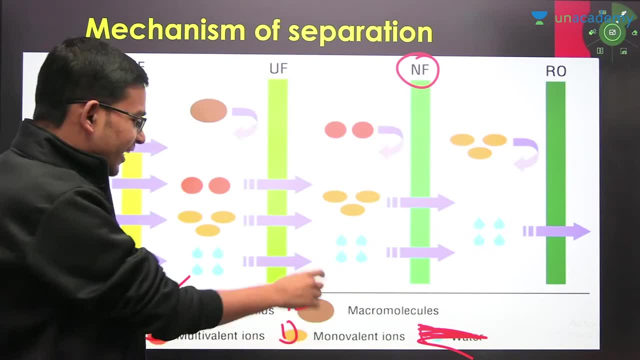 D part. Monovalent can be passed. Very good, Monovalent. Monovalent will pass. Which molecule will pass Monovalent? Okay, Neither will your suspended pass, nor will your multivalent pass, nor will your macro. 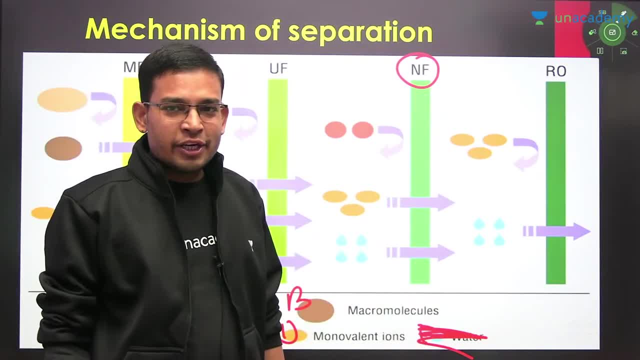 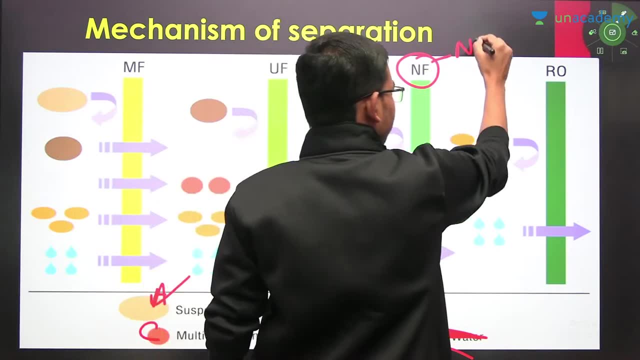 pass. Tell everyone: Can't this question come? Tell me: Did this question come out well with this theory? Tell me: Did you think of a nice question or not? Nice, Tell everyone this question. Did this question come out well or not? 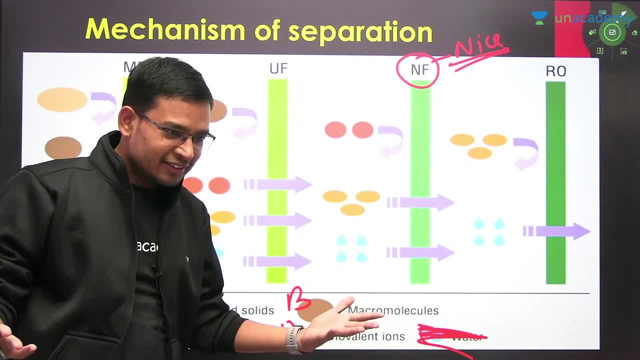 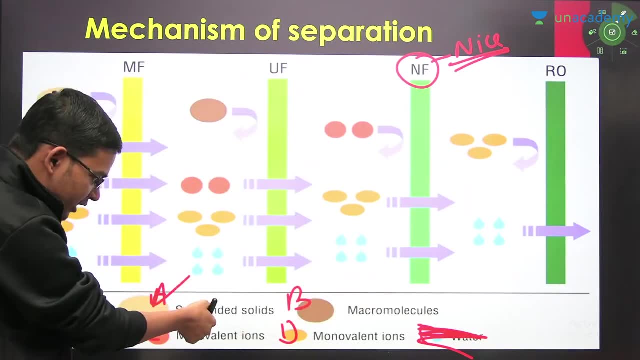 This can be possible. These four options can not be. This can be possible. This can be possible. This can be possible. That brother give me the nano filtration. What will be the passed element through the nano filtration? What will be the passed element through the nano filtration? 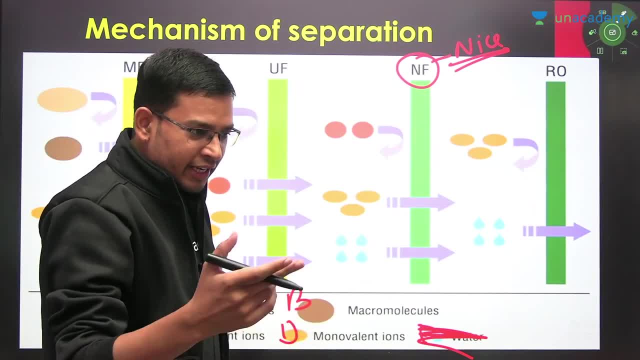 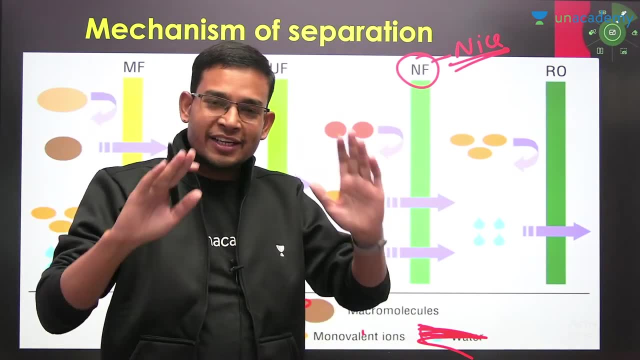 Suspended multivalent macro nano. Okay, This can be asked in the GATE exam. So on which will you tick? On the fourth one You can come. by ticking, You can read as many theories of nano filtration. 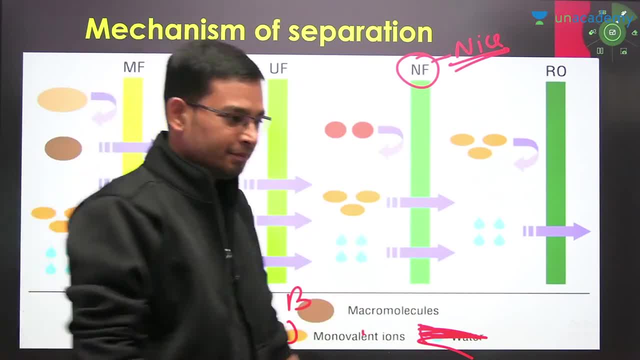 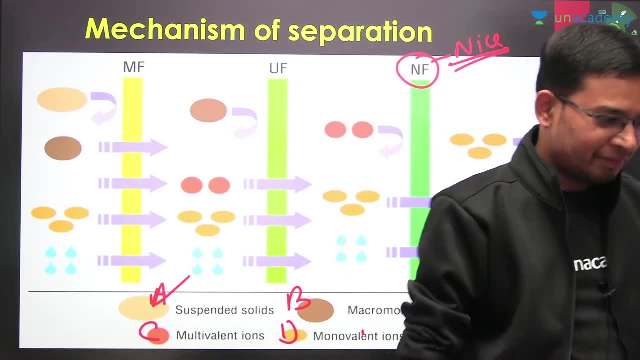 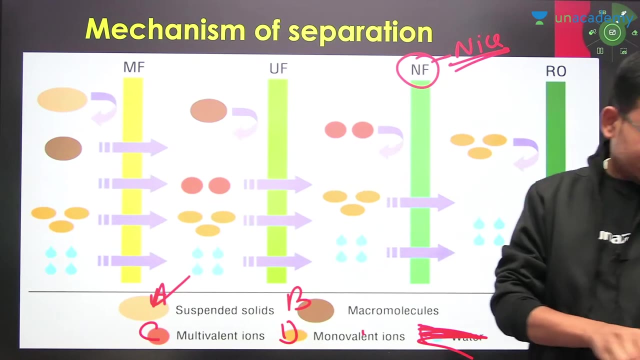 Brother, until you think like this, the question will not be able to be handled. Yes, In multi and monovalent. Yes, you will be confused with the word akshay in multivariate. ok, multivariate. yes, MSQ can also be made. 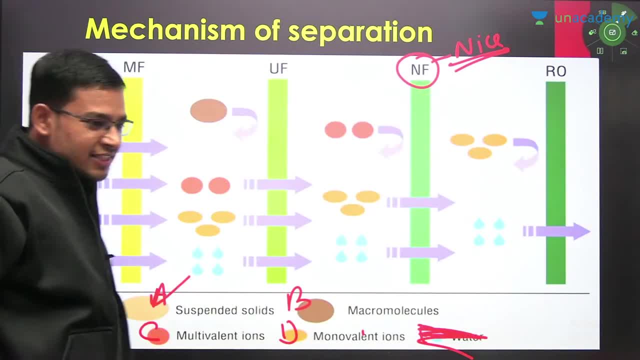 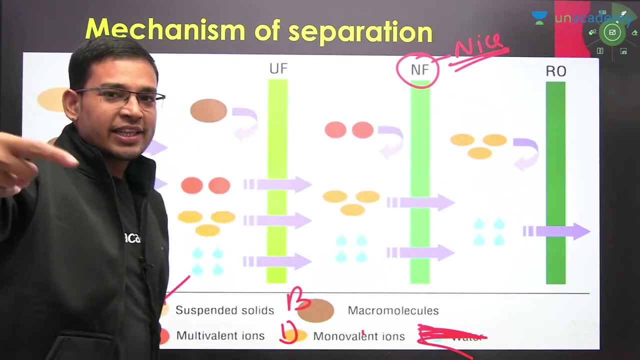 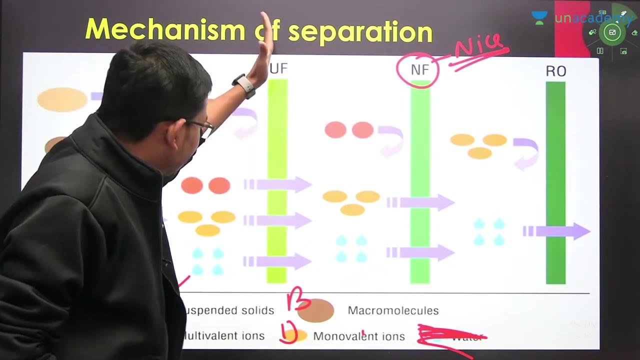 ok, lovely, this can be asked in the gate exam. amazing, MSQ can also be made. now. see, you guys started thinking- at least you are thinking that- how questions can be made from particular theory. right, come on. similarly, similarly, it can be said that which molecules will pass through ultrafiltration. 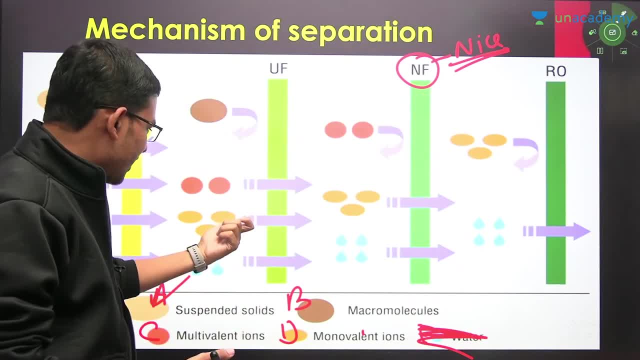 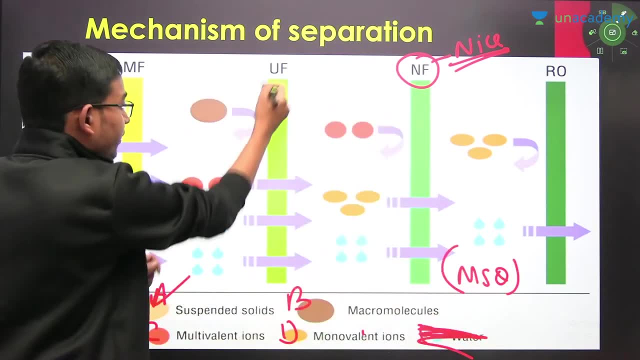 ok, MSQ can also be made from here, which will be passed to you through ultrafiltration, in case if I make MSQ from these four options, if I make MSQ, then tell everyone on which we will tick. for ultrafiltration in ultrafiltration. 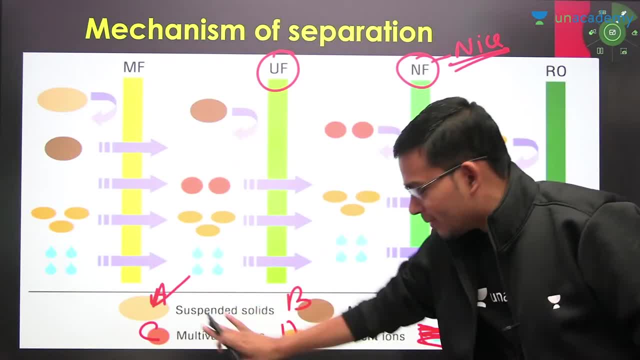 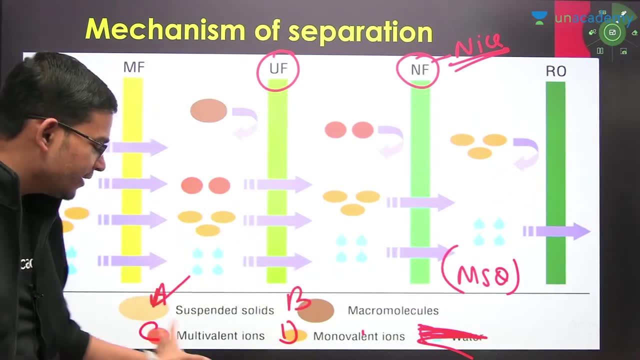 everyone will tell MSQ. you have these four options. everyone will know water, water. there are 70 children here. 70 children will tell water. which option will be there from? A, B, C, D, C and D? is the right answer? absolutely correct, C and D. 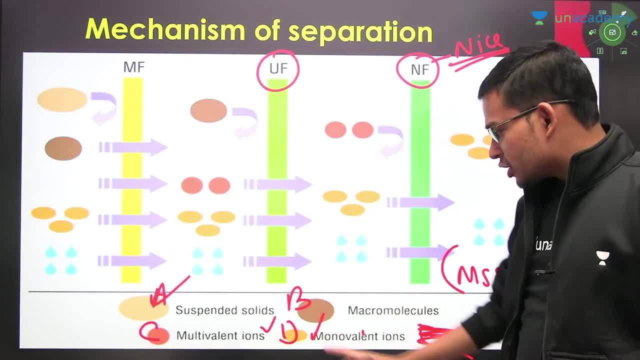 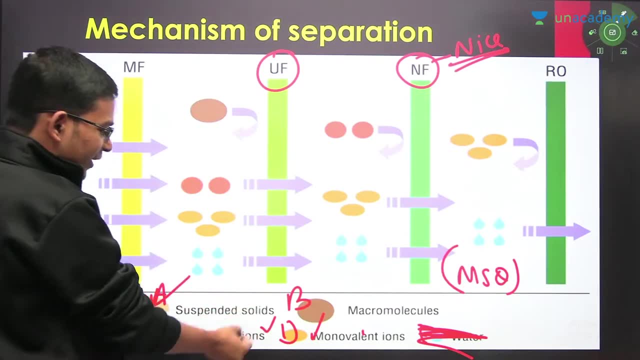 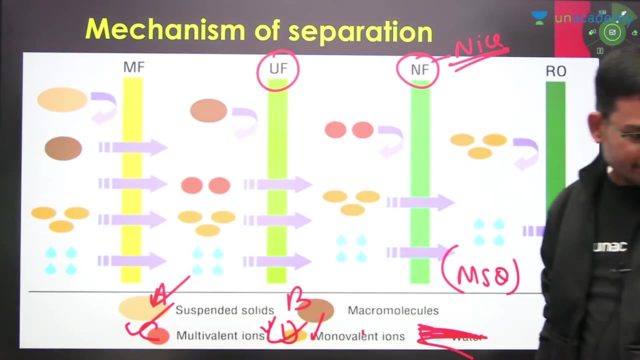 means multivariate, multivariate and monovariate will be passed, suspended will stop and macromolecules will stop. suspended will stop, macro will stop. by ultrafiltration means this will pass, this will pass. ok, C and D. C and D will be the right answer. C and D will be the right answer. 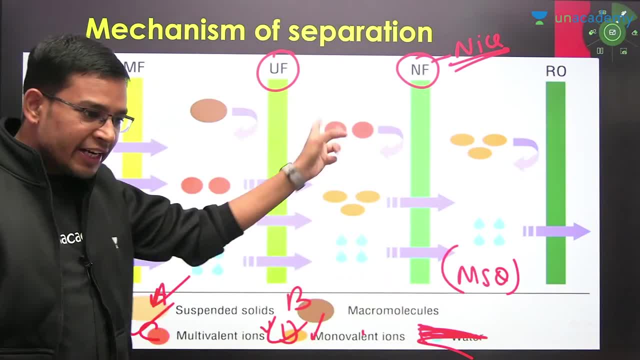 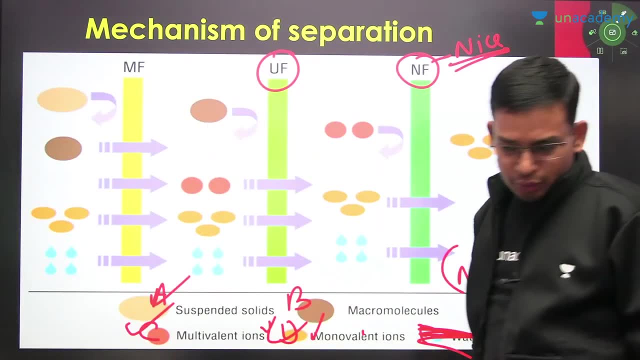 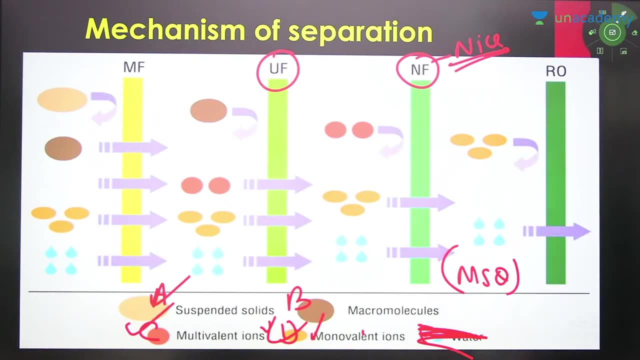 ok, I told you first you understood the mechanism. then how will you ask the gate question? he can ask in this way: from this slide, from this slide, C and D will pass, they will pass. absolutely correct, perfect, no problem. no problem, nobody is having any doubt. ok, come to the next point. 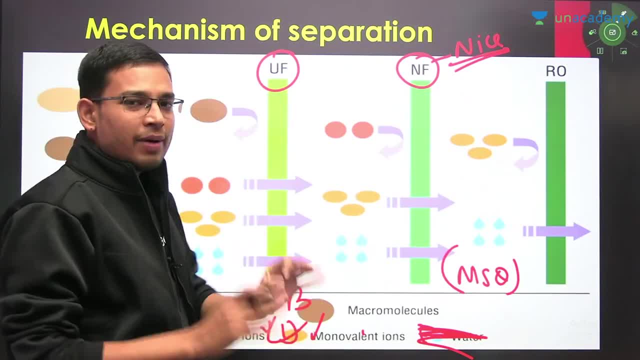 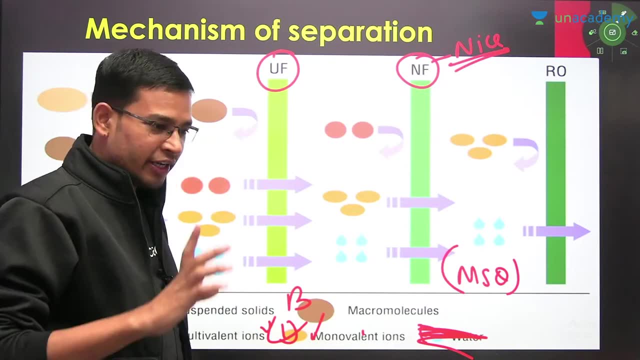 now from this slide: whatever question you get from the master, you can take a run easily, no problem. you can take one or two runs as you came, you can easily hit it. I know this much from this slide. if you will get any question then you will hit it. 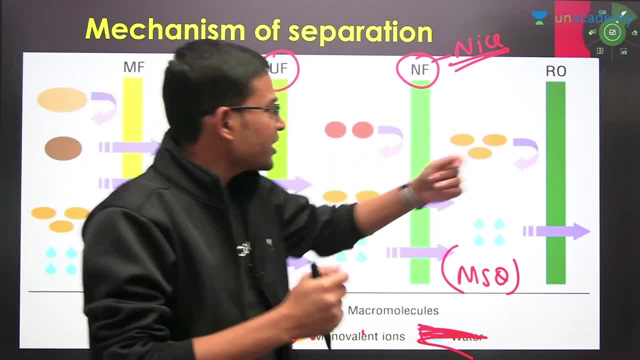 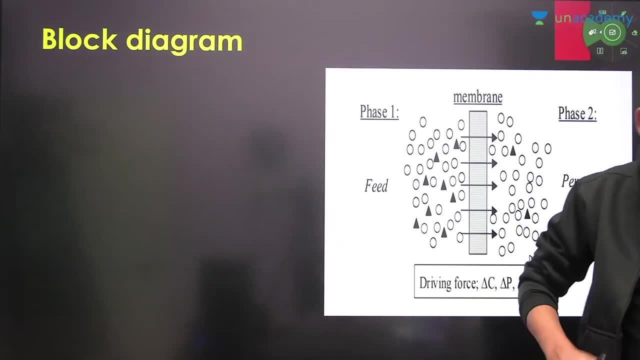 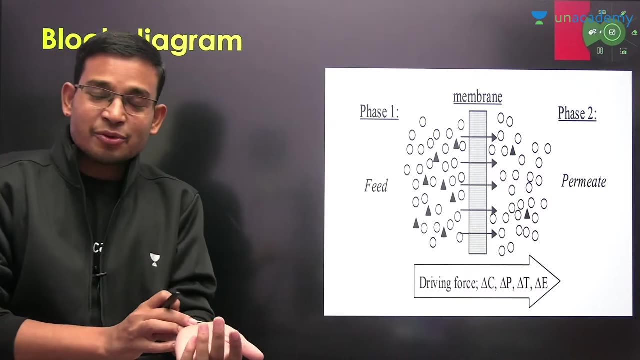 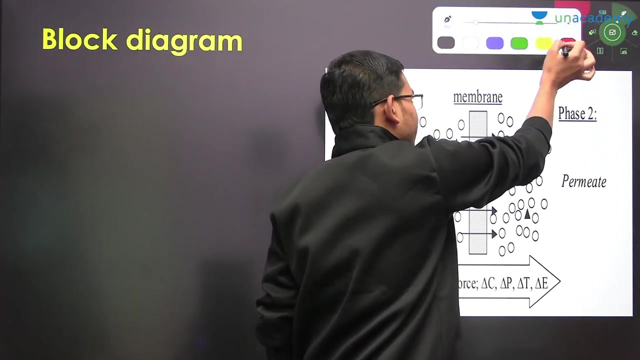 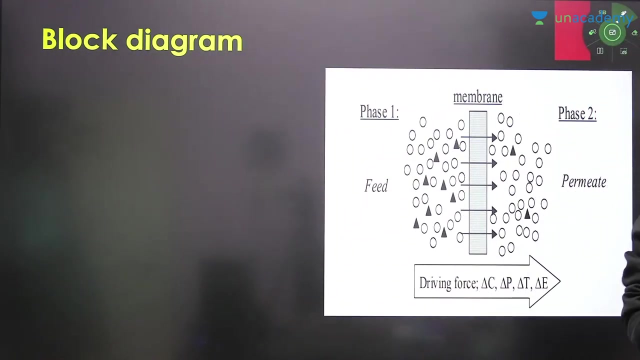 I am sure. ok, Okay, now come to the next point. Now I come to the block diagram. okay, the last 5 minutes topic and your number is here. one number is sure. yes, yes, I hope so that the question will come. I hope so, I hope so that it will come. but I know that if this question comes, then it will come numerical. if it comes, then numerical will come only. but yes, look, there is no COT in the GATE exam, that anything can come right, anything can come in the GATE exam. nothing can be said from the beginning. from the beginning, Guru can say something. 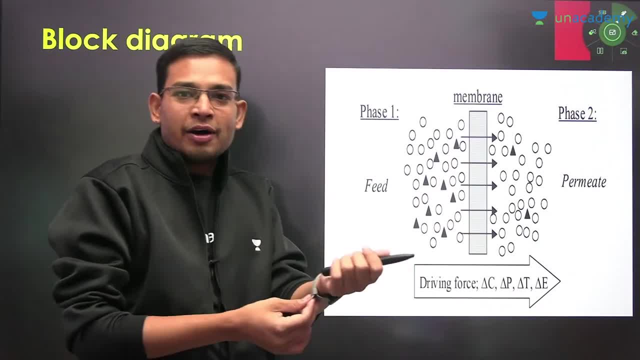 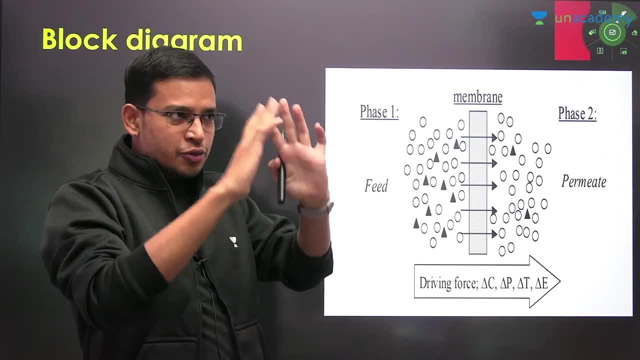 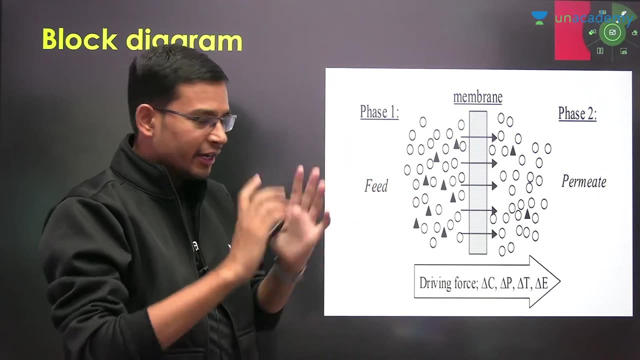 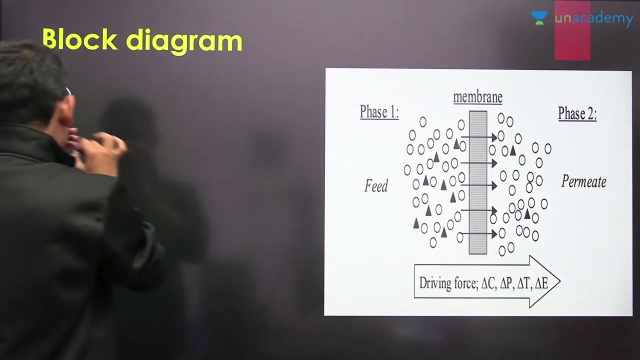 nothing can be said. okay, you just have to think there, you have to think, no matter how the question comes. you will just think, think and take out the question. okay, always keep your mind open, keep all the things collected, okay, whatever things you will get, just execute them. that's it. don't panic, stay cool. now come to the block diagram. block diagram for membrane separation. I will talk about this. what is the block diagram? okay, I will talk about the block diagram here. 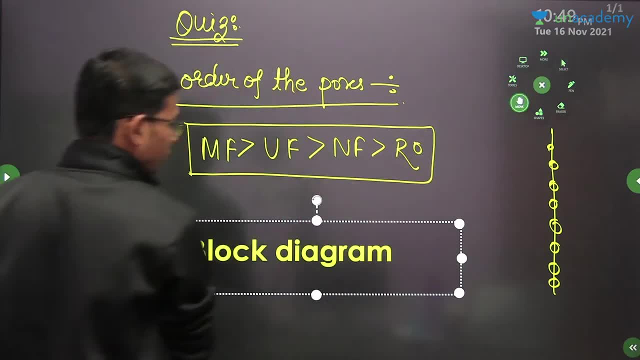 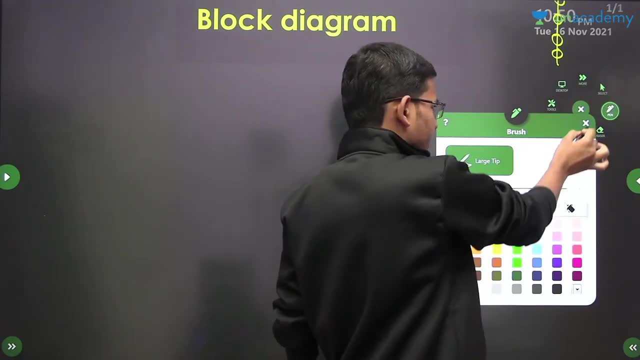 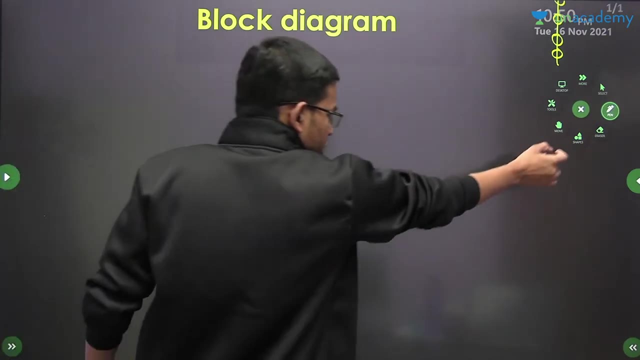 block diagram. okay, now I will talk about the block diagram here. look very carefully, very carefully. you are in your numerical part. you will start a little from here. okay, block diagram. let's suppose this is your block, this is your block. 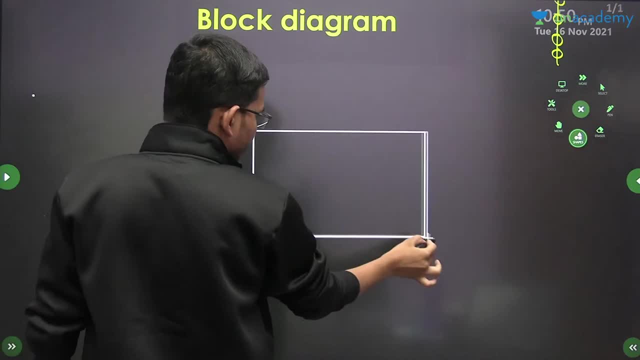 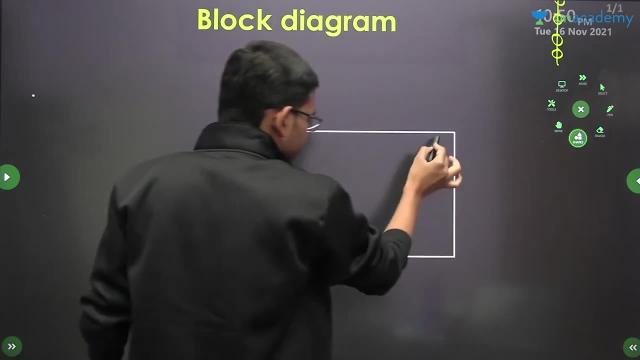 and this is your block. right, this is your block. look very carefully. this group is your block. Okay, creep here. repeat: comment here: кPadman block. and in this way your membrane is attached. in this way your membrane is attached, ok. 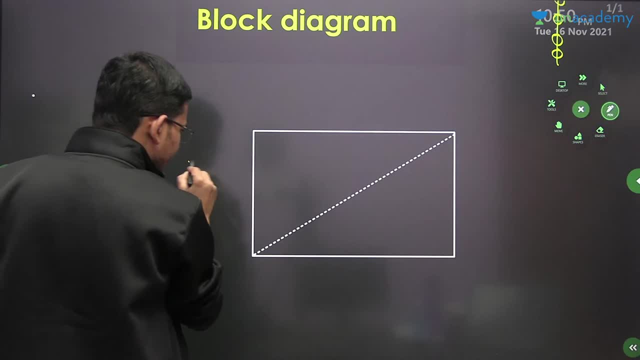 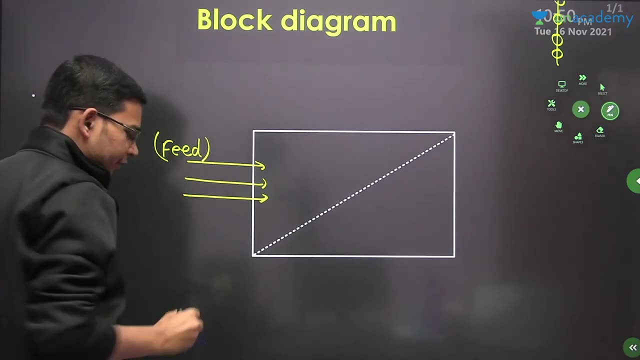 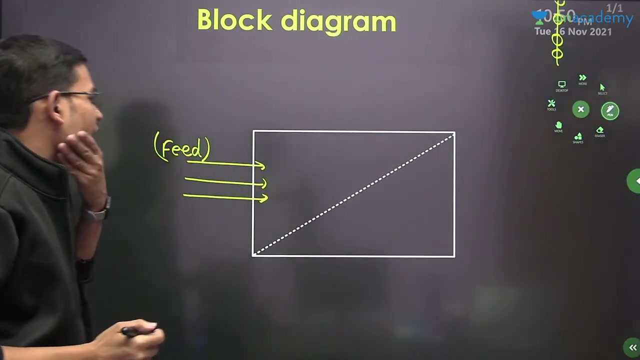 this membrane is attached. so what i will do- i am using some term from here. what i am doing? feed. i am getting the feed to enter. this is your feed. everything is there in your feed. keep in mind in feed your suspended macro, micro, ok ions, etc. everything is there, ok now. 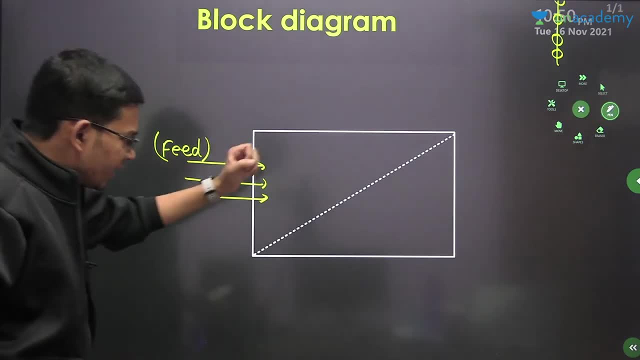 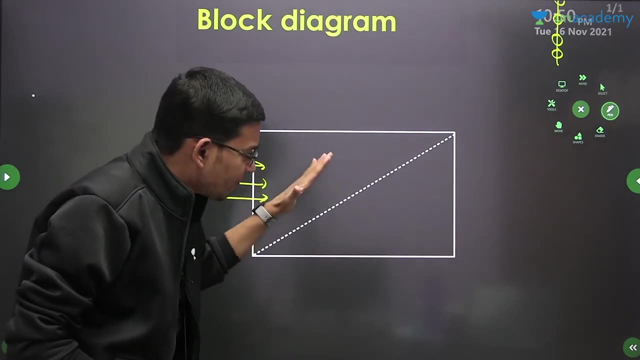 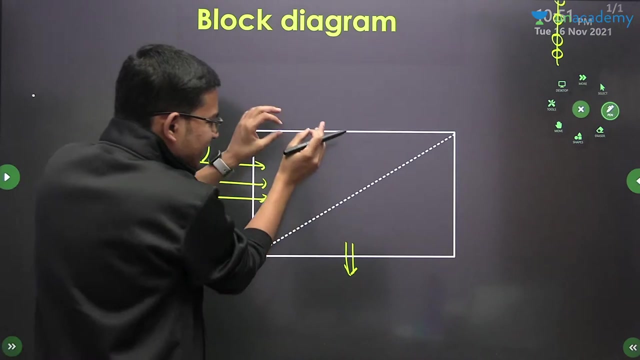 from here it is divided into two parts. this is called feed. as much as your membrane passes. as much as your feed passes means it is filtered. that is called, what is called by all of you. what is called, and what is called the one which is sustained on it, which stops what is called. 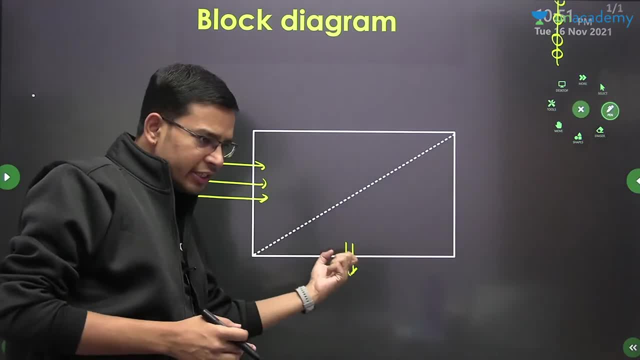 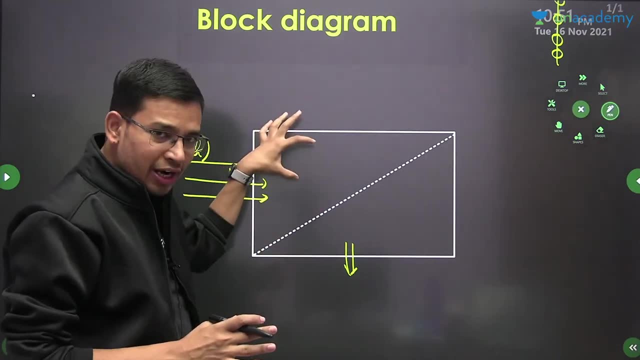 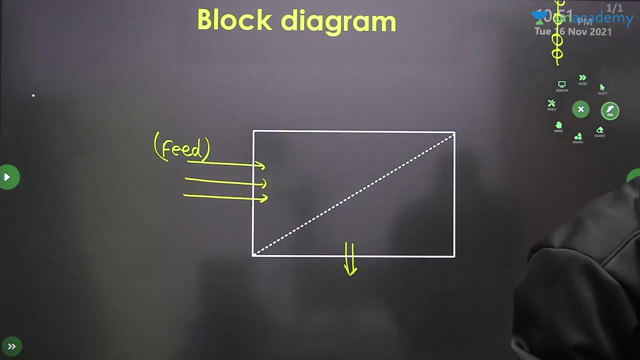 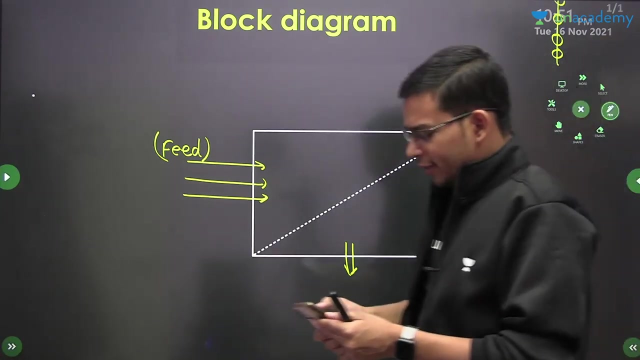 this is called, what all of you will tell. what is this term used? does anyone remember? here will come two terms. here one will come. what is called the one which is sustained and what is called the one which passes. what is called? all of you say yes, very good, very good, lovely, super. 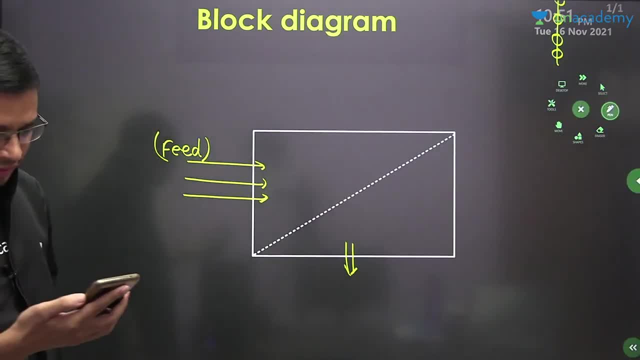 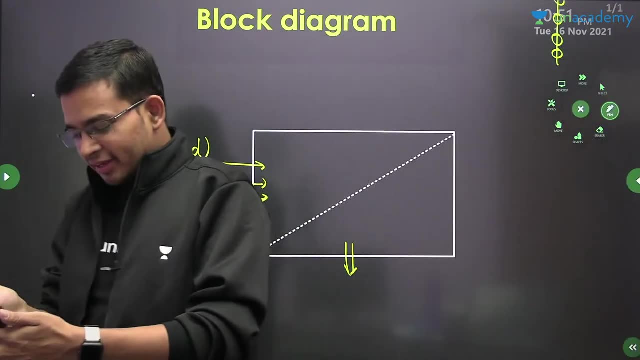 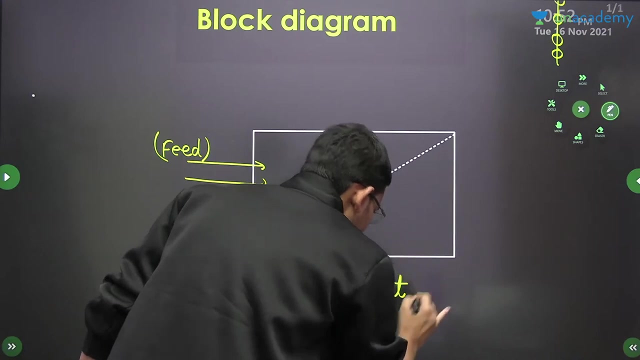 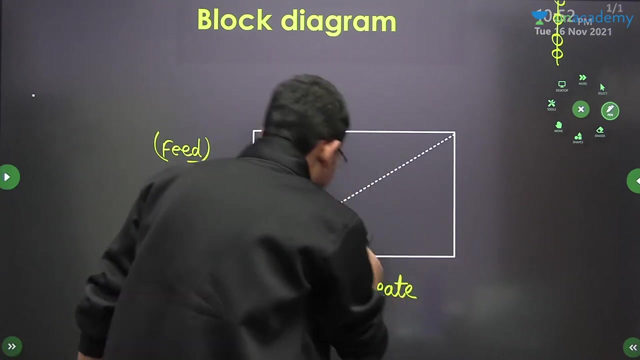 lovely, what is it? filtrate and retentate. filtrate and retentate, very good, permeate, super. we will use one term here: permeate, permeate. ok, one term we will use: yes, very good, permeate. ok, one term, you will use permeate. and here, which part will stop? that we will call an retentate. 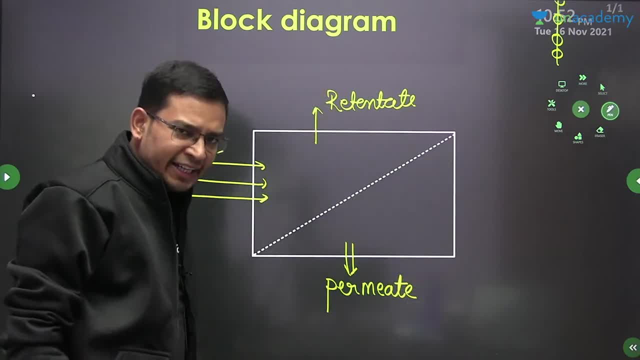 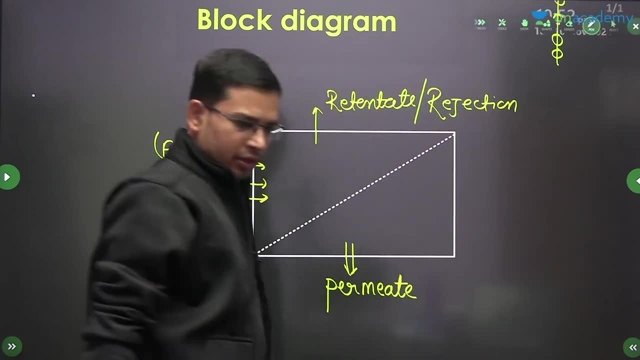 Remember this term completely Retentate. The second term we will use is rejection. Rejection, Right Rejection. The second term we will use is rejection. Will we use anything else? Yes, We will use permeate in this. 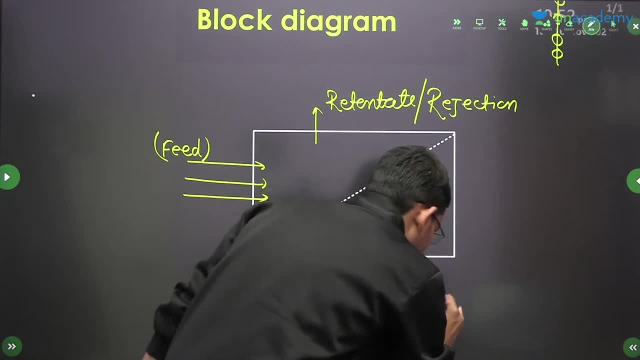 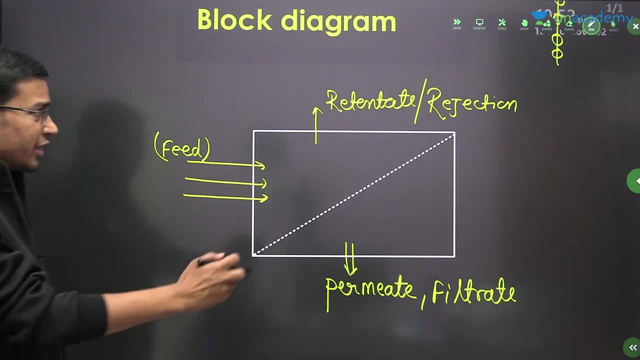 And we will use filtrate in this Filtrate, Filtrate, We will also use filtrate. What other terms will we use? All of you just tell me. What else will we use? Everyone, Everyone, All of you just tell me. 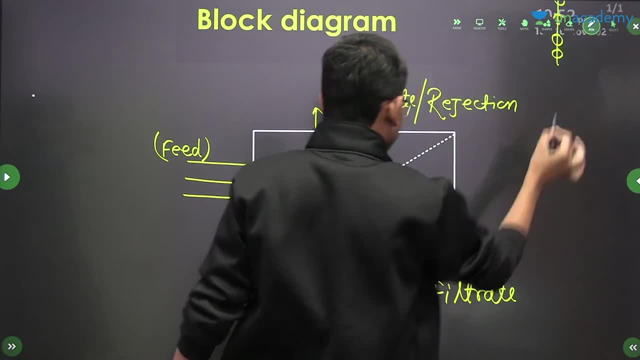 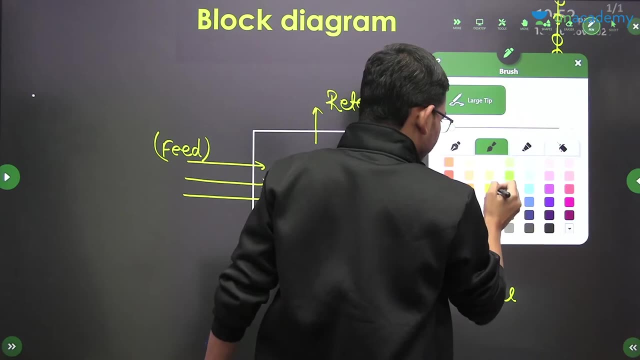 What else will we use Everyone? What other terms will we use Everyone? What is this part of yours? It has passed. What has happened to you, Guru? it has passed, Ok, And this part has stopped. This part has stopped. 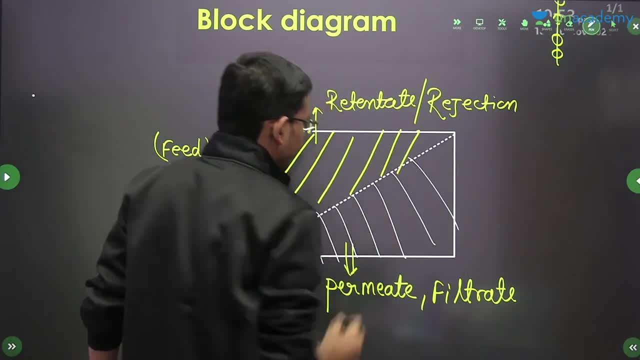 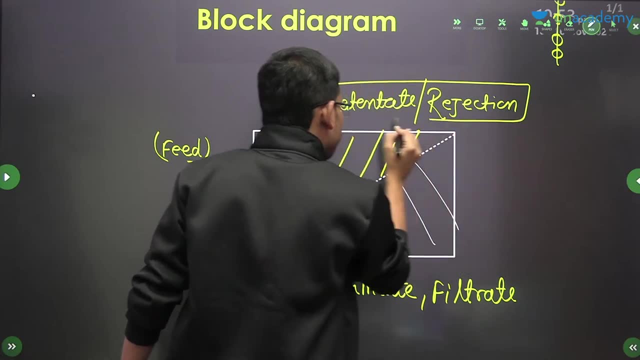 Ok, It has stopped. Right, We will say this. The part which will stop Feed's some amount of the part which will stop, We will say it: Retentate and rejection. Ok, We will say this, Which will pass. 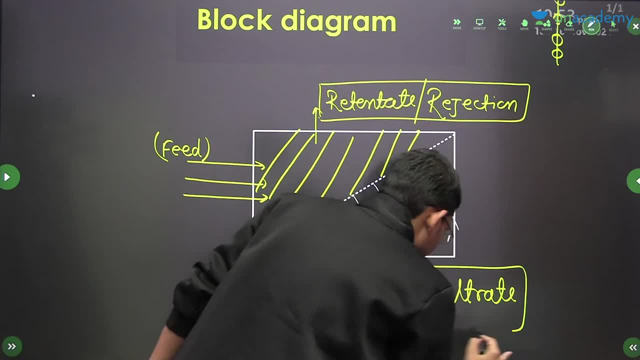 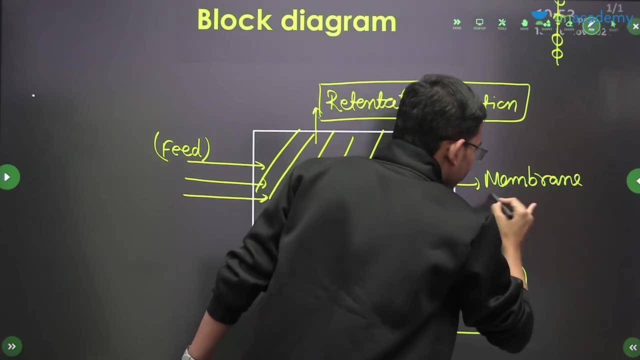 We will call this permeate. We will call this permeate. What is this? This is the membrane. This is the membrane. This is the membrane. Ok, this is the membrane. what is this membrane? ok, we will write all the terms. 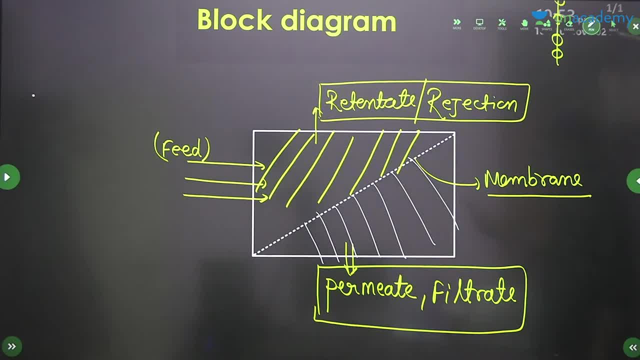 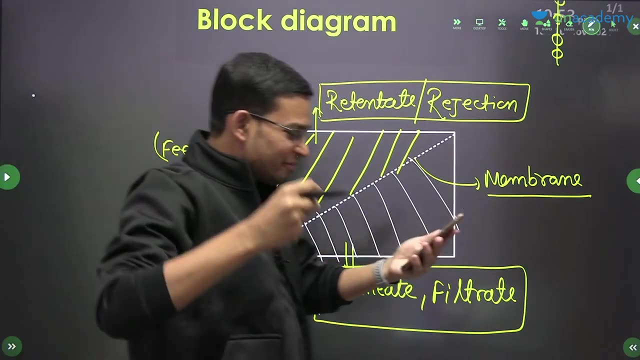 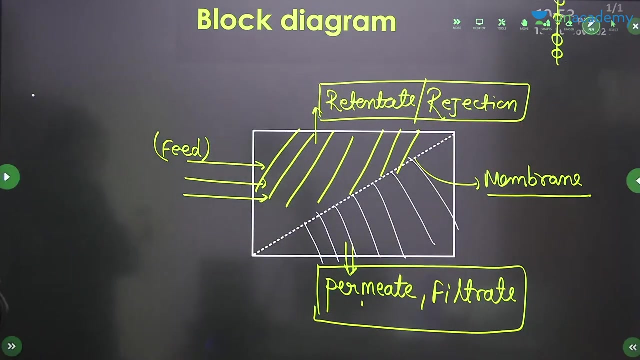 everyone cake upper. yes, you can ask the order of flex. you are right. you can ask the calculation of flex over size, under size. yes, you read this in mechanical operation: over size, under size. yes, you can say that under size. you can say that. very good, very good. 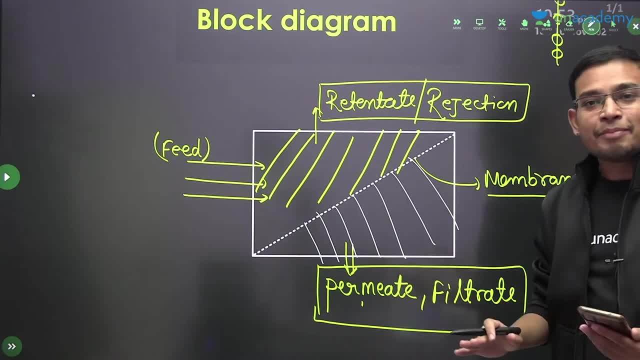 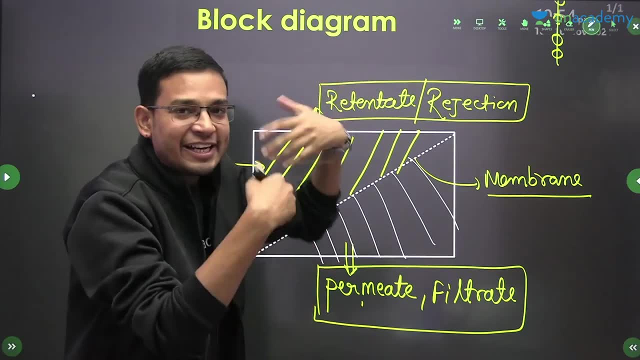 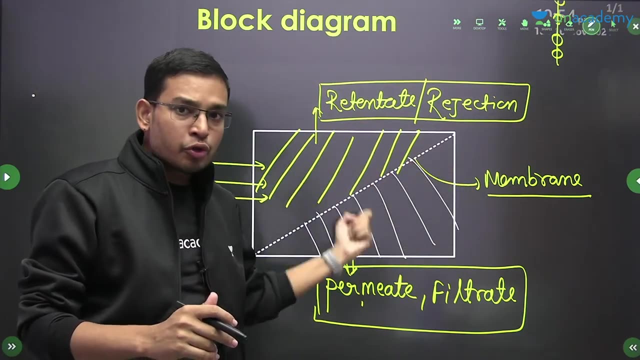 yes, very good, stopped, retentate, passed, permeate, absolutely correct, absolutely correct. so pay attention that what is stopped, that is retentate or rejection, ok, and what is passed is permeate. i will use this term in the coming time. these terms will be used very well. 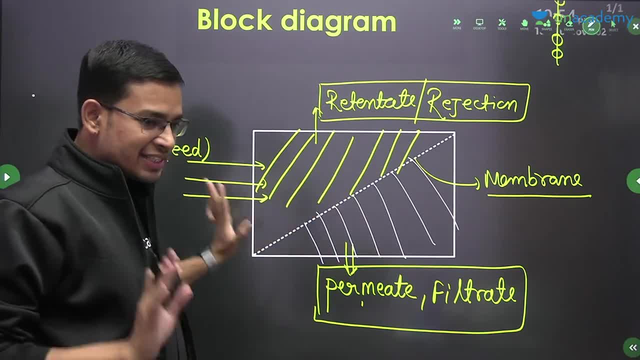 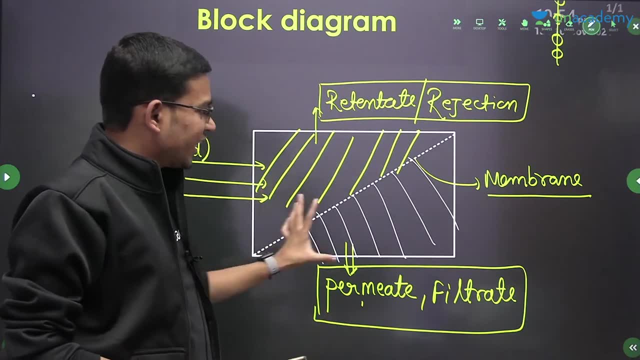 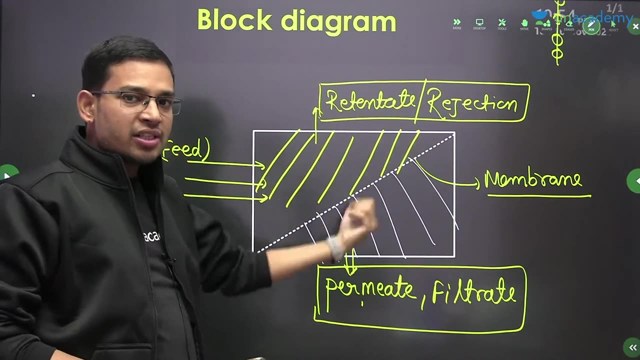 ok, next thing, we have this block diagram. make so many of them. this is your block diagram. this is the block diagram, because now, what i will take out from questions, i will take out from these. now, i will put all the material valance in this. i will put all the material valance in this. 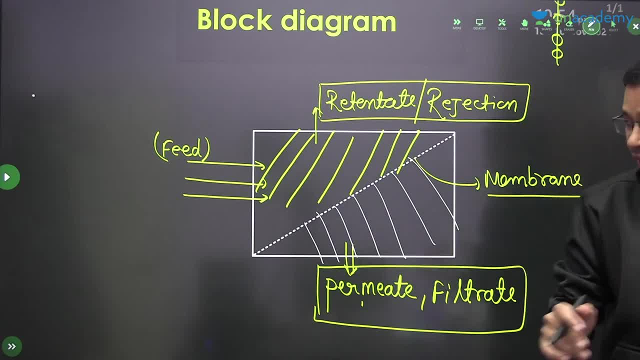 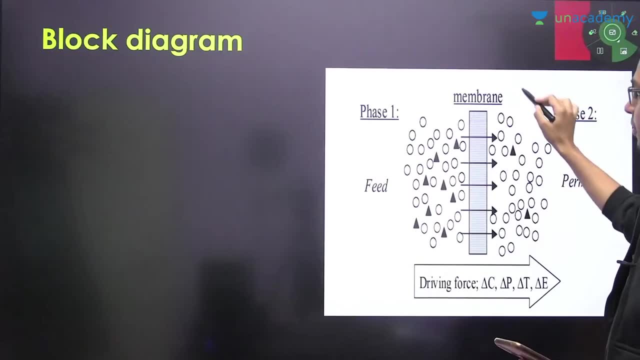 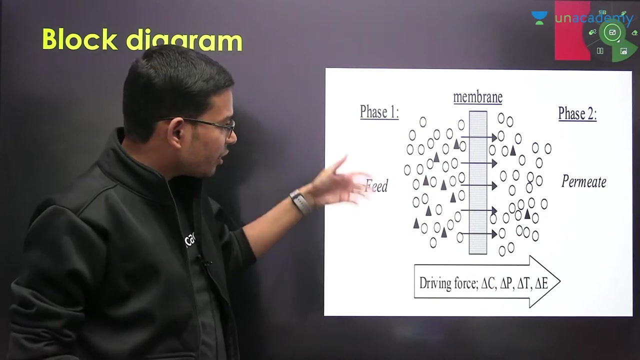 how will we tackle questions? we will take out using this block diagram. ok, now, all of them have done. come to the next point. this is done now. where is the dark stop? ok, is that? where is the dark stop? ok, we will take out. here you go. there is a dark. 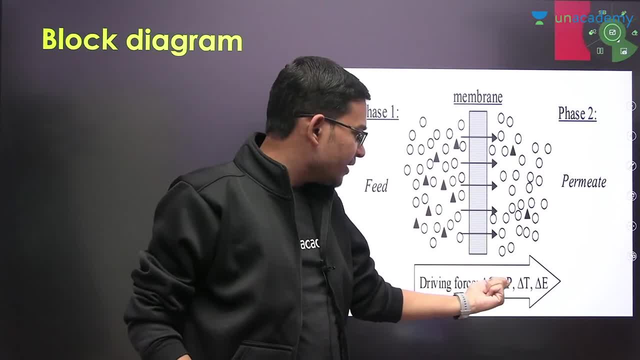 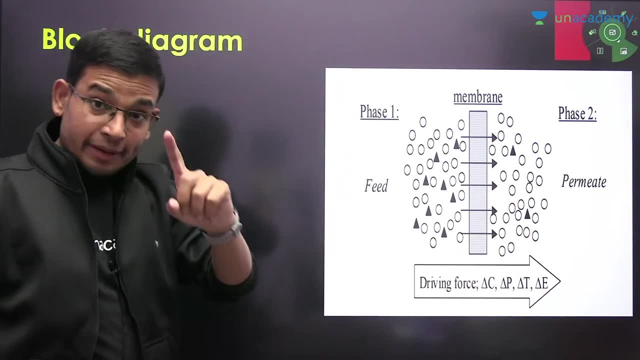 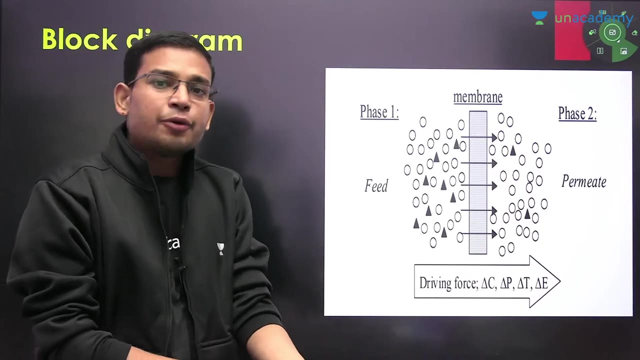 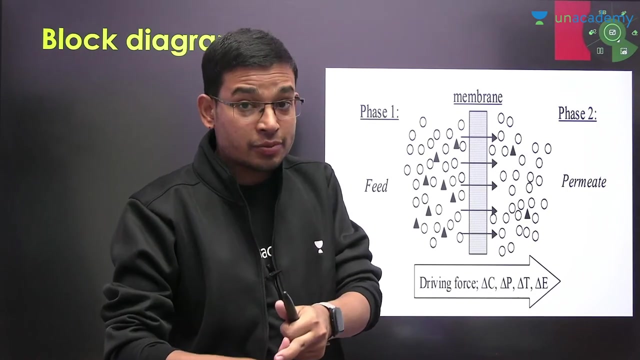 we will take out here, here, here, here, here here. ok, but it will not come here, but it happens. this temperature difference is also a driving force. but all the processes you have studied- ultra filtration, micro filtration, nano filtration, reverse osmosis- 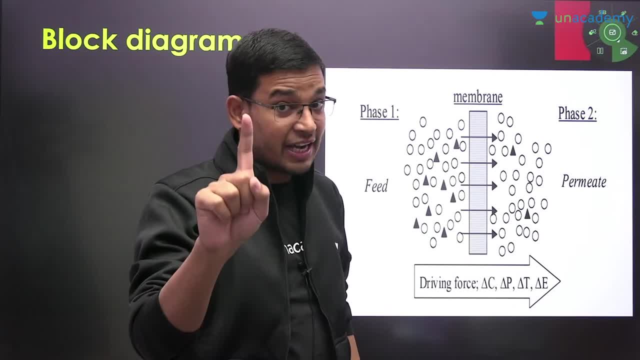 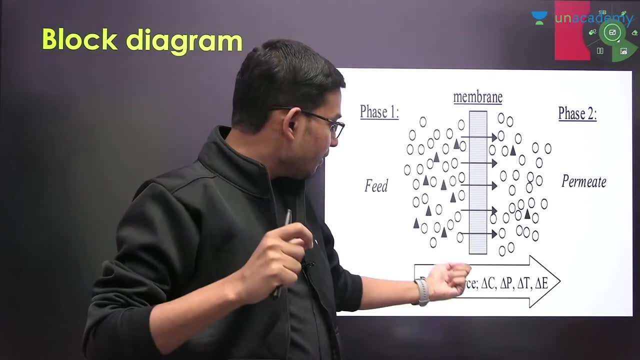 in this driving force is pressure difference. that can be asked in the question. this question can be asked to you. all the filtration you have studied. what was in all of them? your driving force is pressure difference, concentration difference. like your dialysis etc. you will get to see concentration there. 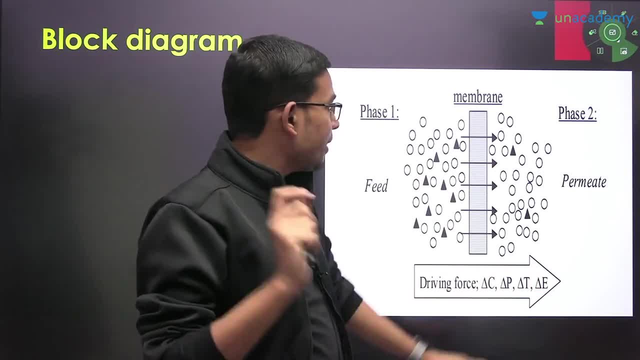 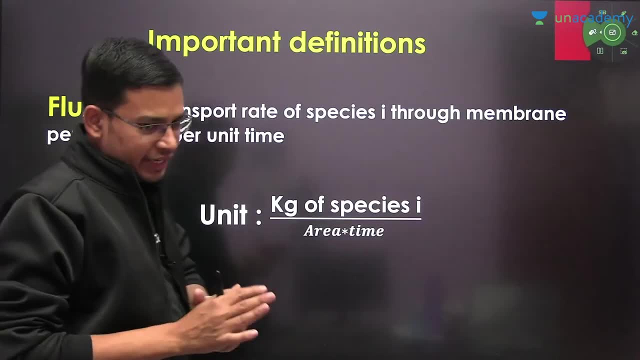 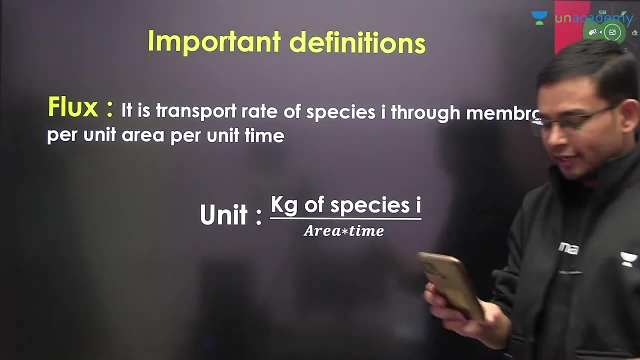 temperature difference electric fault like your electro filtration. you will get to see this there. come to the next point, some important definitions. now, from here, your story will start. write this definition: I will move from here tomorrow. what is the flux now? your real game will start from here. 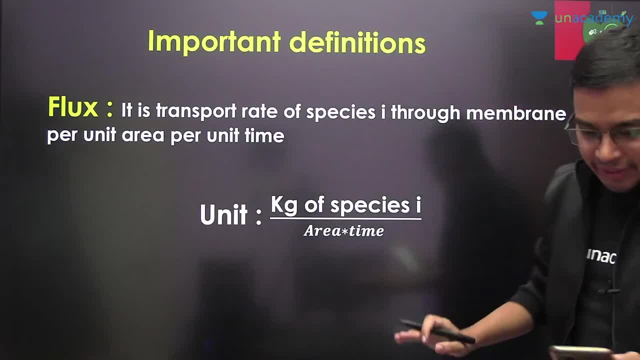 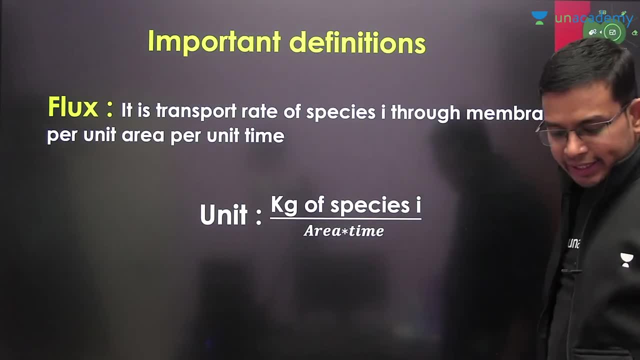 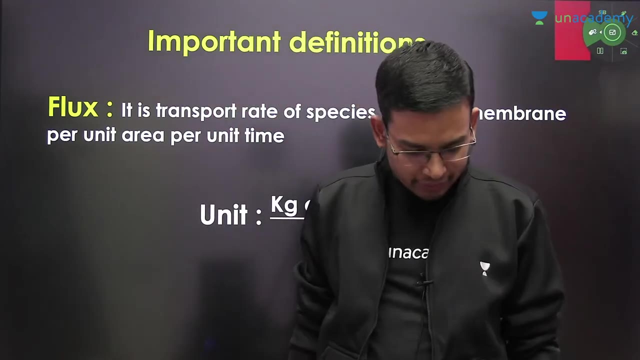 your real game will start from here tomorrow, so everyone will write. there will be many important definitions. I will continue this from tomorrow. today we will keep this much session because one session will be on 11.45, where I will get the practice of distillation today, right, today's session, I keep this much. 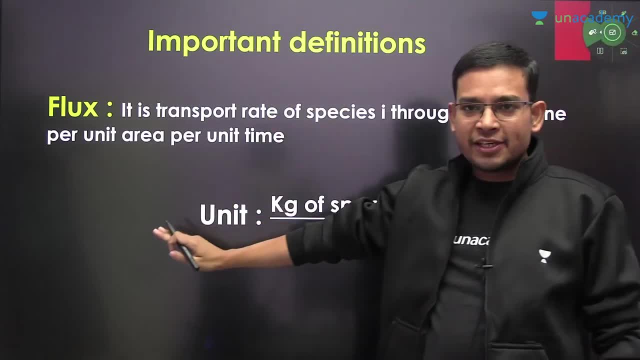 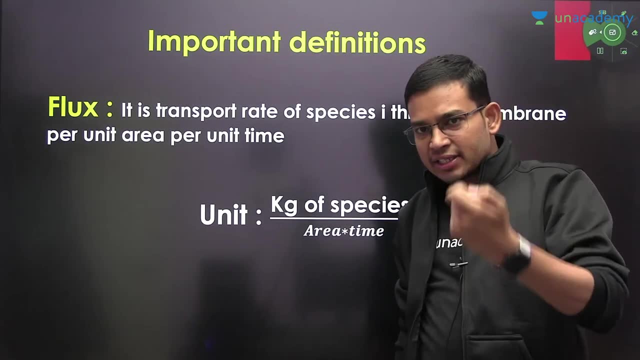 now, this is the first definition. now, small terms will start involving you. ok, one term will come, will understand those terms very well. numeric term. now, we will understand very quickly today、 all the part in theory is over. just this much, you are aware, to graph rhythm. this much is not enough. 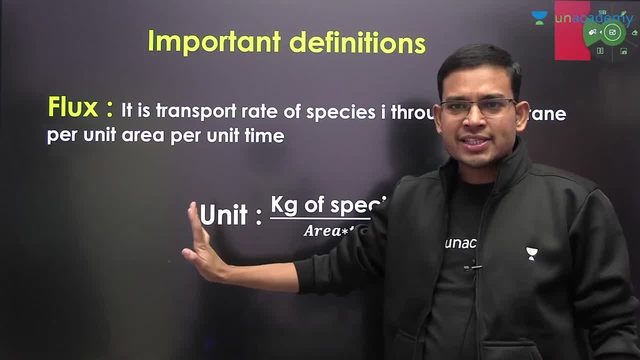 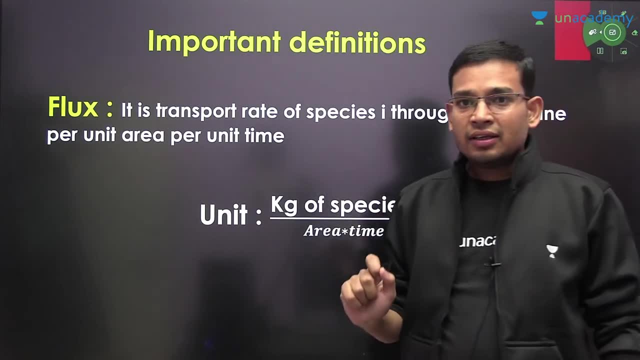 otherwise, If I had wanted this theory, then it had been studied for five days, which has no meaning. the number of theories we have studied today, these the mythologies I have studied for a, but it doesn't have any meaning. I know that gate doesn't have any meaning. 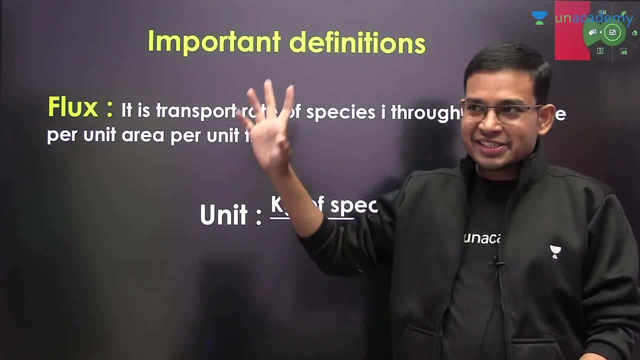 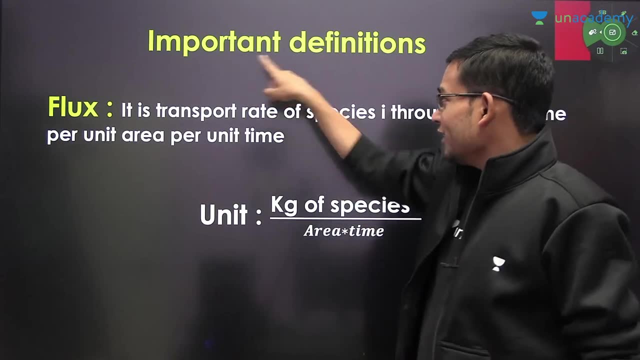 you guys are happy. I would have brought colored figures, sir, this molecule of red color. it would have been fun, but the question of gate doesn't come out. the question of gate will come out from yesterday's lecture, so we will add heading flux, the flux that we will calculate here. 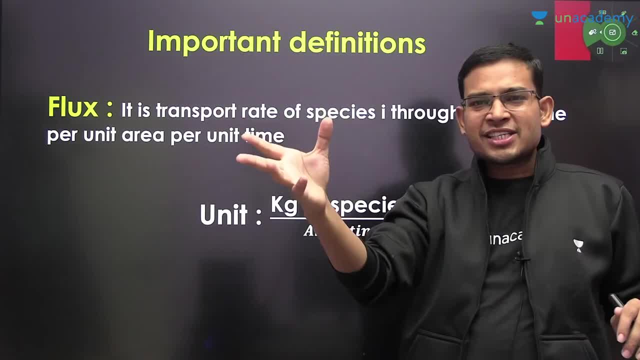 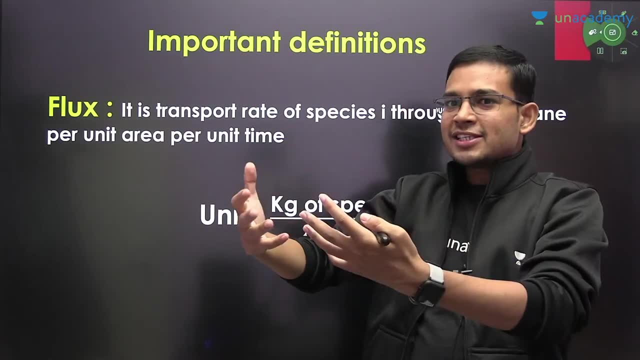 in membrane separation. how will we do that? amount of the species i flux is our universal law. amount of the species i per unit area per unit time. amount of the species i passes per unit area per unit time. that's called flux in the membrane separation. so everyone will write. 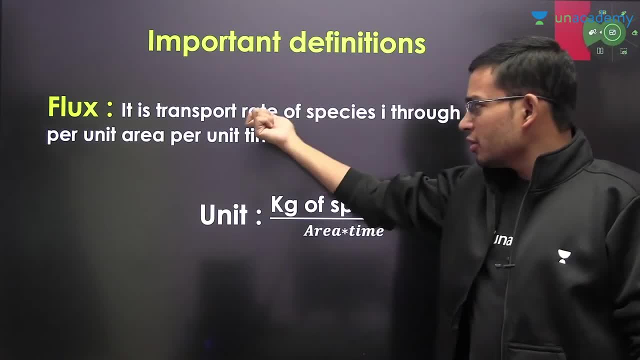 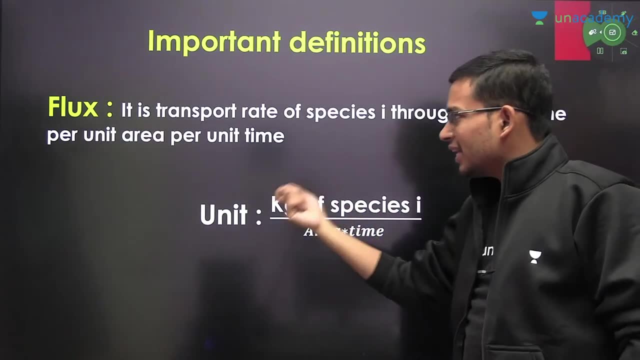 amount of the species or transport of the species. amount can also be, transport, rate also can be. this can be rate. your amount can also be so: kg of the species. i per unit area, per unit time. that's the flux. this will be the unit. so what will be the unit of this? 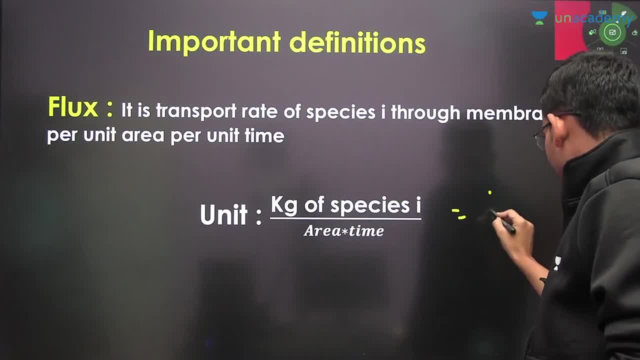 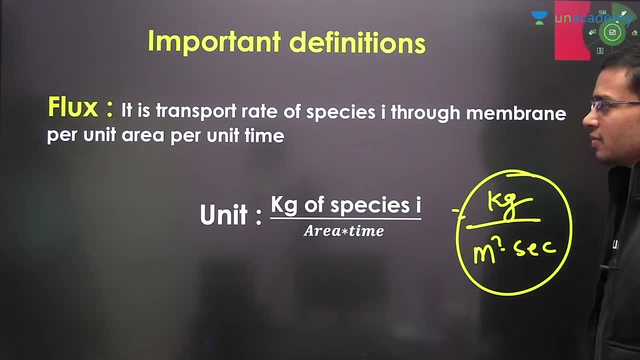 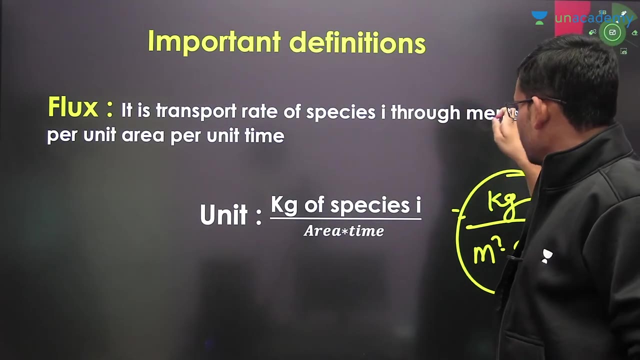 everyone will write it here. unit is kg. unit can be kg upon meter square per second. this unit is possible, this unit we will write. So how is flux defined here? It is the transport rate of the species i through membrane per unit area, per unit time. 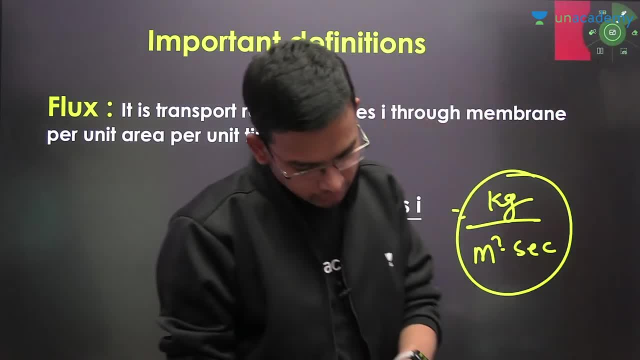 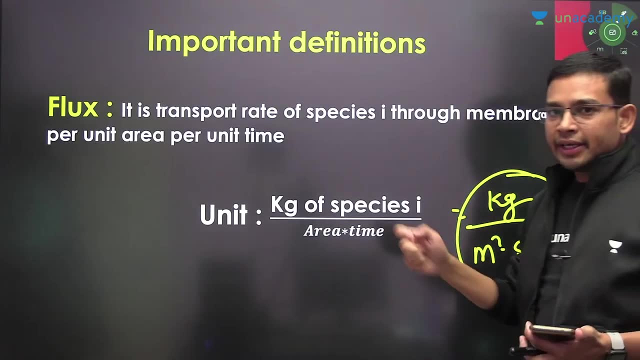 So many people will write the definition of this in an amazing way. Yes, kilogram per meter square per second. Now you will see small terms will start from here. What is flux? What is permeance? What is permeability? What is permeability constant? 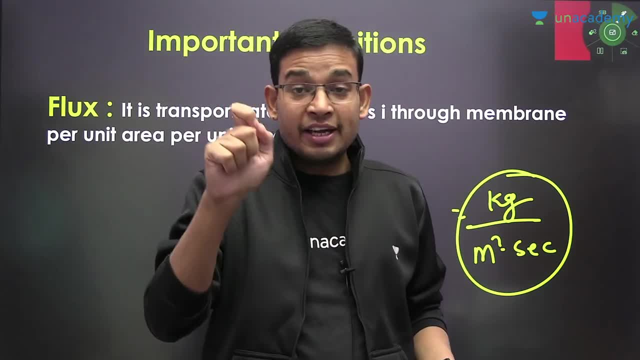 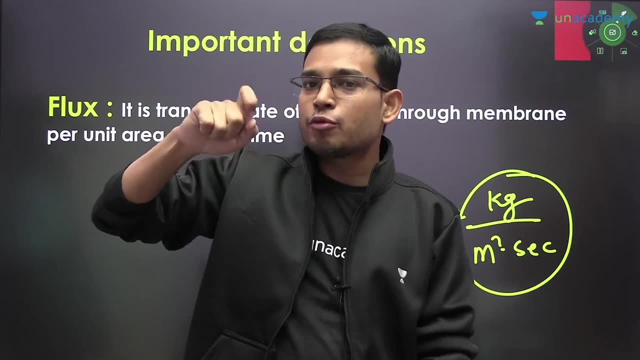 These are small terms like: what is diffusivity? What is mass transfer coefficient? What is permeability? What is permeance? What is permeability constant? You will know all these terms and only then you will be able to tackle the question. 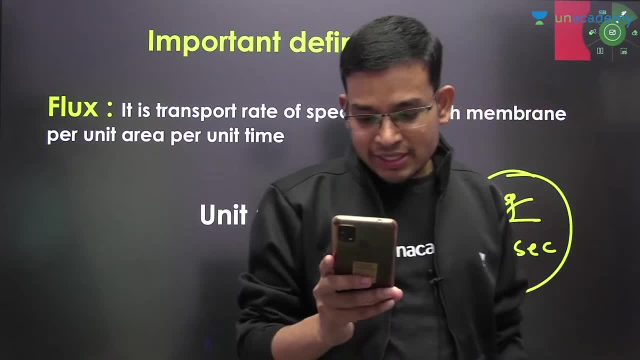 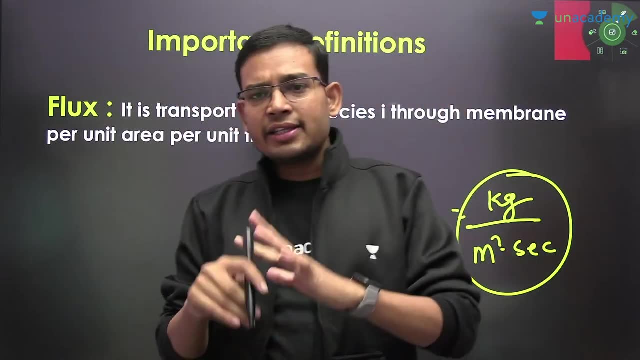 So we will talk about this tomorrow. Sir, thank you so much. I watched your all IPC lecture. Yes, thank you so much. Hope you all enjoyed today's lecture. Now understand one thing: You do not need to study more than this in the theory part. 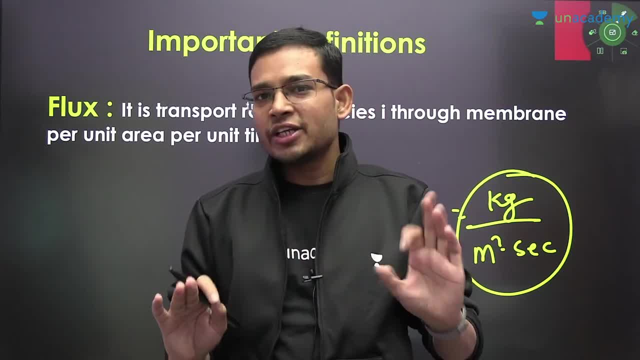 I am telling you that in the GATE exam you will not be asked questions of theory. I am telling you that in the GATE exam you will not be asked questions of theory. This is my personal experience. You can understand anything. 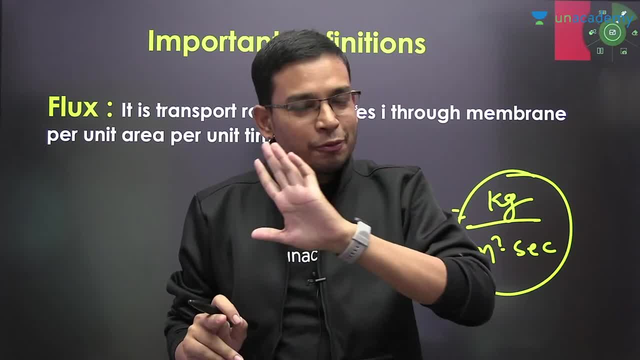 I am telling you, I am telling you this in my experience: You will not be asked questions of theory in the GATE exam. No matter how much I teach you theory, you will get numerical. So how to study is numerical tackle. 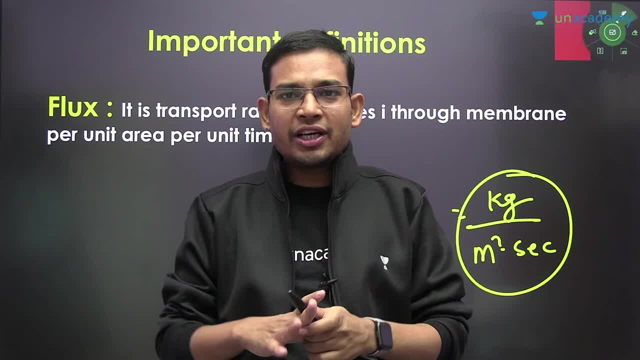 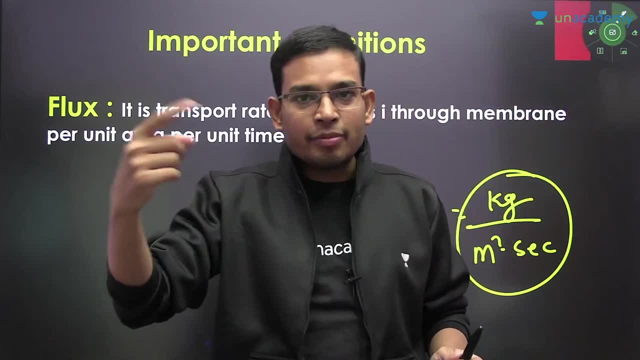 Always keep this in mind. You will get numerical. You will get theoretical. Whatever I have told you, theory can be possible from this part. That's it. You will not get anything else. Now we will talk from here about how you will get numerical. 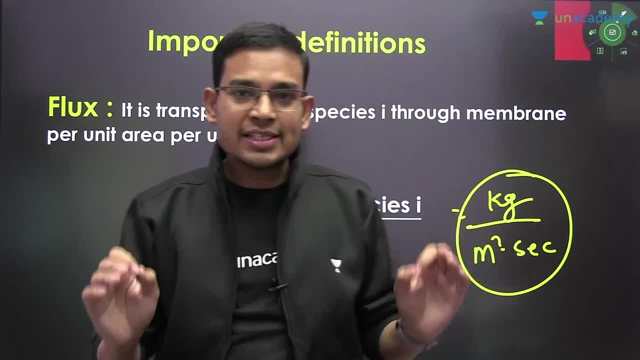 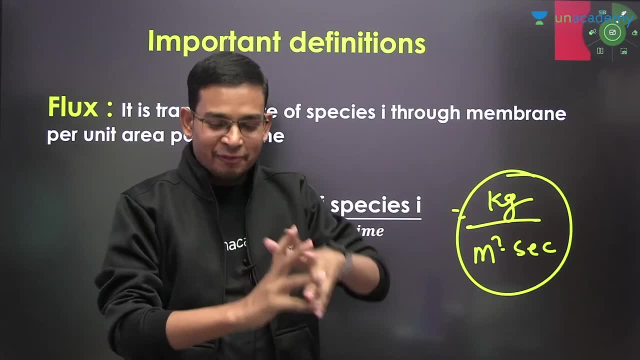 We will talk about that tomorrow. Yes, hope you all enjoyed today's session. Today was the first over. You will get to see all the overs in the coming time. Now we have just flicked. Okay, It's well leaving very soon. Sir, how many days will the membrane separation last? It will last, It will end. Okay, I cannot decide now How much is it Right, But yes, it will last at least 3 to 4 days. It will last at least 3 to 4 days. 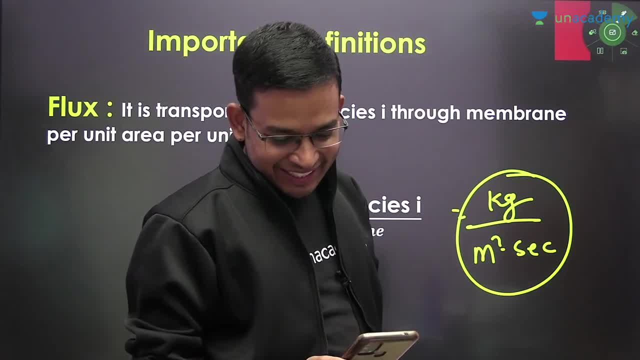 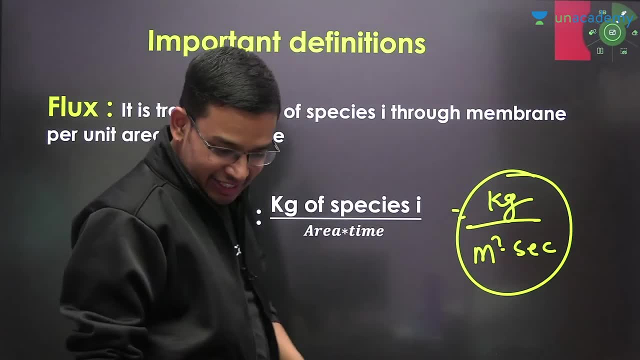 Okay, Yes, It was fun, sir. I hope you all enjoyed. Okay, It was a small session. It was small, It was tough. You all have supported. well, Yes, 70 children are watching. I was not feeling that 70 children will also come in the session. 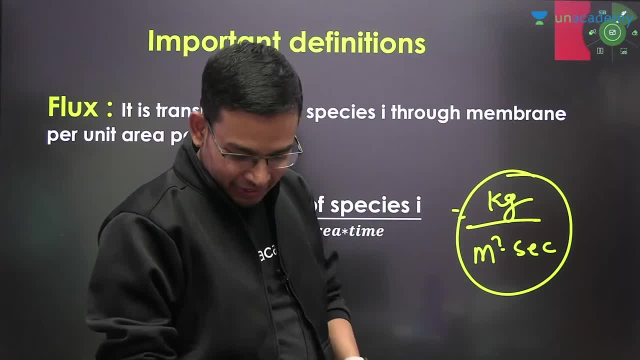 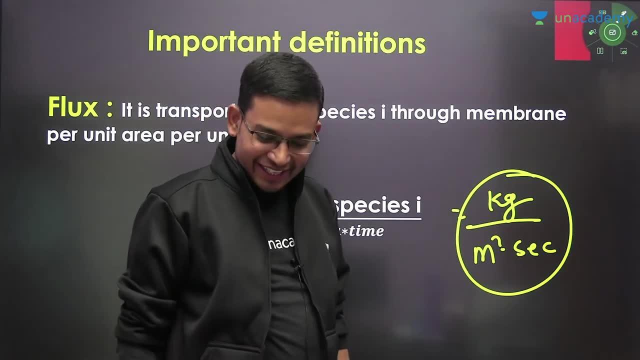 So then understand, I will get membrane separation done at your next level, Okay, In case so many children are present. Yes, sir, So then I, Yes, Yes, Yes, It is important to stay steady, Yes, 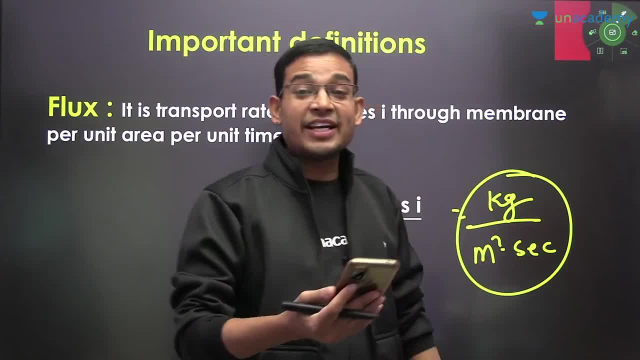 Absolutely correct. It is important to stay steady, Guru. Okay, I did not know that 70 children will also come, Because in the session, 20 to 25 children are coming. these days, Sir, your mass transfer and IPC are coming. 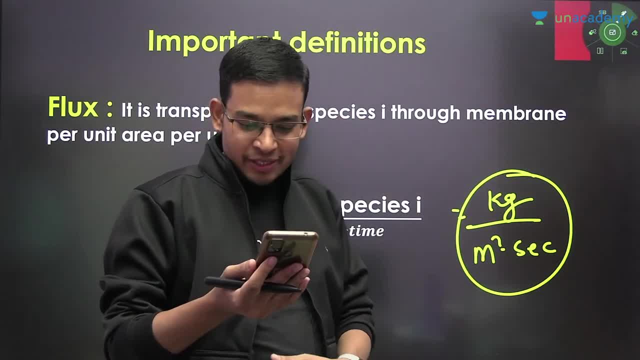 Yes, Thank you so much. Thank you so much, Vaishali. Thank you so much, Sadanand Mandar. Thank you so much. Come on, brother, I will just talk from here. I will teach permeability tomorrow. 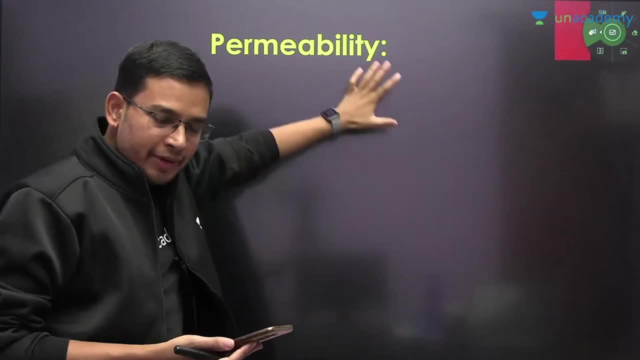 Okay, I will teach permeability tomorrow. Right, Come on, I will just talk from here about the offer. So, brother, This offer is going on right now. Sir, everyone will come in the next session. Yes, There is no problem. 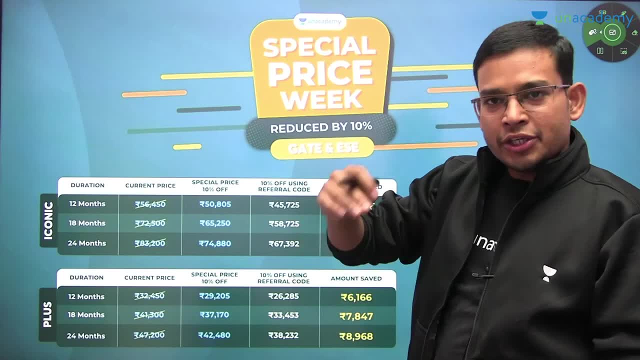 All of them will come, They will enjoy and go. I guarantee only this much. Come on, I will just talk from here. Guru See, Special price is also being offered at some time. So those who are also interested, For whom? 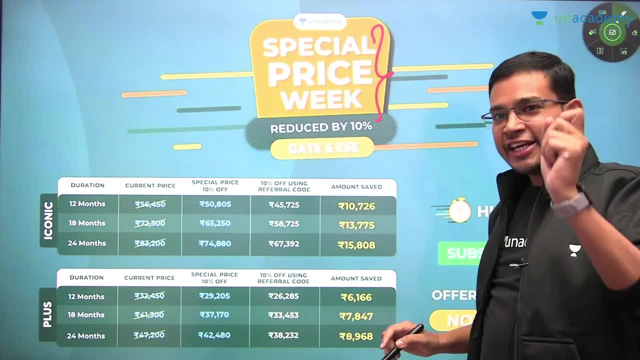 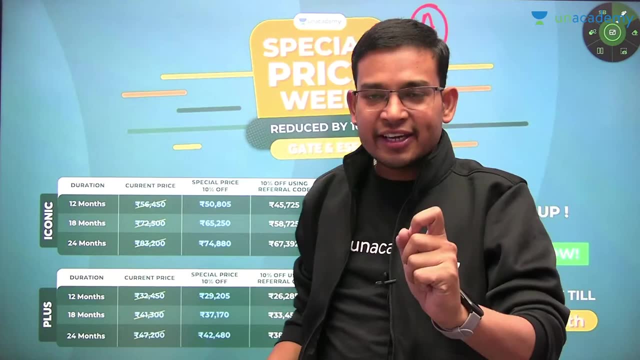 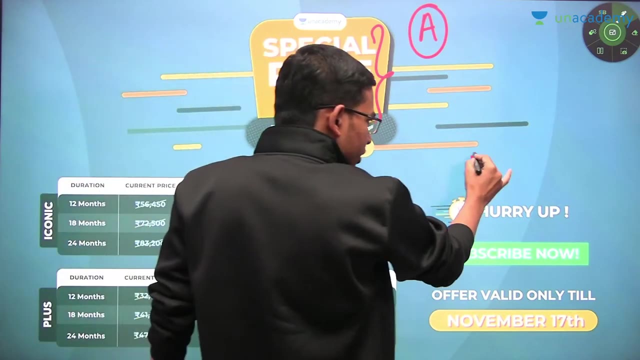 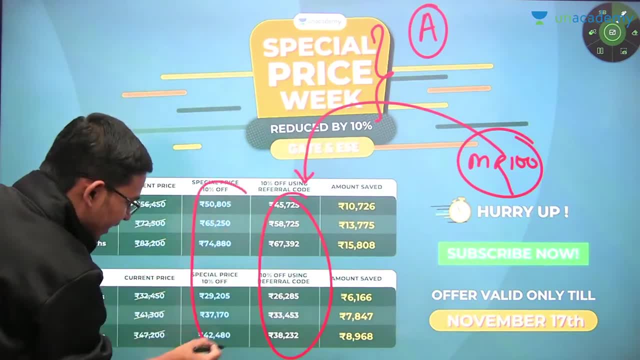 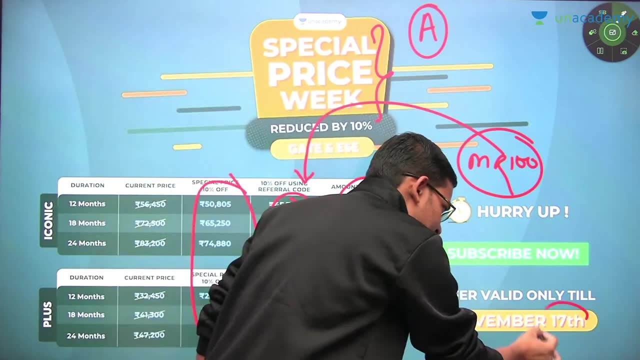 Oh see then, Sir, From here there will be a source to start for free. I will give you one thousand rupees. Okay, At that time. I am sorry for your loss, sir. We will have to delay it, Sir. 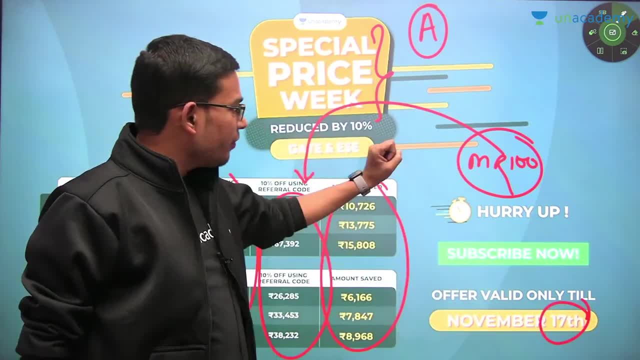 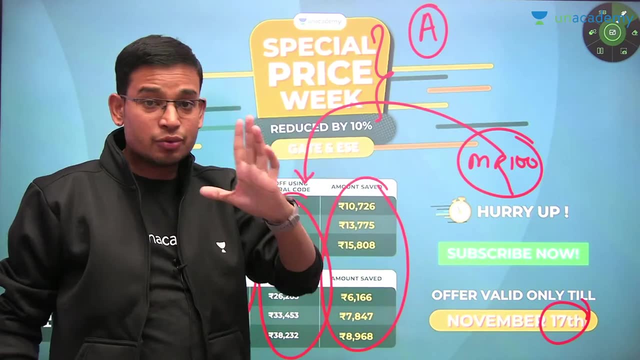 Stop talking. by tomorrow this offer will be over, so whoever wants to move can do it now. the first batch has started for batch A23, so you will use the code MR100. from here, you will get a 10% discount. see, this is the fee structure. 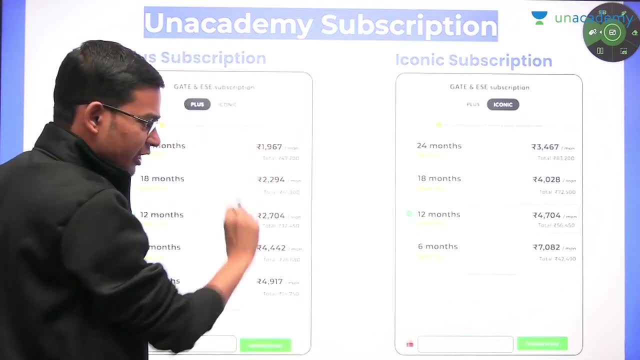 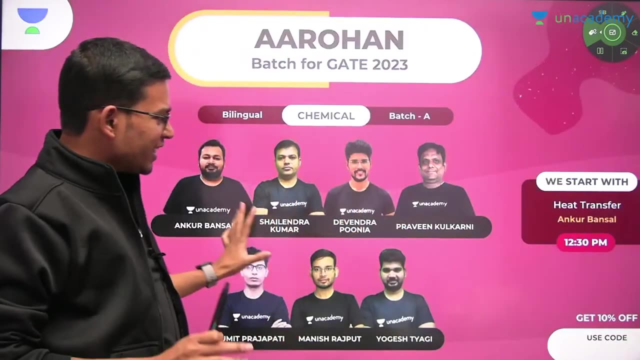 those who want to move with plus. this is the fee structure on the basis of EMI, so you can see those who will not be able to pay at the same time. they can go on the basis of EMI. there is no problem. this batch A has started. 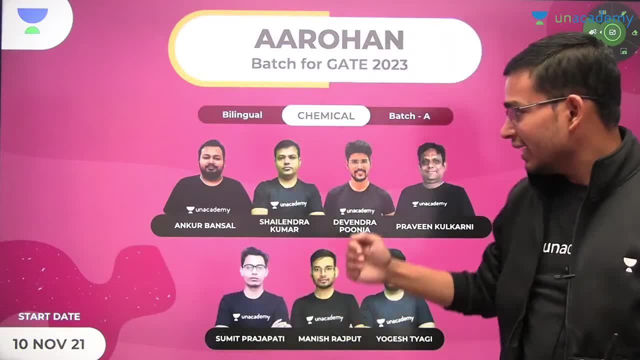 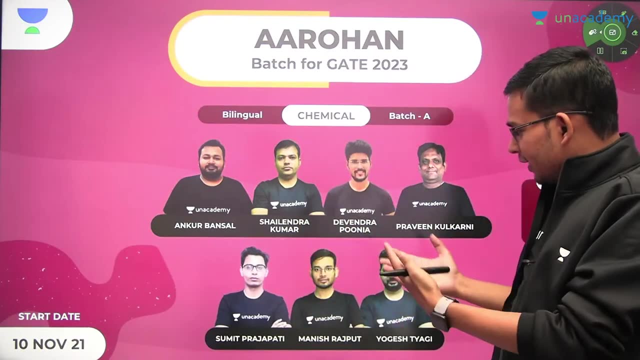 in which your heat transfer has started. you can continue with the heat transfer. this is our team of chemical engineering. one subject is different from us, not like this. study from Ankur sir. study from Deven sir. ok, one subject you will get a chance to study from 2-3 people. 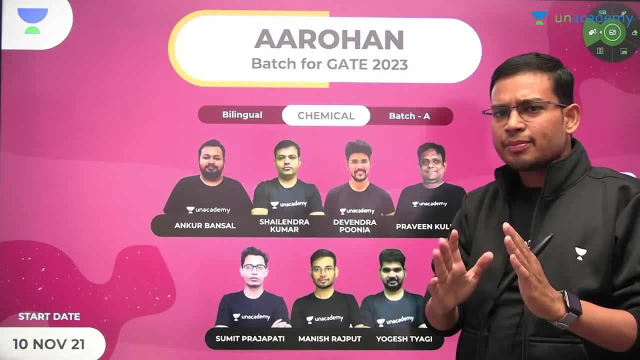 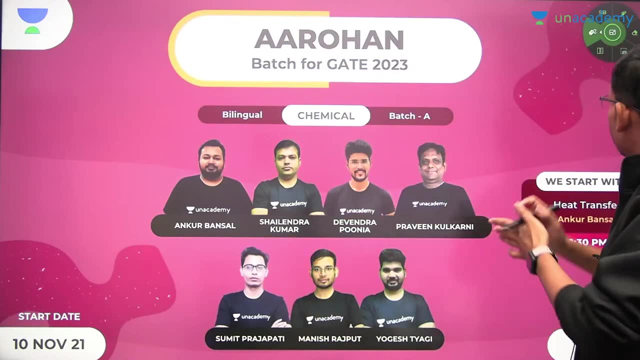 ok, IPC is done. there is no such subject. study from the same faculty you can study from 2-3 people means you will have fun in a nice way with the whole team of chemical engineering. so whenever you join, then join. you just have to use the code here. 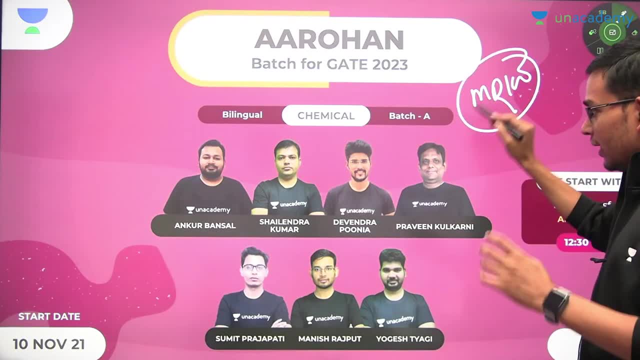 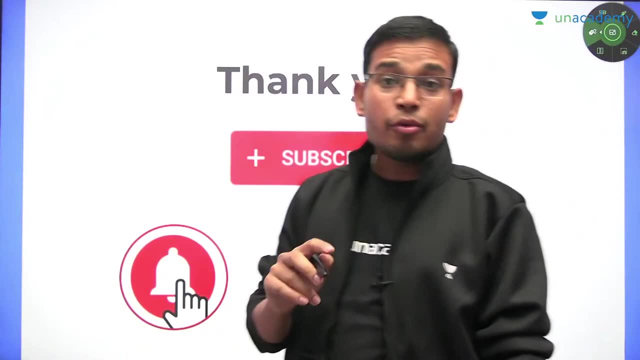 MR100. this is the personally my code. this is my code, so you can move with this code and follow our team. ok, I will talk from here. ok, thank you so much. thank you so much. tomorrow morning you will have first order system and now, from 11.45, 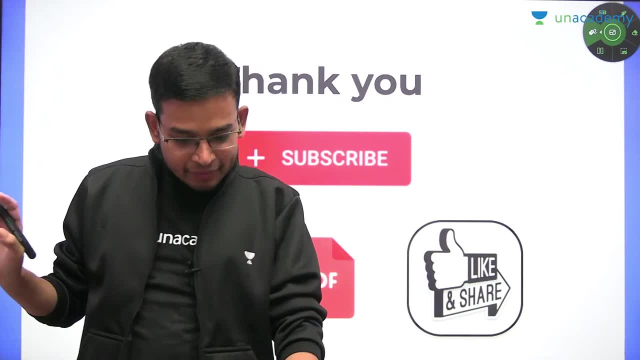 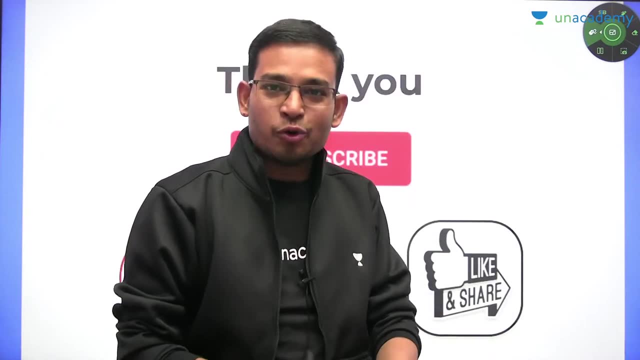 you will have one more class. ok, 45 minutes break for you. ok, 45 minutes break for you. I will also have dinner. ok, because of this I have left a little early, otherwise 2 will be saved. ok, yes, Salen, sir said to ask you once. 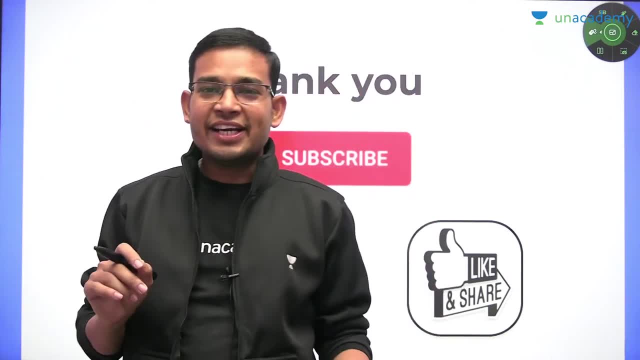 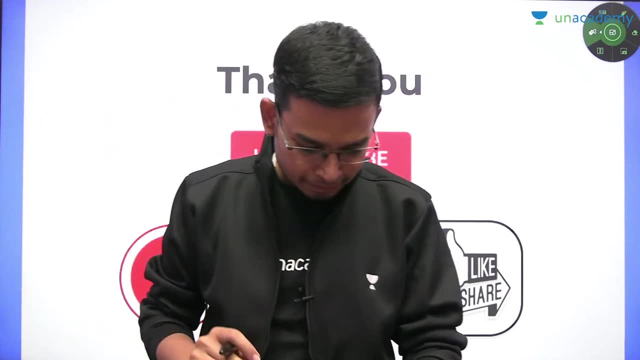 for solution thermodynamics. yes, you guys, if you are present, then solution thermodynamics. after finishing all these newly added topics, I will start solution thermodynamics on YouTube. ok, don't worry at all. ok, Sadanand, I will start on YouTube. yes, Vaishali, I will do solution thermo.